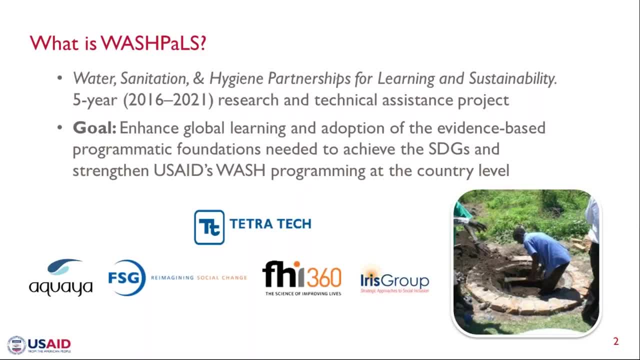 Service, as well as Subhas Januri, the Associate Director for FSG, both who have worked extensively on this report and presentation. During the presentation and the webinar, all participants will be on mute, but you can submit your questions through the question box on your control panel. So if you just 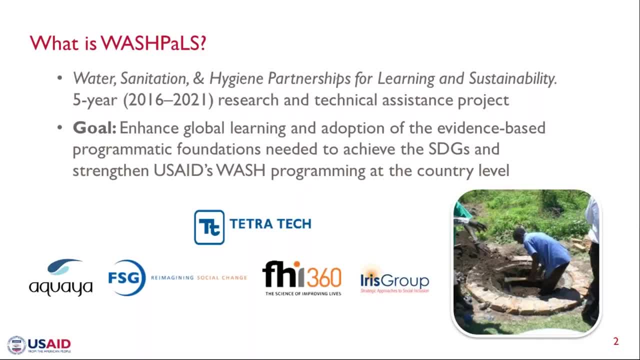 open that up, you'll see an opportunity to provide questions there. You can submit those questions at any time during the webinar. We will be collecting them and also sharing them with the entire audience and participants as we go And then during the question-and-answer. 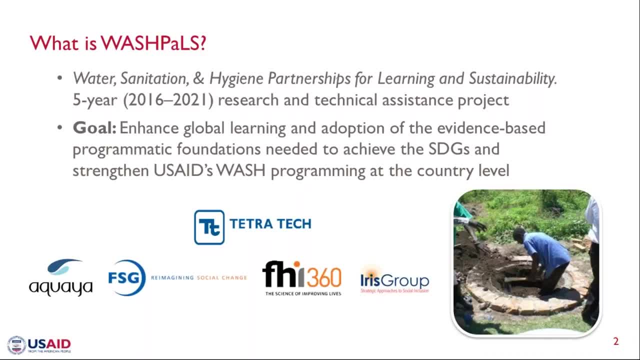 period, we'll have a facilitated discussion that'll go through many of those questions. This webinar will also be recorded and posted after, if you would like to rewatch it or share it with your colleagues or share it with others. So let's get started. 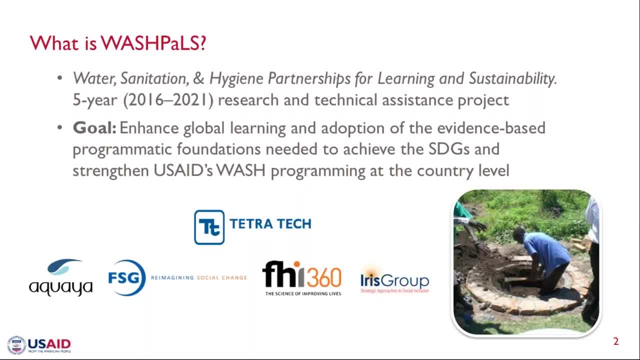 Just before we jump into the content, I wanted to share with you that this Global Desk Review that we completed was conducted through a USAID project called WASHPALS: WASH Partnership and Learning for Sustainability. This is a five-year project from the Global Health Bureau. 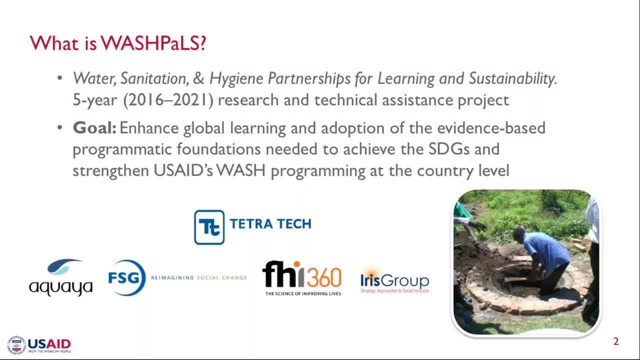 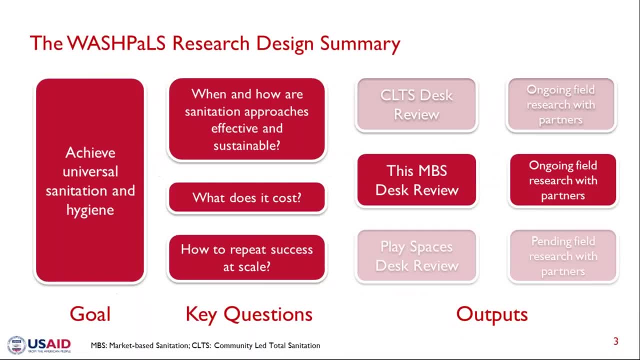 that includes a number of partners. It's led by Tetra Tech but includes Aquia, FSG, FHI360, and Irish Group. You'll be mainly hearing from the FSG today. Our entire WASHPALS project is really focused on learning and research and we've really 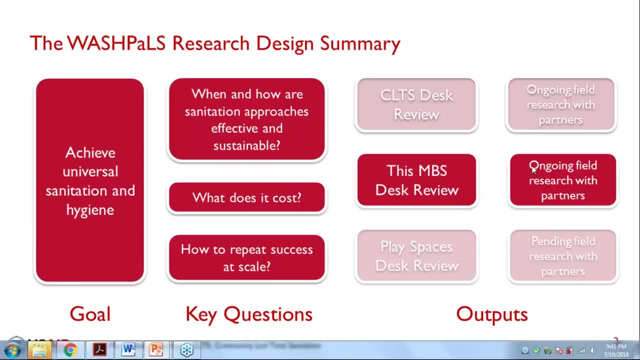 focused in on the sanitation and hygiene sector, particularly looking at how can, together, can we achieve universal sanitation and hygiene, And we've focused in our trying to define the areas by which we want to explore by defining three primary large areas, One of which is when and how our sanitation and hygiene approach is effective and sustainable. 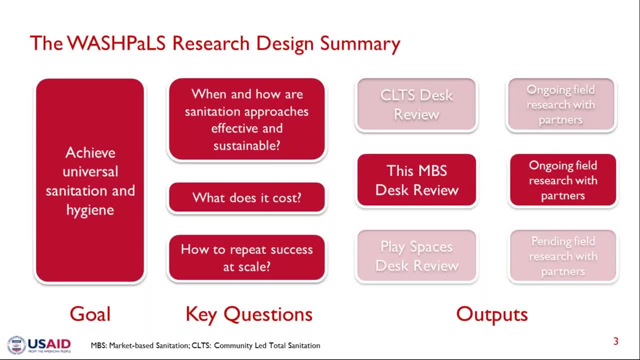 what do they cost and how can we repeat them at scale? So those questions have helped us define three primary areas where we're doing research focused in on CLTS, market-based sanitation and clean play spaces for infants and young children. Today, you'll be hearing primarily about the market-based sanitation component. 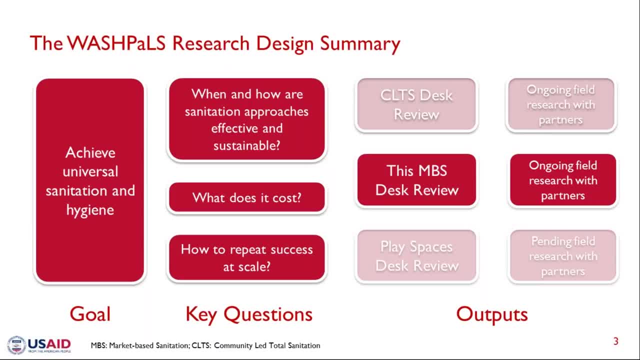 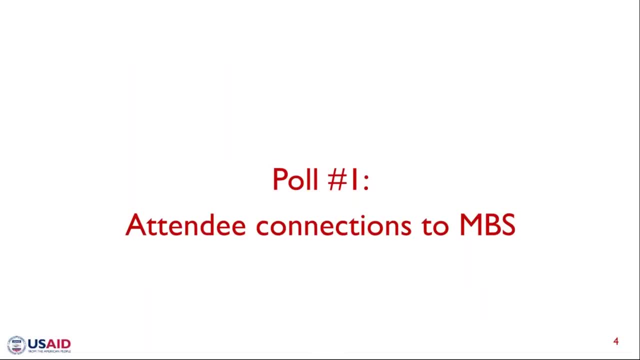 We're going to be looking at how we can make the most of the benefits of the market-based sanitation. So we're going to be looking at the benefits of the market-based sanitation component of our research, primarily this initial desk review. So with that I would like to transfer you over to our first poll. 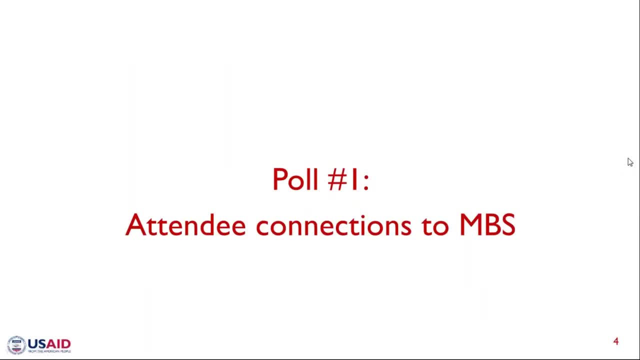 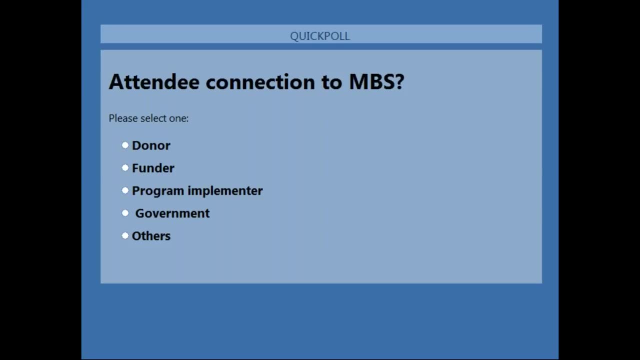 So, attendee, we want to learn a little bit about your connections to market-based sanitation. So, if we can start the poll here, If you can just vote on this poll, And while you're doing that, I will hand over the poll to the next person. 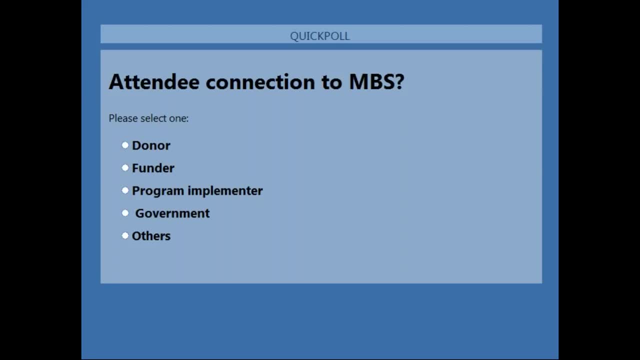 And then I'll hand over to you and then we'll move on to the next question, And then I'll hand over to you and then we'll move on to the next question. So the first question is: And then I will hand over to you, and then I'll hand over to you and then we'll move. 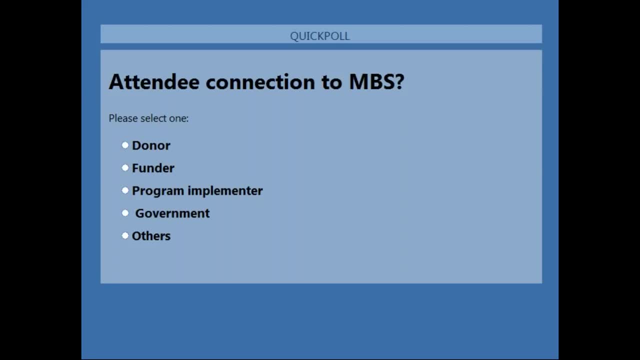 on to the next question And then we'll move on to the next question. So if you can just please step forward to answer this question, Okay, So I will hand over to you and then I'll pass it to you, Okay. 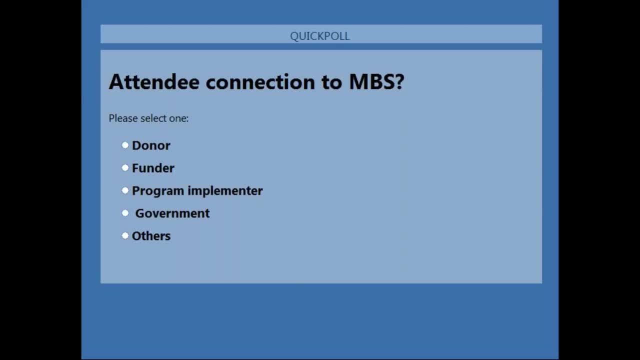 Thank you, Jesse. Thank you, Jesse. Thank you, Jesse, for the setup and introduction to the WASH BALS program. I'd also like to extend a big thank you to the numerous individuals and institutions who partnered with us in this analysis by way of sharing insights and our data for the analysis. 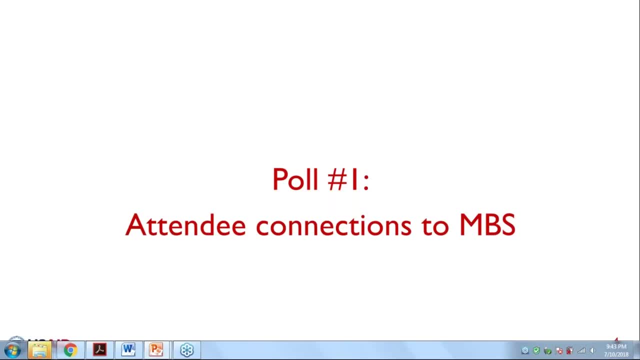 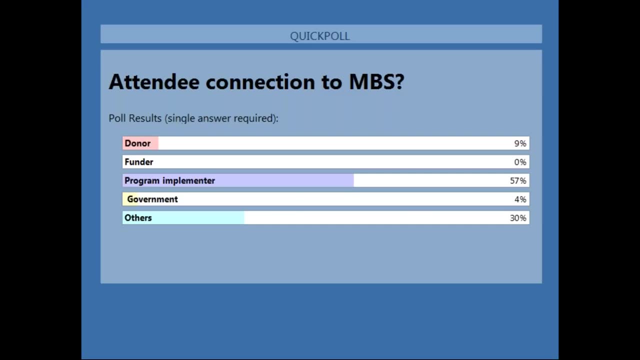 At this time. I'll just close the poll to see what you think. Okay, to see what the findings are, and let's just share them. so, as you can see, we have a split: largely program implementers, some others and few donors. that's great, gives me a sense of the audience. so 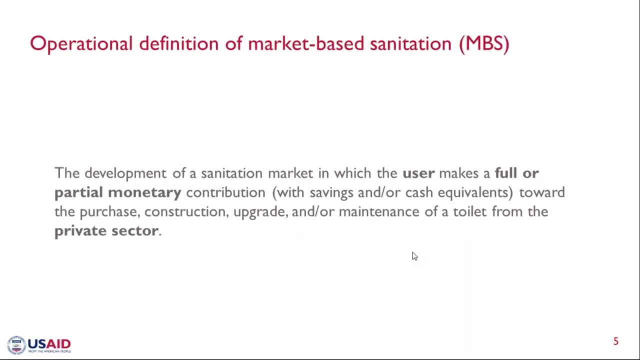 let's move on to the presentation itself. so before we start, we get into the findings. at the outset I wanted to lay out the definition of market based that we have used in our study. as you can see on the slide, there are two key criteria that we use. first is that the user has to make at least. 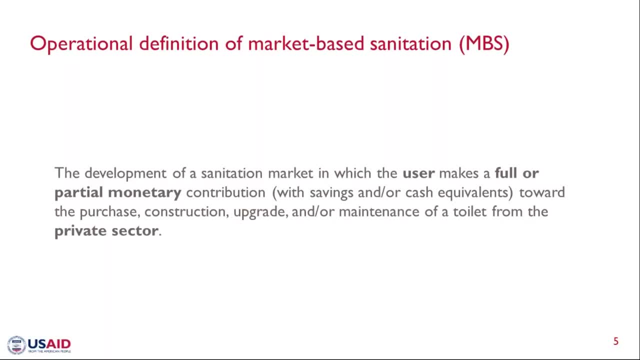 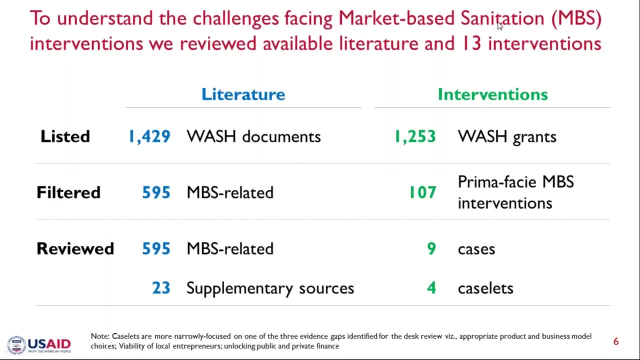 partial monetary contribution and second, that the product and service delivery has to happen through the private sector. so, using this definition at wash pals, over the last year or so we reviewed over 600 articles and studied 13 interventions across the Google's out to arrive at the fame of the scaling market. 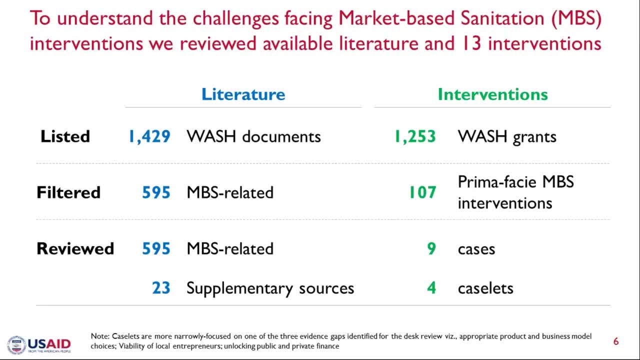 based sanitation. the literature was reviewed with the focus on freaky evidence, gap areas of business models, sanitation entrepreneurs. and unlocking public and private finance for market based sanitation. this involved the systematic review across the business models, sanitation entrepreneurs. and unlocking public and private finance for market based sanitation. this involved the systematic review across the 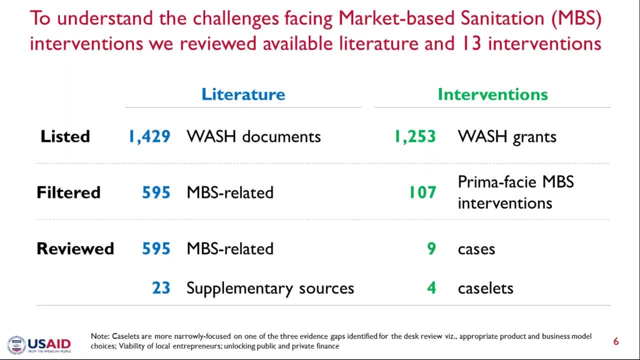 seven sector-specific resources using 16 search screens. For further details on the sources, the search screens, the methodology, please refer to annexure 1 in the report. Since a large proportion of the results we got on these searches were grey literature, these findings were augmented by a desk review of 13. 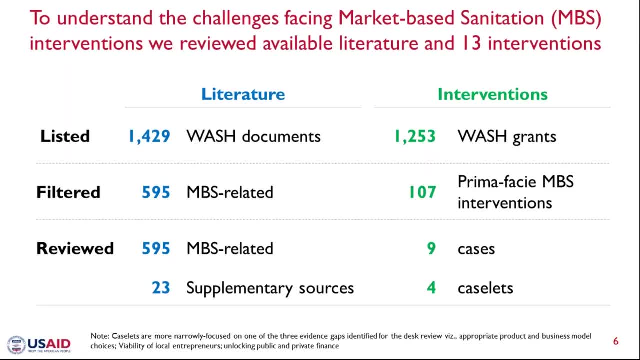 interventions, of which 9 were studied in detail and 4 called caselets in the report and on the slides, were studied for specific crops. These were around any of those three evidence gap areas that I spoke about earlier. So what did we find? 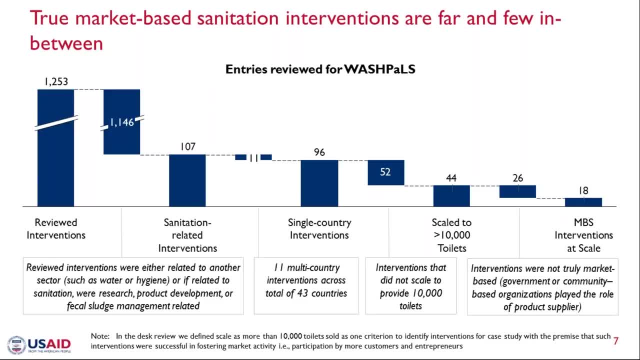 At the outset, let me say that scaling market-based sanitation is hard work. Finding them was hard enough. In our analysis, we were able to identify only 18 single-country truly market-based interventions That scaled to at least 10,000 toilets. 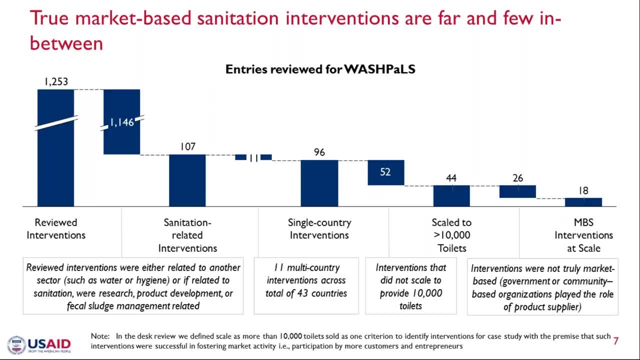 Which, if you think of the problem at hand in itself, is a fairly low bar for scale. That said, five of the interventions we studied did manage to scale to over 100,000 toilets. We think that studying these interventions has revealed some. 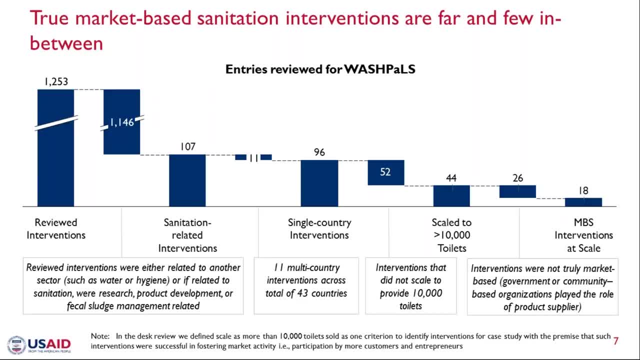 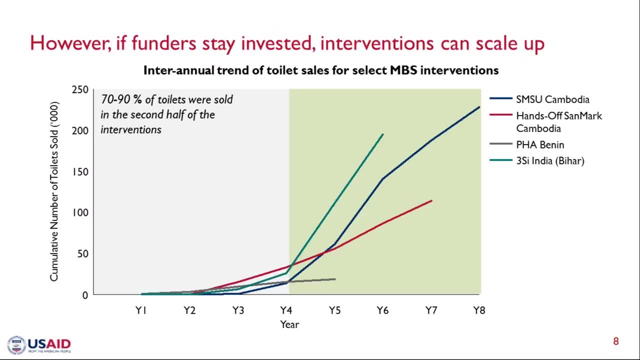 common strands which can be leveraged by other intervenors to scale market-based sanitation. So not only is scaling market-based sanitation hard work, it takes time. As you can see on the schematic, most programs took two to three years to get their business model right and were only able to start. 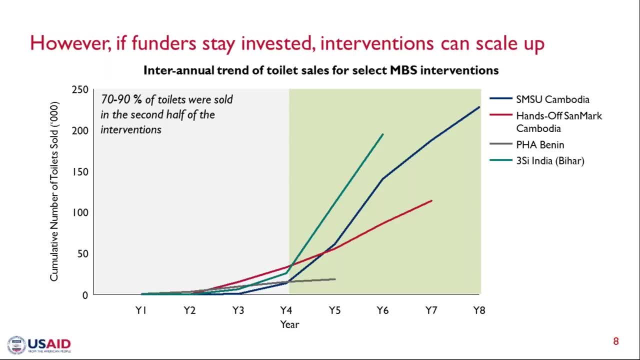 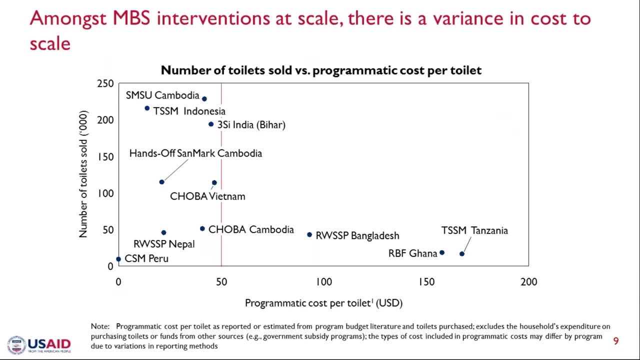 scaling post that period. There is a bit of hawkishness here. that reaffirms the need for funders and implementers to stay invested beyond the normal project horizons, which only are three to five years, if they truly want to scale and support markets to go to scale. We also tried to create an understanding of the 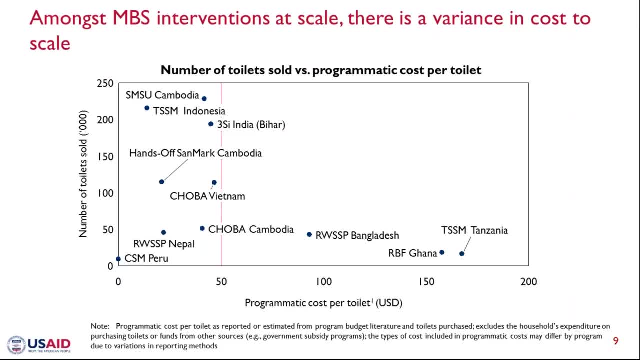 programming dollars that went into creating the scale. And when I say programming dollars, as you would see in the notes, it's just about the cost that was put by in the programming and the implementer, by the funder, and not the actual cost of the toilet which was paid by the. 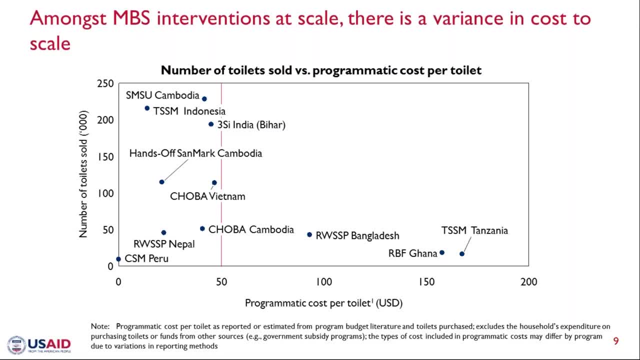 household. As you will see on the slide, the cost varied significantly, primarily due to the scale achieved by the program. In general, however, what we saw was the programs which were able to scale did so at the programmatic cost of twenty to. 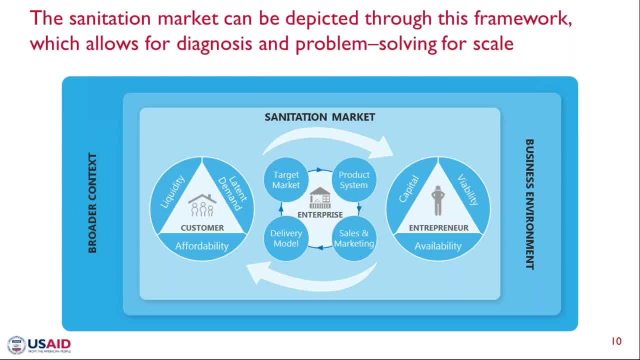 fifty dollars per toilet. So we looked at six hundred articles and thirteen interventions, but what did we learn? What you see on the slide is our synthesis of the findings. This is the way we, conceptually, are framing how the sanitation markets work and are going to walk through these layers and 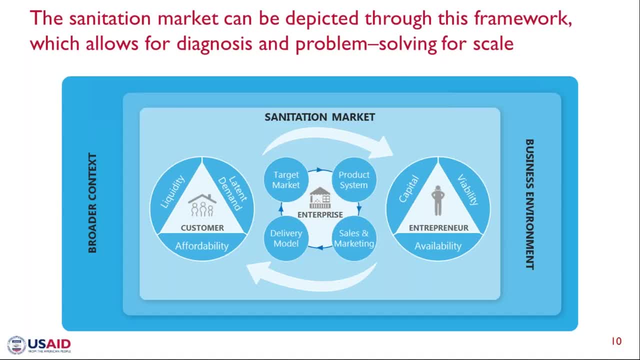 elements in the next twenty or so minutes. At the core of the framework is the sanitation market, the middle layer that you see, which comprises of customers, entrepreneurs and the interaction between them characterized by sanitation enterprise. This is the layer of the framework an implementer has the potential to create. 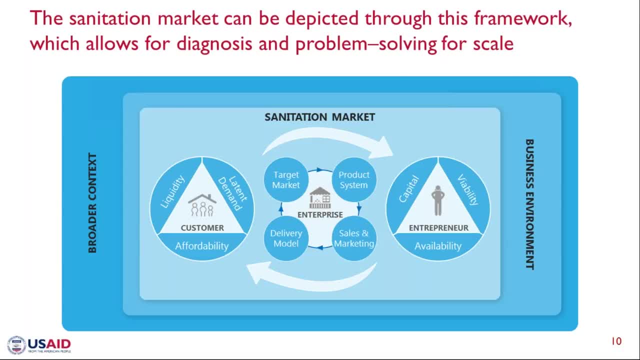 significant impact through an intervention. These are the elements they would have most control over. At this level, the sanitation market might be constrained due to lack of entrepreneurial capacity or due to commercial unviability of sanitation enterprises. In addition, barriers such as lack of liquidity, affordability and a lack of willingness to invest in toilets. 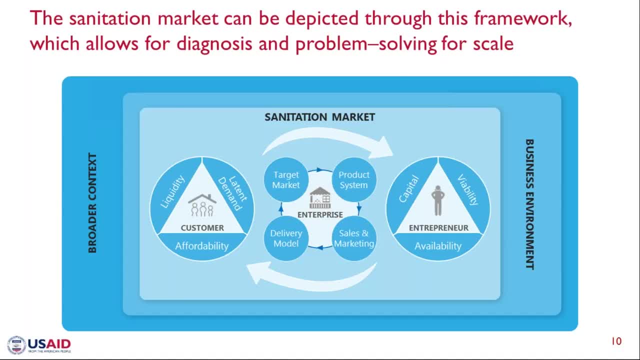 can restrict customer demand. Even if these barriers, significant as they are, are overcome, the design of the sanitation enterprise itself, what you see in the center of the schematic, is challenging. since a target market needs to be identified, appropriate product systems developed from the identified market, demand activation mechanisms. 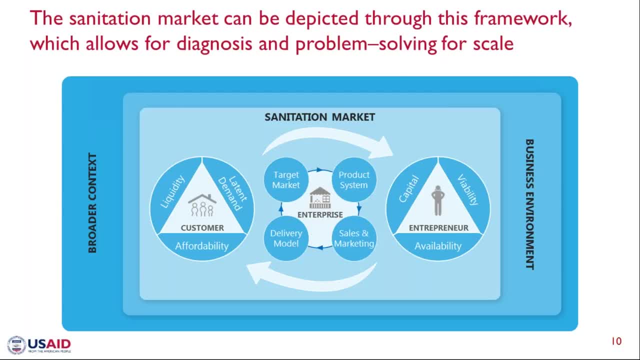 created for sales and marketing and delivery models designed to fulfill demand. However, barriers do exist beyond the sanitation market In the broader business environment. these could be around elements such as associated supply chains for raw materials such as cement market rules defined by government. 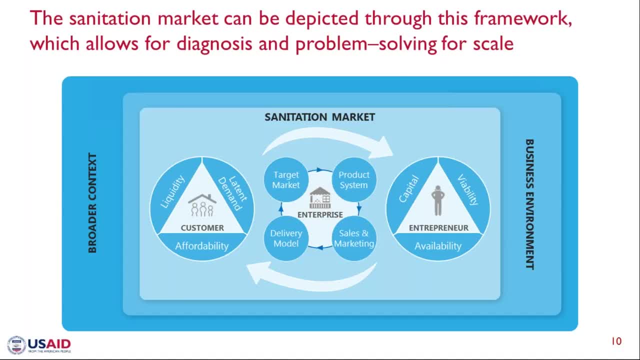 policy and legislation, and or availability of public goods. While these barriers can severely constrain the growth of the market generally, the local enterprises are not in a position to influence these. Think about it: it's hard work for an entrepreneur just to run an enterprise. 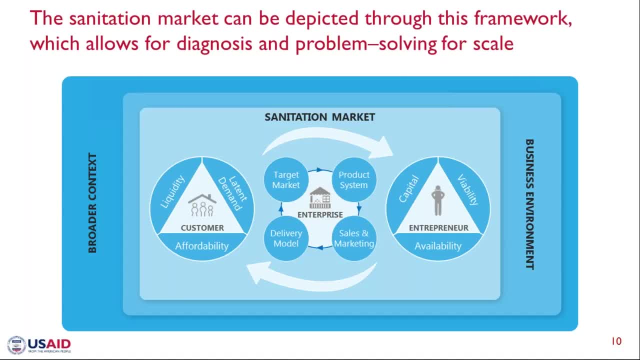 There's a lot that's going on. there's a lot of moving parts that she needs to manage. On top of that, for an entrepreneur to take over the task of influencing business environment as well is really tough. These barriers therefore frequently require intervention by governments. 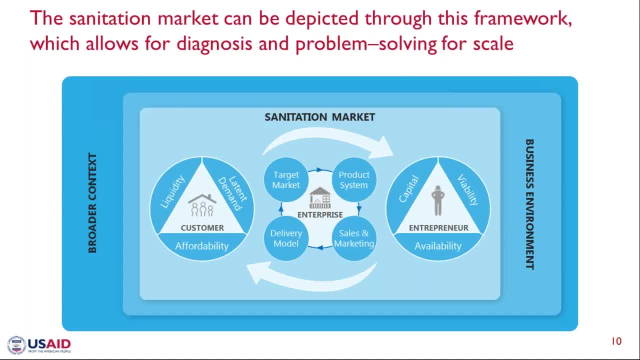 and or funders. For example, by charging penalty on landlords who do not provide sanitation facility to their tenants, governments in Ghana change the market rules, thereby increasing the potential market size for sanitation. Thank you, So there is a core sanitation market and the business environment within which the market 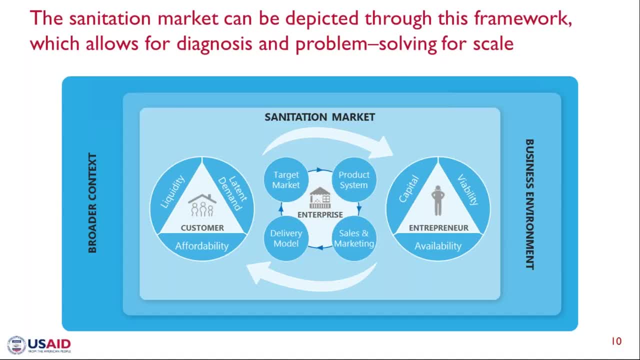 operates. However, the broader context also matters. In this layer, we highlight the role of broader context, such as social norms, macroeconomic conditions, environmental conditions and hard infrastructure, and determining if market-based approaches alone are adequate. While these barriers might not be immediately accessible, they are not. 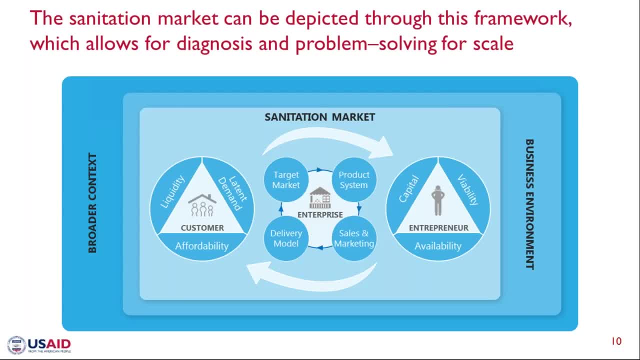 By a pure market-based intervention. developing an understanding of these variables does allow us to make an appropriate use of the approach and augment it with other complementary approaches, such as CLTS or CATS, where needed. In the following slides, I will aim to get into some detail around each of these three. 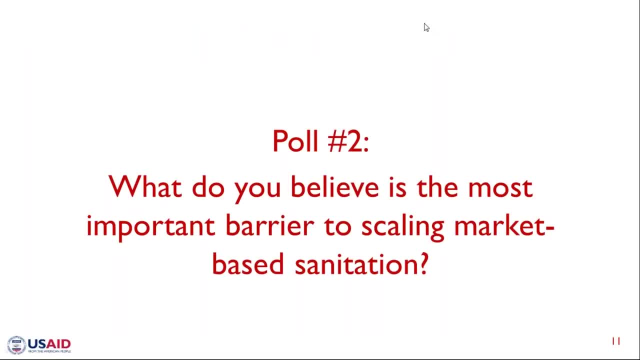 layers. Before I do that, though, I just wanted to run another poll, which was around looking at that schematic. Based on your comments, I would like to know what your thoughts are, Thank you. Thank you, And based on your experience, what do you believe is the consistently most important? 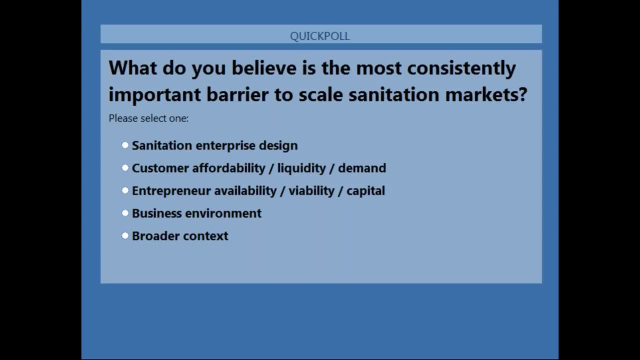 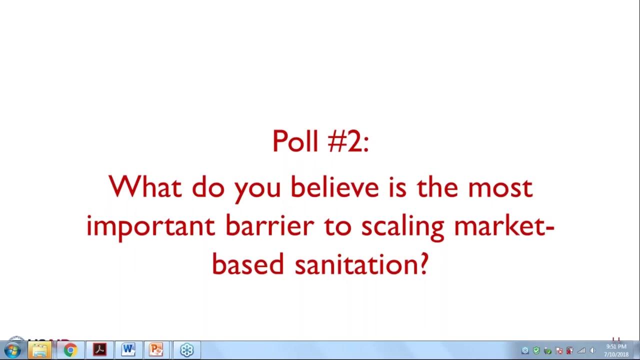 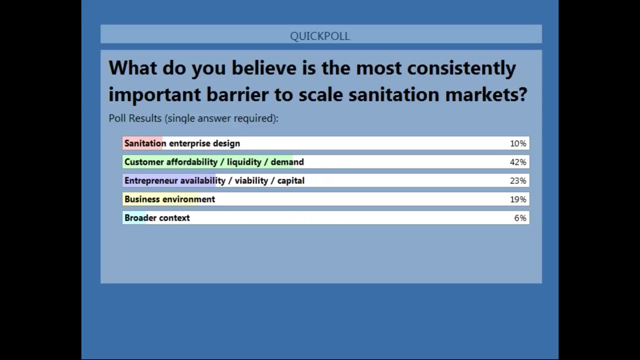 barrier for scale And I'm going to sort of hold on for 30 seconds. I'm just going to give five more seconds, as most people have voted but some haven't. So there we are multiple answers, but customer affordability or the customer has come out. 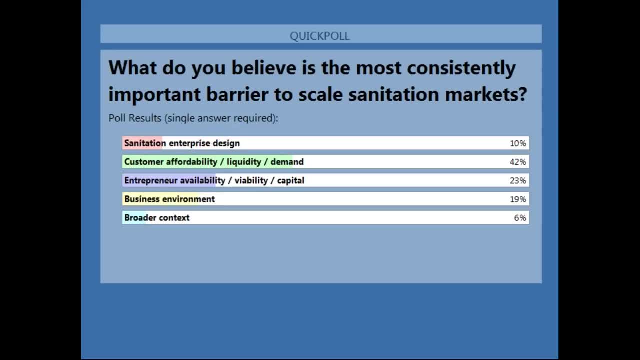 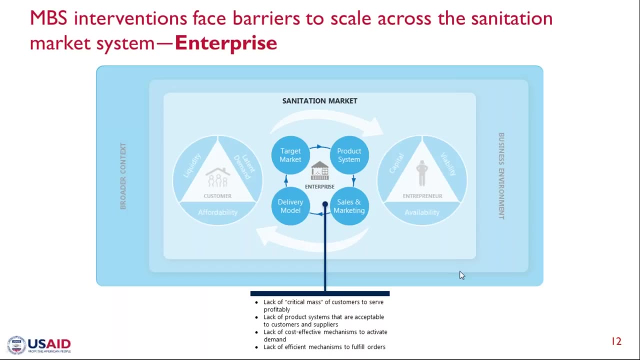 as the winner, going with entrepreneur, And then the sanitation enterprise, design, And one-fourth of the audience, at least, thought the barriers actually lie outside the sanitation market layer. It's quite interesting. So let's look at the sanitation market layer, which is what most of you thought the key. 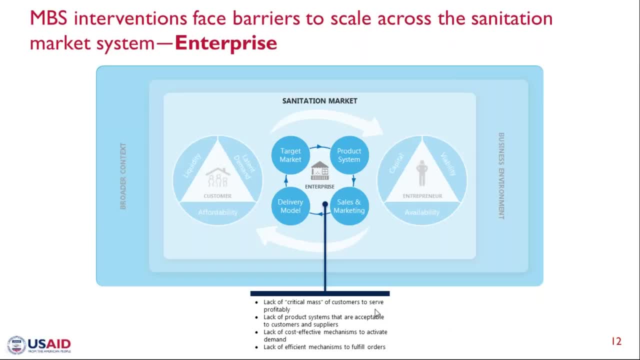 barriers lie in. So what did we think of the barriers in the key sanitation market layer, As we described earlier, this basically involves- It involves customers, entrepreneurs, who are connected via the sanitation enterprise. While designing an enterprise, the entrepreneur-implementer could be faced with four key barriers that 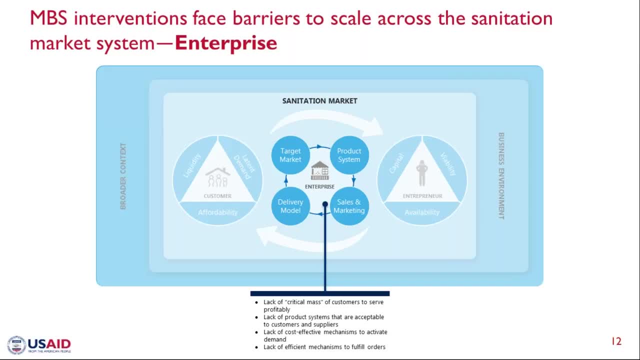 she has to solve for, namely lack of critical mass of customers to serve profitably, lack of appropriate product systems, ineffective demand activation mechanisms and an inefficient delivery model. I'll try and go into details of how these have been solved And how some of the interventions have addressed these over the next few slides. 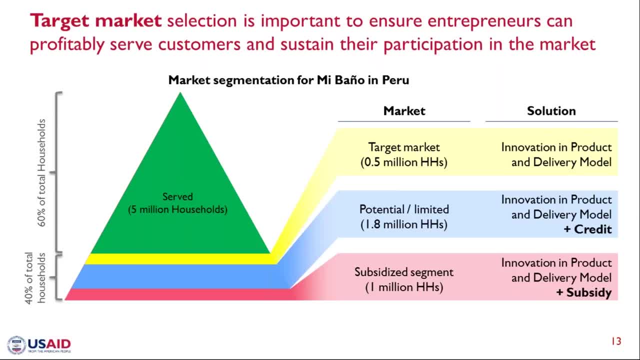 So let's start with the barrier around critical mass of customers. This can be addressed by carefully selecting the part of the market that the enterprise can profitably serve. It is important to distinguish target market selection from the broader objective of the program and indeed the SDGs. 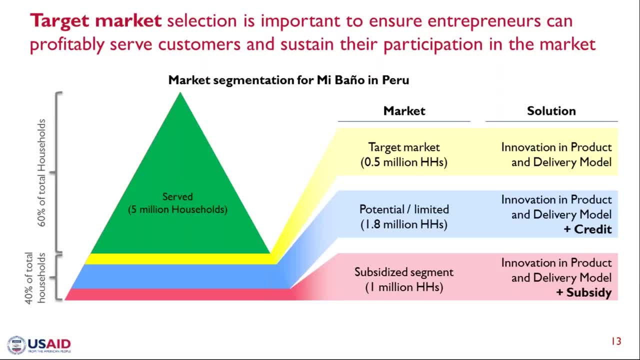 The target market selection happens at the market or an enterprise level. Therefore, it is important to select, At least initially, those segments of customers which entrepreneurs can profitably serve. What we have seen is that a sweep or a phased approach is crucial, especially in the early 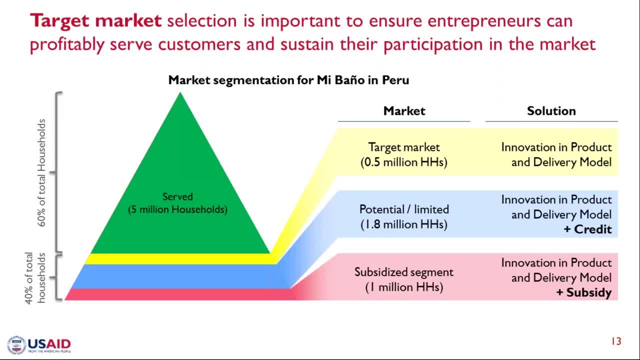 days of an MBS intervention, since it creates a demonstration effect for both customers and entrepreneurs. More customers can see the product being used and hopefully lead to increased demand. Similarly, more entrepreneurs generally get attracted to the sector, looking at the success of the pioneer sanitation enterprises. 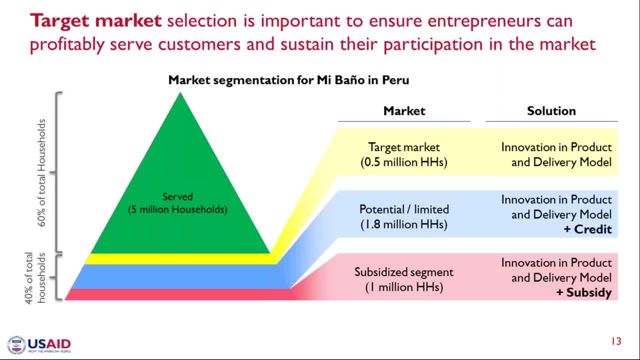 We have seen a demonstration effect for both customers and entrepreneurs. We have seen a deliberate focus on selecting a market rather than an approach of targeting everyone. in the IDE Cambodia program, in the BMGF funded 3SI intervention in Bihar, as well as WSB's. 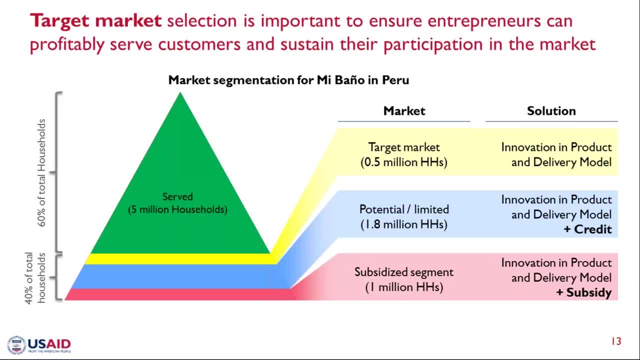 program in Peru. The figure on the slide describes the Mi Banier program in Peru. In this example, as you can see, the program started. The top 60% of the market was already covered by the commercial 12s and it was the bottom. 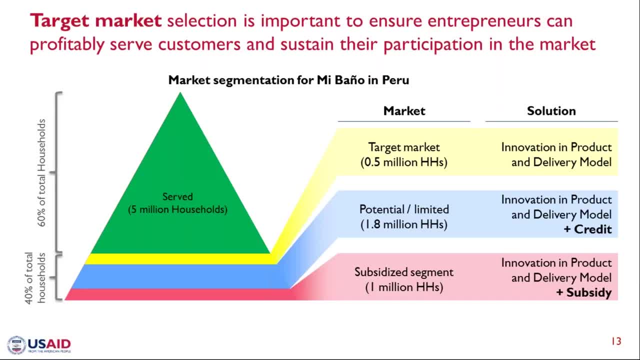 40% of the population that needed new solutions. The program segmented the bottom of the pyramid into three layers that could be served either through innovations in product system and delivery models, or those that also needed either credit, which is labeled as potential limited here- or subsidy- the subsidized- 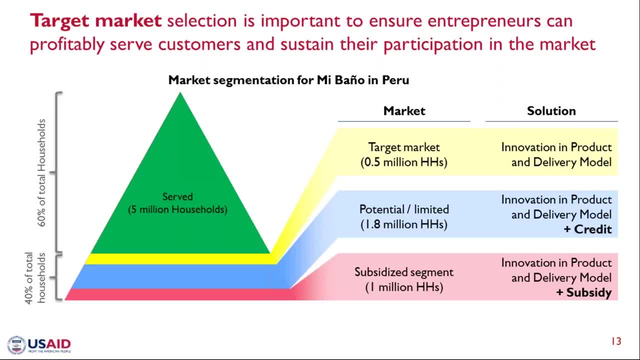 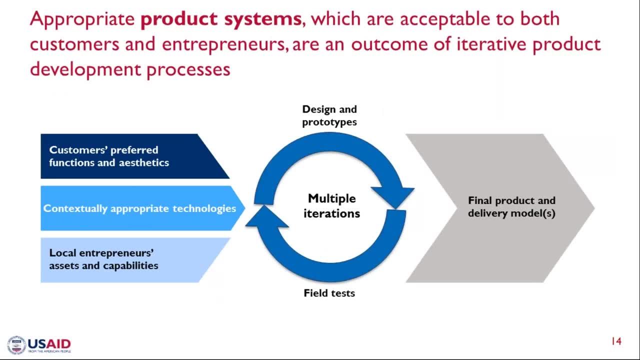 segment. In this case, the program made an explicit call to start with market segment, just below the currently served markets, which amounted to half a million households. So we have selected the target market. now what? How do you know which in the product system and delivery models It is important. 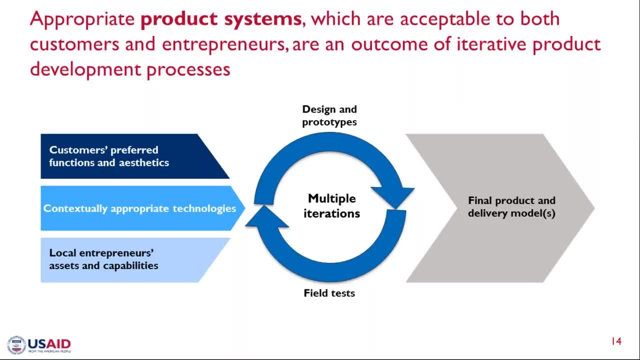 that the market can offer appropriate product systems. By appropriate, we mean products that are desired by the customers and can be profitably delivered by the enterprises in the market. More often, what we have seen is that the options available to the customers are either too expensive or of poor quality, Since the customer and market context is different in every program. 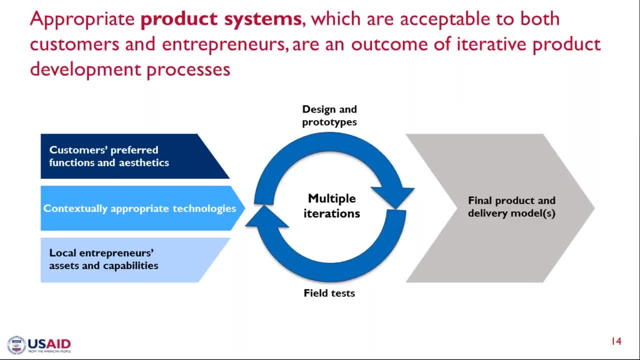 we recommend that an iterative, human-centered design, this formative approach, be used to arrive at the product system. This was done not only in the IDE and the 3SI programs I mentioned earlier, but quite early on in Mozambique, where the dome sand flats were designed to do away with the need. 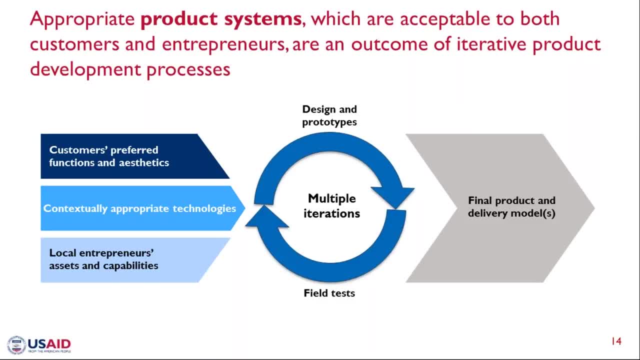 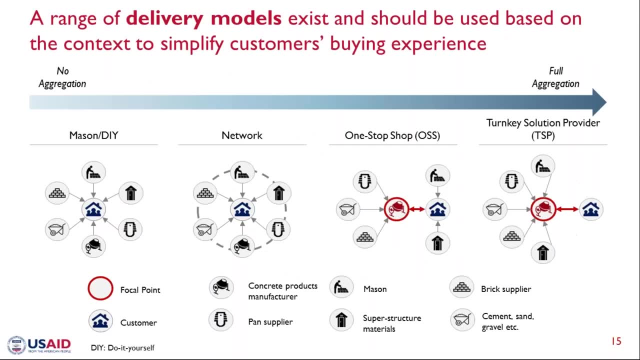 for rebar, which was both in limited supply and expensive, while at the same time addressing the durability concern that the local customer had. This brings us to the next part of the enterprise design, that is, the delivery model. As you can see from the schematic, while we catalog the different potential delivery models, we do not make any 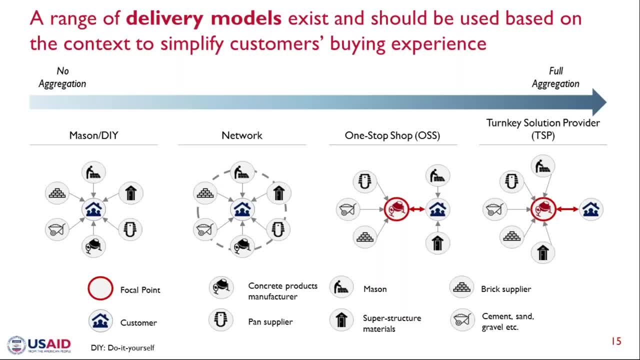 recommendation as to which delivery model is the best. That depends a lot on the context and the capabilities of the entrepreneur. However, a concept that we have introduced in this report, and one that I will like to highlight, is that of the focal point enterprise. We define a focal point. 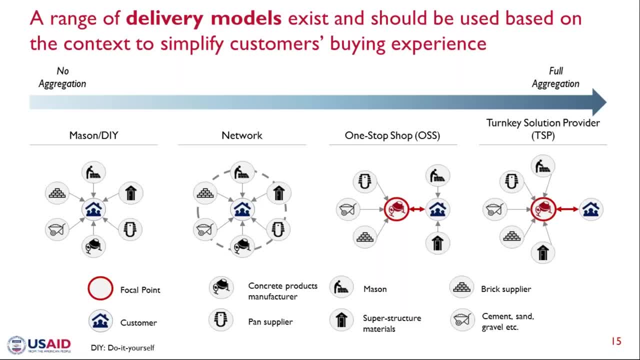 sanitation enterprise as the customer facing business that aggregates products, product components, services, information or a combination of these, depending on which delivery model we are talking about. This, therefore, is the go-to enterprise, in some ways, for a customer looking for a sanitation solution. 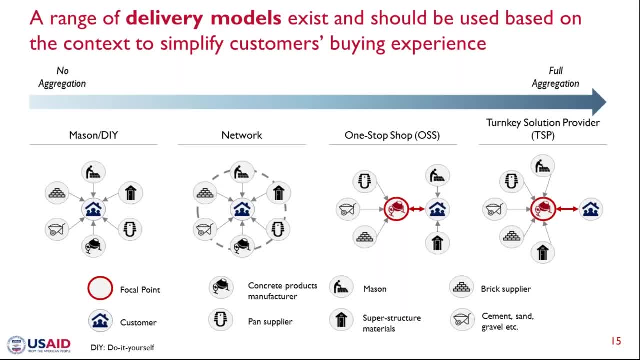 For instance, there is no focal point in a DIY outfit as in a network model, while there is no created designed focal point, the player, the customer approaches can play of role of one because they are creating as a loose network and affiliation. However, in the more aggregated model, such as one stopped, 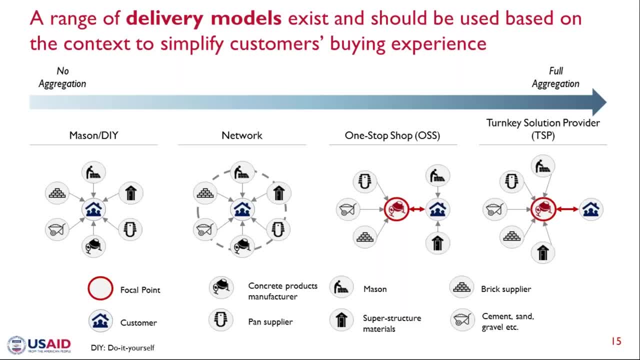 shop or the Toiki Solution Providers. there is a defined focal point that interacts with the customers and covers either a part or whole of thie nr Maine as perto oposite. So you can see in the dues model that the entire process for the delivery model will be Min tricks based. 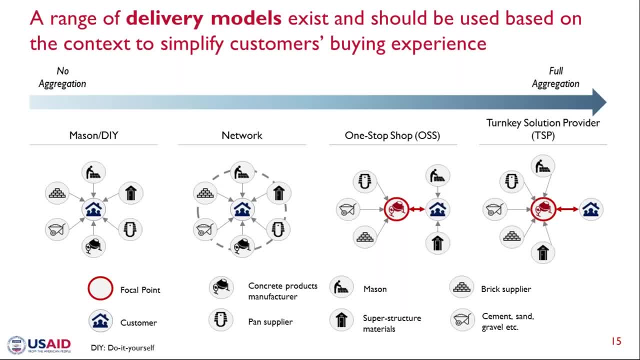 into one начini and all saucebox platform can be succeeded from inside the swear. here is a defined focal point that interacts with the customers. There comes either a part or whole 🎵 buying process. I know this is a fairly busy slide. there's a lot to take on, so I 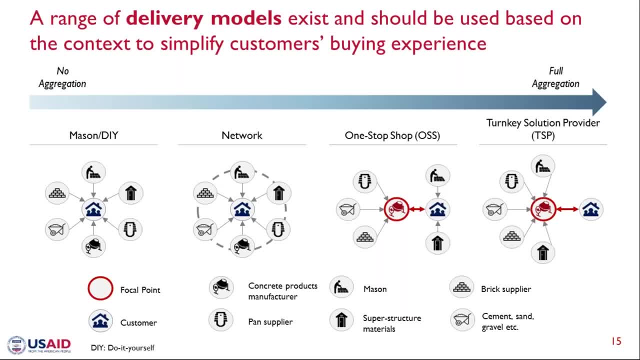 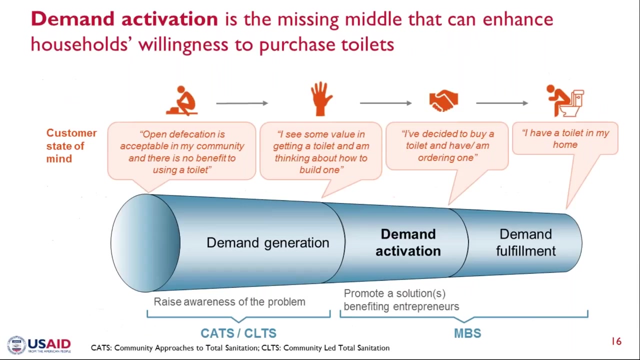 just wanted to mention here that this is the figure numbered 11 in the report. So for further details on each of the models and examples highlighted on the slides, please refer to section 4.1.4 in the report. So we have innovated on product system. we have innovated on delivery model. is that? 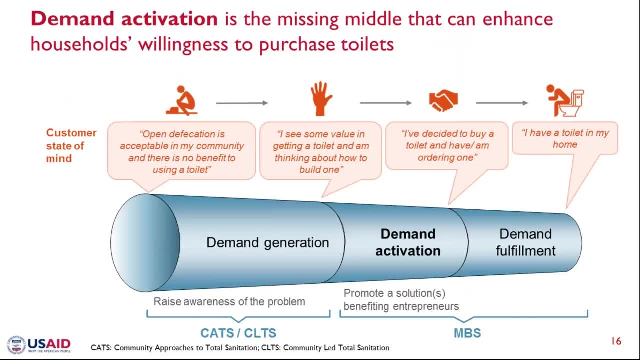 enough What we found. normally it isn't. Supporting the customer on their mental buying journey is equally important. The schematic on the slide, which for reference is figure 10 in the report, indicates the behavioral stages that have to be navigated for a toilet. 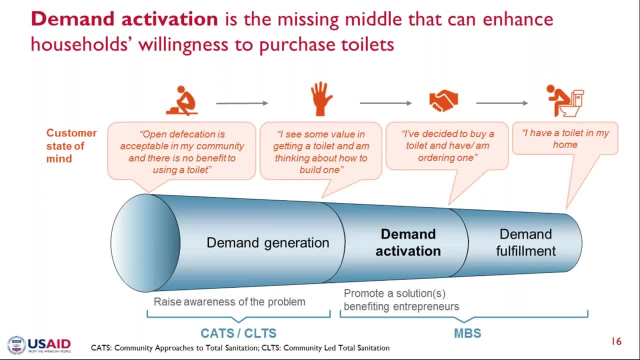 purchase At the extreme end, as you see, is a customer for whom ODE is acceptable, So we've done the same thing for the product system, which is based on their and therefore has no need for a toilet. the aim that we all have as programmers is to get this. 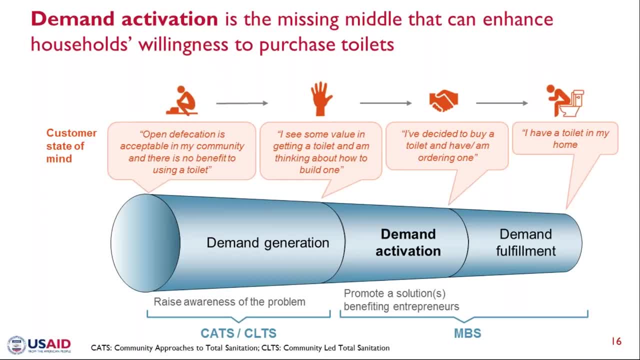 customer to actually buy a toilet. as a sector, we've been good at creating demand through clts, cats and other such mechanisms that allow us to get customers to see the value in getting a toilet. we are calling addressing this phase of the customer journey, ie moving them from the first. 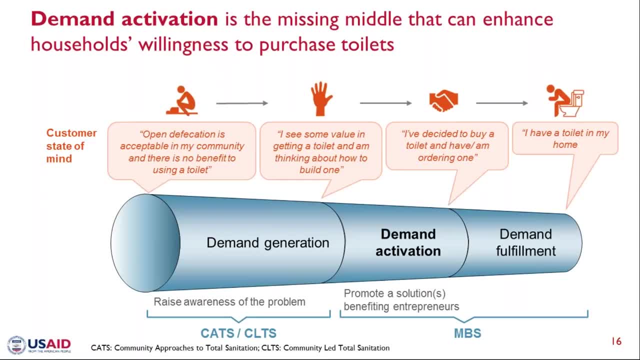 schematic to the second, from open defecation to seeing, i see some value in getting a toilet- demand generation, which is essentially around raising awareness of the problem. at the same time, all of you who have worked in market based sanitation would have worked on the supply side to build delivery models to entrepreneurs, to think about product systems. 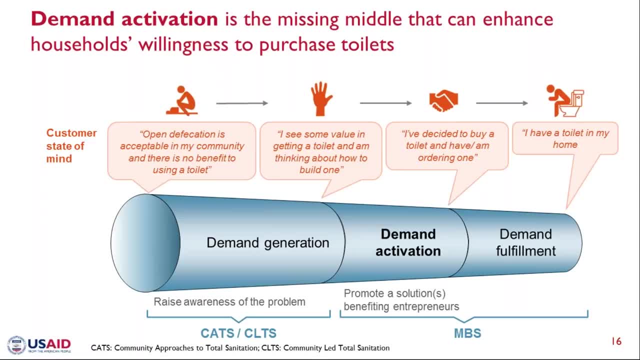 and how they get to the customer. this is what we are calling demand fulfillment. what we have identified as a key criteria for success is the missing gap between the two, what we are calling demand activation. this is necessary to move the customer from the first schematic to the second, from open defecation to seeing a toilet. 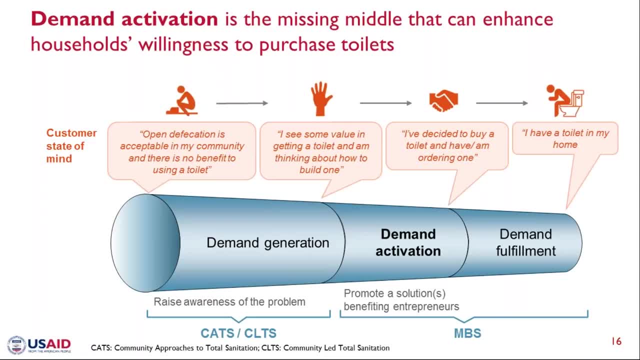 the toilet purchase from a consideration where the customer sees some value in getting a toilet, but still maybe lowering his needs of hierarchy, to an actual purchase decision. this has been successfully done by several interventions, such as watershed in cambodia, ide in cambodia, psi and bihar, usually through field sales agents. 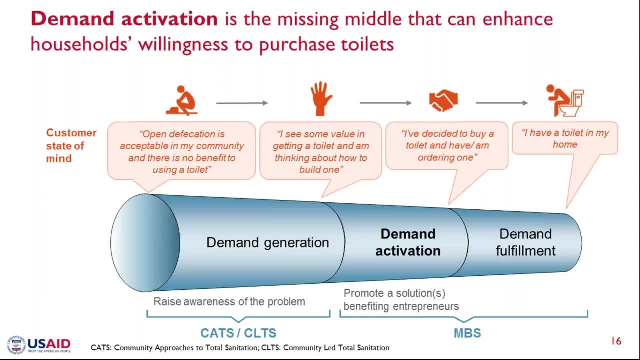 who are paid commissions either directly by the entrepreneur or by the program, and it's very important that the organization is designed to provide the customer with the best possible service and the most efficient and effective service that they can get that are needed in designing an effective enterprise. 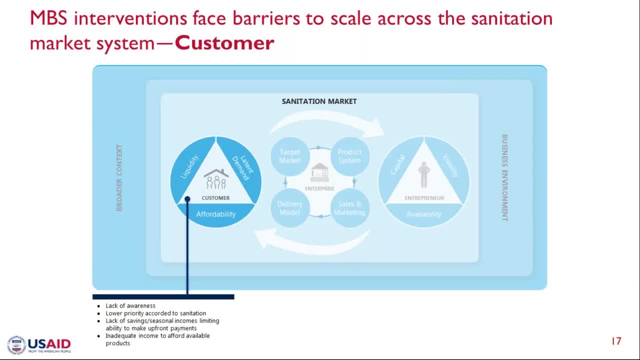 now let's look at another element in the sanitation market layer, namely customers. no market can survive without customers who are willing and able to pay for the products being offered, and this is exactly where the barriers to scaling market based sanitation lie. as discussed earlier, demand generation is not. 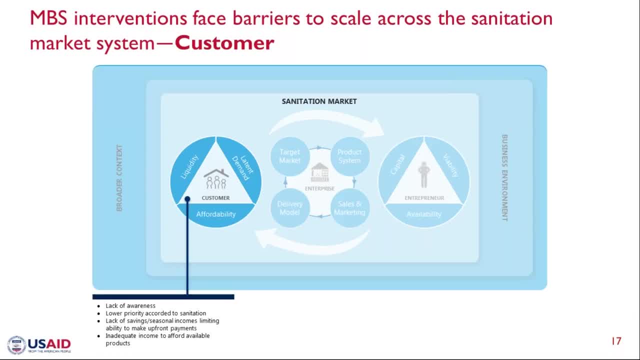 something that mbs can do, as no single sanitation enterprise will be able to make the requisite investment. hence, lack of latent demand, which can be activated through demand activation mechanisms which we're discussing, can be a barrier to scale. in addition, customers might be constrained in making the requisite payments due to a lack of savings or seasonal incomes, leading to the 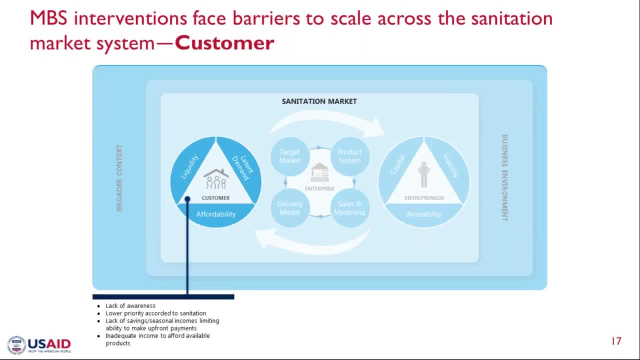 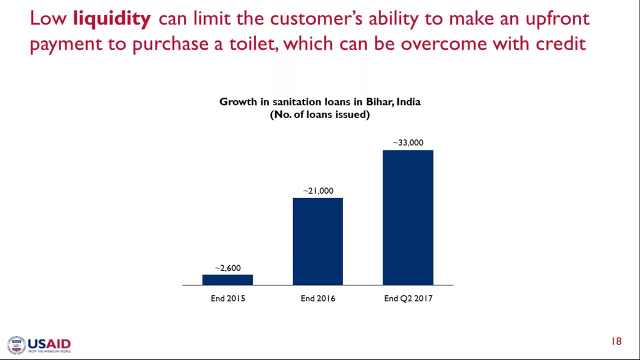 liquidity barrier or, in other cases, simply might not be able to afford the available product. we will discuss these later in this presentation- liquidity and affordability questions in the next couple of slides. liquidity as a challenge can be addressed through provision of credit. we just put up an example of beha, where psi partnered with friends of women, world banking. 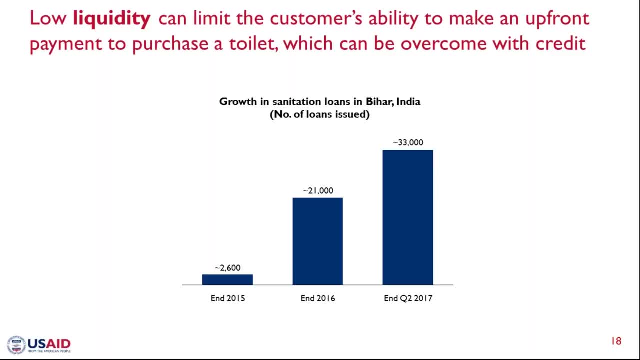 to provide credit to consumers. as you can see on the slide, there has been a significant demand for sanitation loans from the time the loans were made available, highlighting the fact that, at least in beha, there was a reasonable segment of the population for which liquidity was a challenge and not affordability. 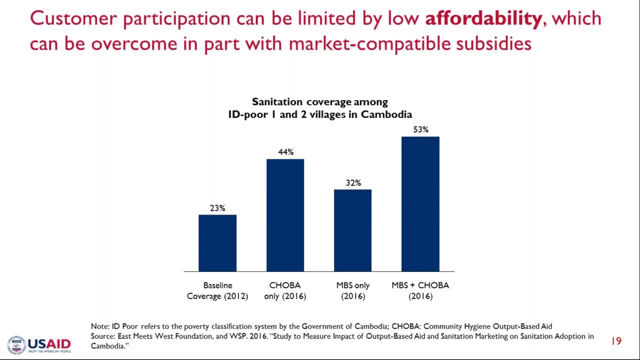 but what, in situations where affordability is, is the problem? our research indicates that well targeted subsidy can significantly improve the toilet object. and when i say well targeted, the key emphasis is that the subsidy should not distort the pricing of the market for market-based players. the chova example illustrated on the slide is a case in point. 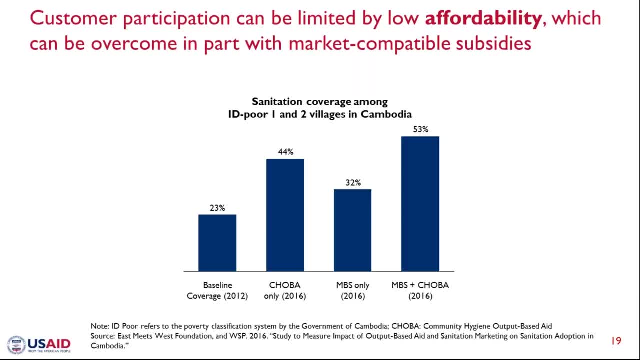 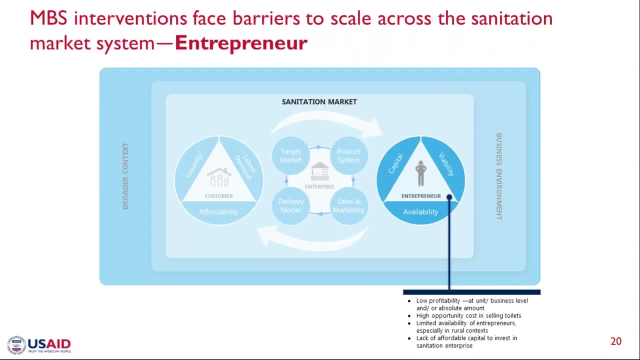 but drrct clearly showed that while subsidy only and mbs only programs both had an impact on uptake, combining the two led to much better outcomes among the bottom 40 percent of the households in the country. moving on to the next and final element of the sanitation market layer, which is the entrepreneur, 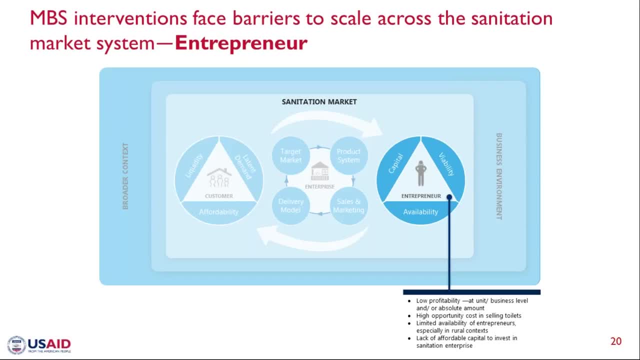 barriers to scaling mbs related to entrepreneurs start with the availability of entrepreneurs-in-source surprises there. I guess This is especially true in rural environments where there are no sanitation entrepreneurs and is further exasperated by the low profitability both at the business and unit level of the. 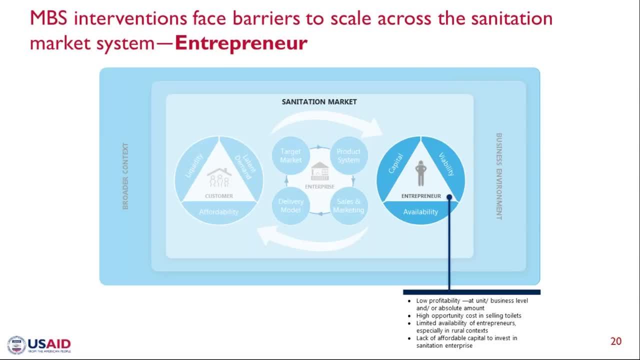 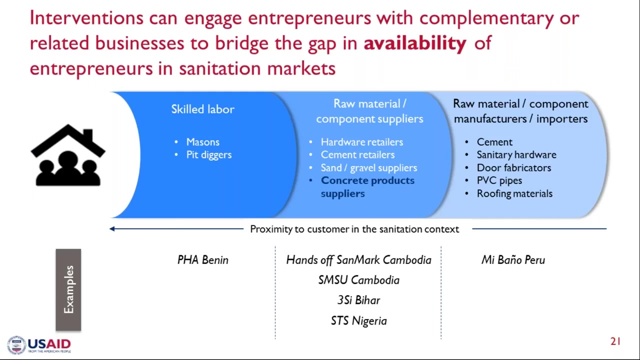 sanitation enterprise and potentially the high opportunity cost of engaging in sanitation versus other potential businesses. Where the entrepreneurs do exist, they might face significant barriers in accessing capital to expand meaningfully into the sanitation market. Let's look at the availability barrier. While there might be a lack of sanitation entrepreneurs in the markets, 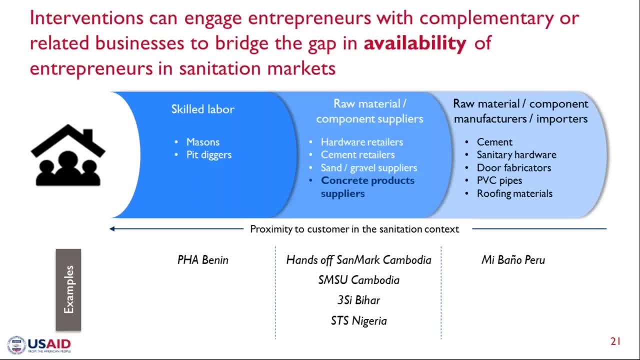 that interveners go to. our research indicates the capabilities and attributes required to run an enterprise are not unique to the sanitation sector. Therefore, the opportunity exists to leverage existing entrepreneurs in the adjacent markets. On the slide you see, this is indicated by the various arcs in the diagram, going from darker to light. 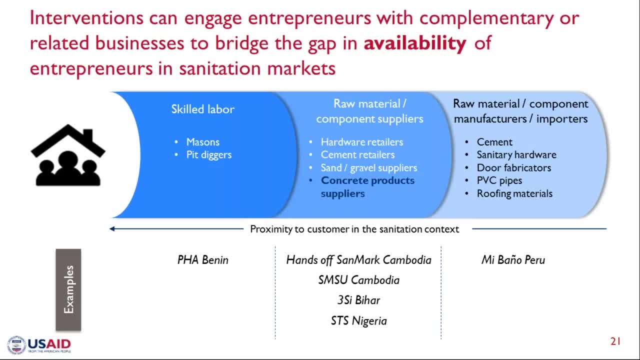 depending on how far away they are from the customer. For example, in Cambodia ID and Watershed, they recruited entrepreneurs from a pool of existing precast concrete products manufacturers to create sanitation enterprises. One thing to note, however, here is that there is a lack of sanitation enterprises in the 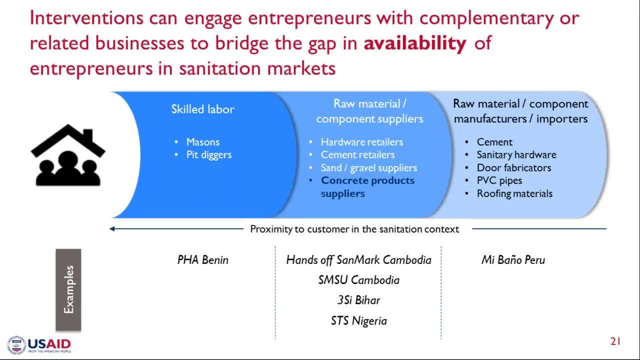 market. There is a challenge they might face, which is around lack of customer trust for their new offering, especially if they are, let's say, in the furthest arc, that is, on the slide, or completely unrelated businesses, Even if the intervener can convince entrepreneurs to get into sanitation. market access to 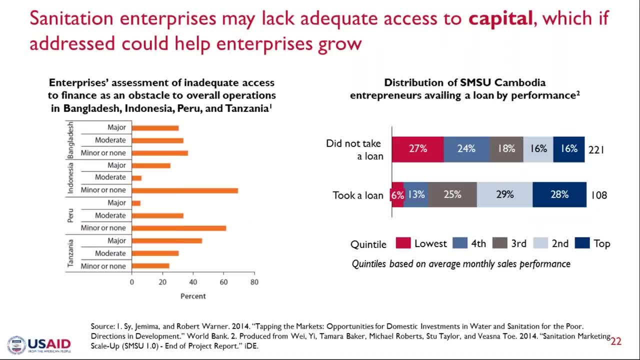 capital is a barrier to scale. World Bank analysis shows that in most markets with low penetration of supply chains, capital was highlighted as a constraint by the entrepreneurs. This, if you see on the left hand side of the schematic, is highlighted by the number of enterprises which pointed out to inadequate access to. 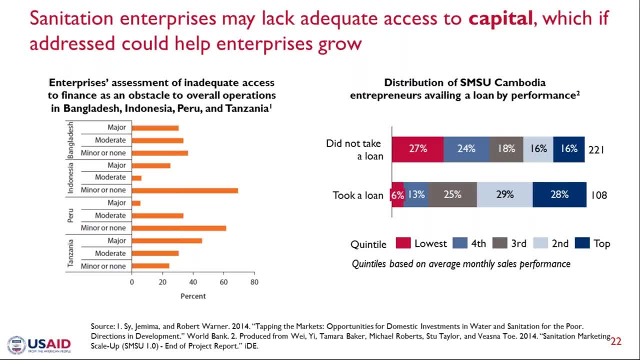 finance as a major or moderate barrier versus those that did not. Also, in Cambodia, IDE saw that the enterprises that took loan tended to perform better in the sanitation market In India. they were able to get more than those that did not. This you would see on. 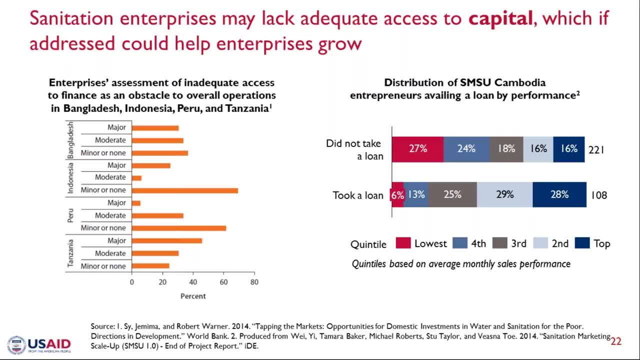 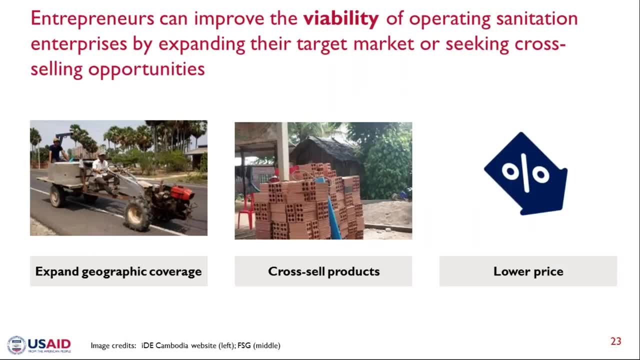 the right hand schematic around the quintiles and the population sets of entrepreneurs who took a loan versus who did not. In areas where entrepreneurs exist and might have access to capital, the viability of the sanitation enterprise still remains a challenge Among the many factors that can impact. 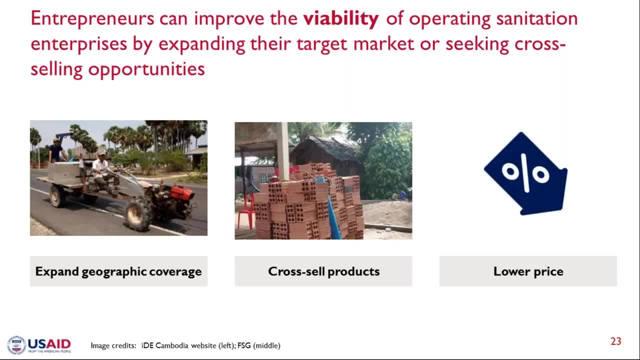 the viability of sanitation enterprises. low turnover and unit profitability, a margin or absolute dollar terms are often the major challenges that face rural sanitation enterprises. The three ways we have seen entrepreneurs improve the viability of their sanitation enterprises are what we have highlighted on the slide, The first one being expanding geographic coverage. 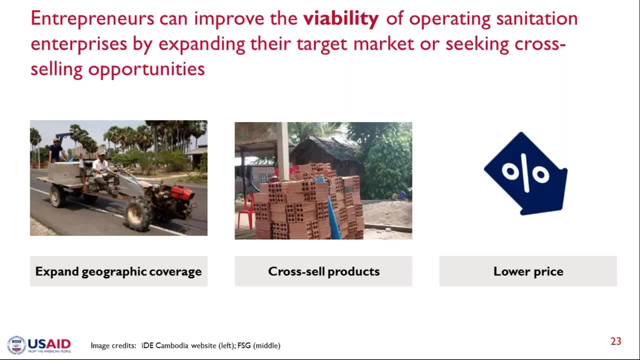 getting into adjacent villages or blocks, which is possible only where the transportation infrastructure is good. The other thing to do is cross-sell products to extract economies of scope. start selling rings for other purposes, cement pillars, tiles, to increase the share of wallet that's coming through from the customer. 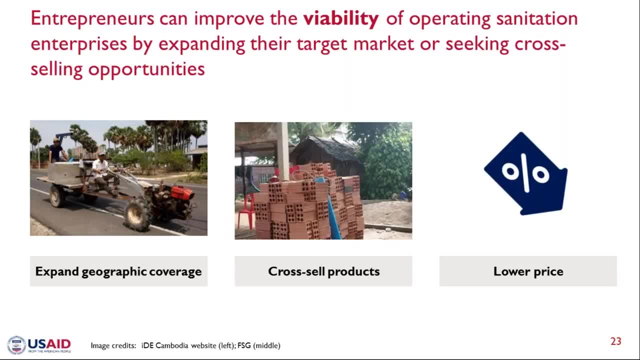 Or, lastly, by lowering price to increase sale, and this is a bit of counterintuitive for most entrepreneurs and could be a difficult lever to pull Our watershed in Cambodia managed to convince the partners to do just that: lower prices to improve sales, and the 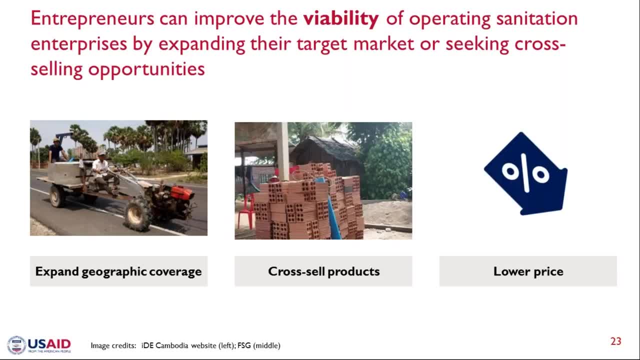 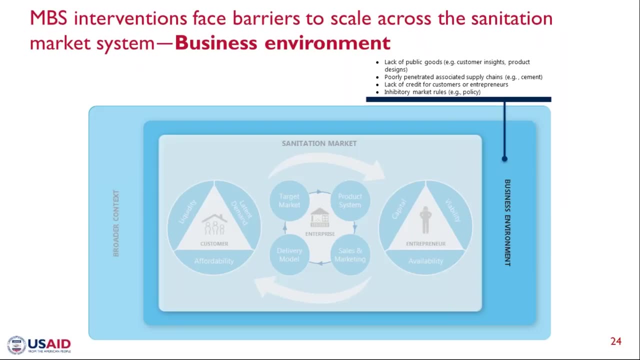 partners did see an increase, a reasonable increase, in their absolute dollar profits. So we talked about customers, entrepreneurs and the sanitation enterprises that form the sanitation market layer. Now let's move to the next layer, which is the business environment, The sanitation market as. 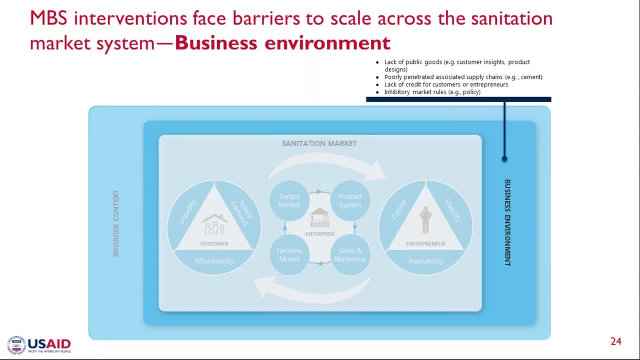 with any other market, operates within the business environment, which could either hinder or support the growth. The factors that can hinder its growth fall on four vectors. These are lack of public goods, such as market intelligence. poorly penetrated supply chains of key raw materials, such as. 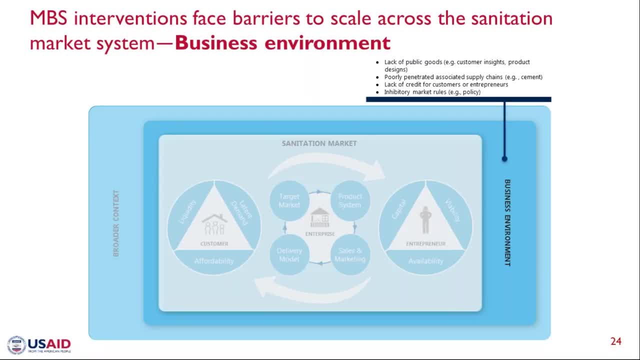 cement sand. lack of financial services. infrastructure for provision of credit We talked about. credit can be a key lever to improve, address the liquidity barrier. that's where, let's say, a microfinance institution does not exist and the traditional banks might not be interested. what do we do? And inhibitory. 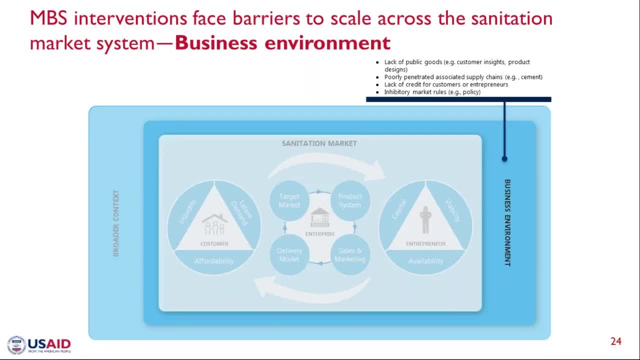 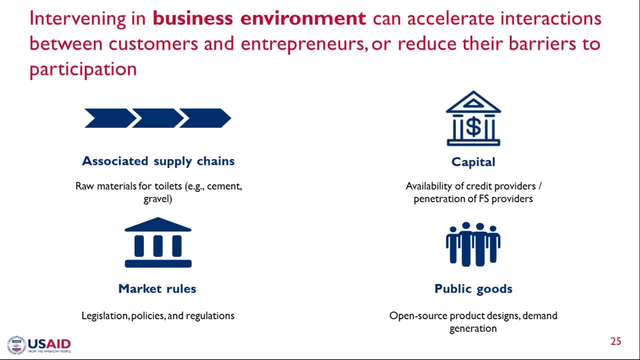 market rules. if, for example, the tariffs on plastic are very high, then what happens in those markets? So let's discuss these four in some detail. Associated supply chain, I guess, is the easiest to grasp. The delivery of a toilet requires that the various raw materials are available to the consumer. 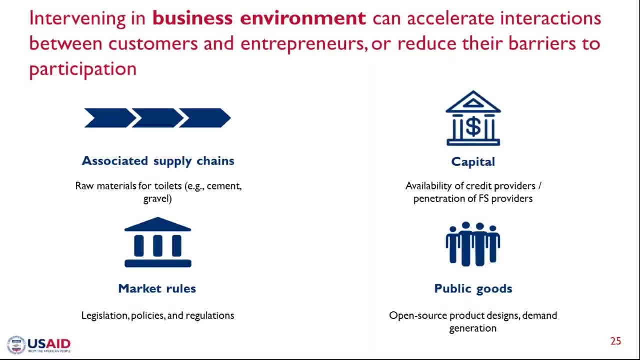 They are available locally or can be easily made available locally. If the supply chain for these raw materials are not well penetrated, then it can impact the growth of sanitation markets because you are now asking the entrepreneur to not only source from further away but incur those costs in sourcing that And 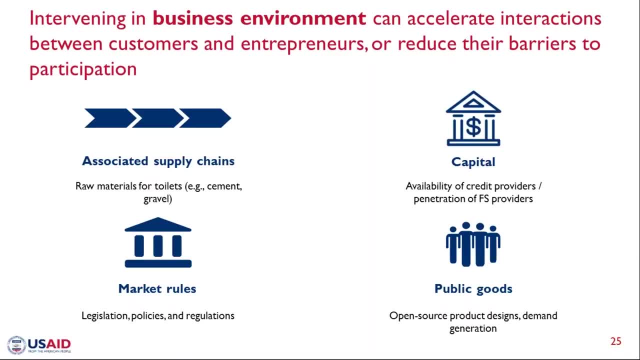 as I said earlier, while providing credit is something that intervener can work on, actual provision in a substantial way requires that the financial service providers, such as microfinancial institutions, mobile money players or other traditional players like banks, are present in the target markets. Funders can encourage these financial 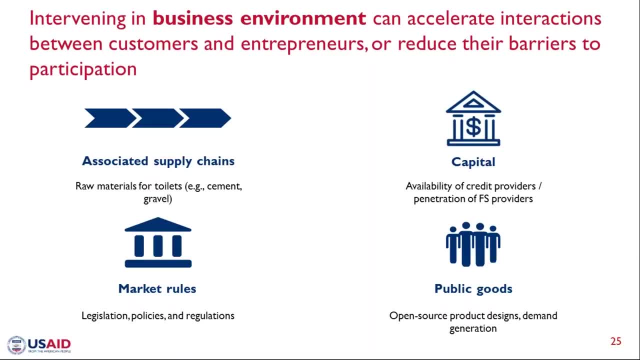 services players to get into the space through provision of either grants or credit default guarantees. Market rules are an interesting one. These are the regulatory tools, and we classify them in three, which is rules, regulations and policy, That various level of regulation and regulation can be used to create a. 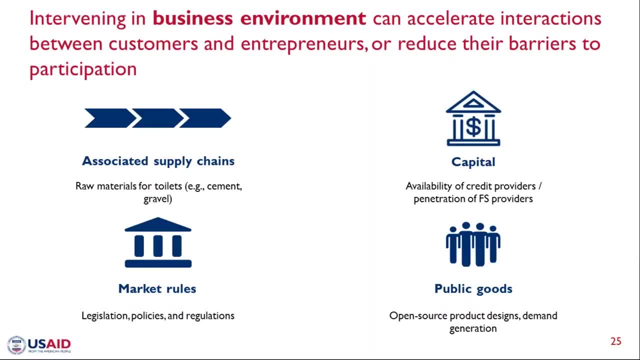 system that can help to protect the products and services of the consumer. So these are the levels of government, right from the federal to a district or a county. sub-county level of government can set which can either support or hinder market. Sometimes, actually, an initiative in one of these areas can actually remove a barrier in another part. 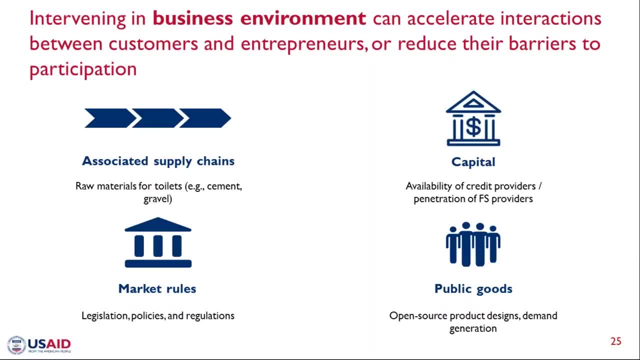 of the business environment. For example, in Mozambique- example I was mentioning earlier- government intervened to ensure availability of cement to sanitation providers, Thereby making a policy change which impacted the associated supply chain barrier that the entrepreneur was facing. Lastly, there is a challenge of public goods. 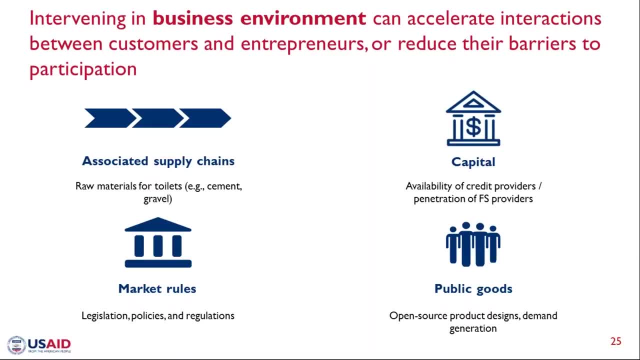 Now we define public goods as resources that can benefit the whole market but might be too difficult for one single entrepreneur to invest in. These include elements such as market intelligence, specifically in case of rural sanitation- appropriate technology. these could be around monitoring mechanisms, around best practices sharing. 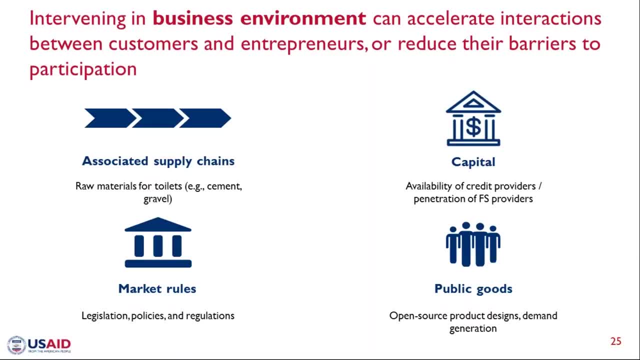 So those are elements which are useful for the entrepreneur community at large, but a single entrepreneur would find it very difficult to invest in them. However, funders are well-placed to provide support on creation and dissemination of such public goods. However, the effectiveness of MBS. 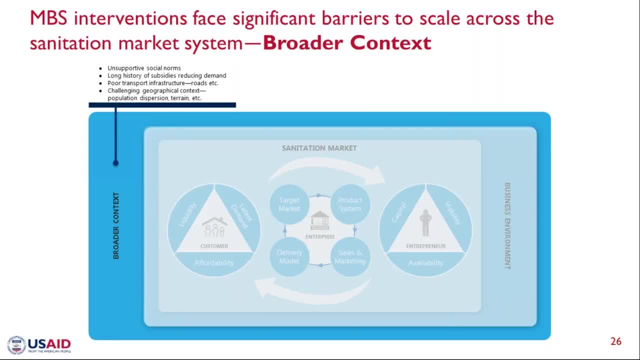 MBS is dependent on the broader context within which the markets are operating. The broader context should drive the choice of intervention strategy. Going with MBS alone or as part of a portfolio of approaches depends on four specific criteria. These are existing social norms around open dedication. hard infrastructure such as roads. 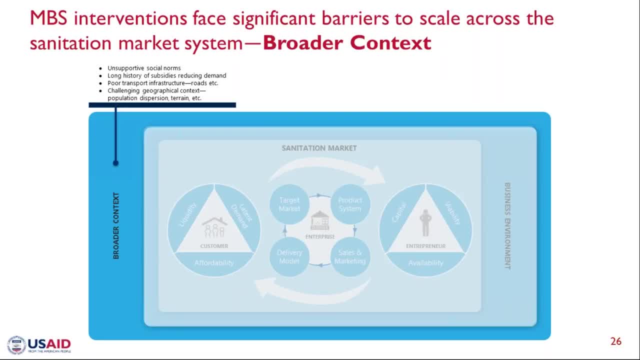 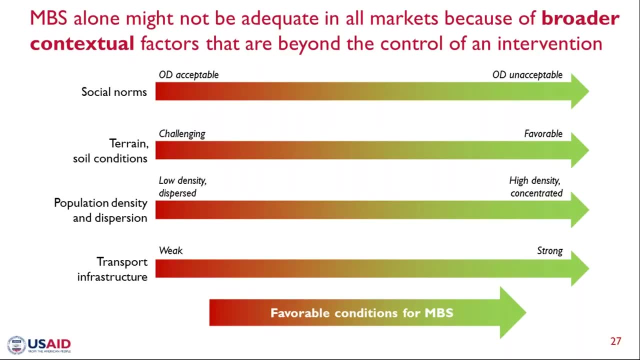 macroeconomic factors, such as interest rates, And the environmental context, Valley conditions, such as topography or soil conditions. As you can see, the effectiveness of MBS as an approach improves as we move to densely populated places with good infrastructure where OD is frowned upon. 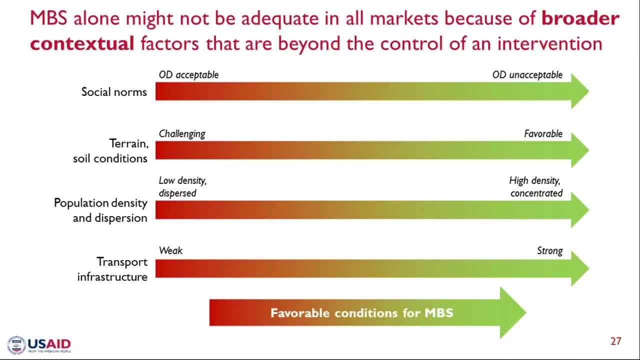 No surprises there. However, if you'll go to the left-hand side of the spectrum that we have on the slide, where OD is acceptable, there's low density, highly dispersed population with weaker infrastructure. MBS alone does not Okay, will not be the right approach to go in with. There might be a need there to complement. 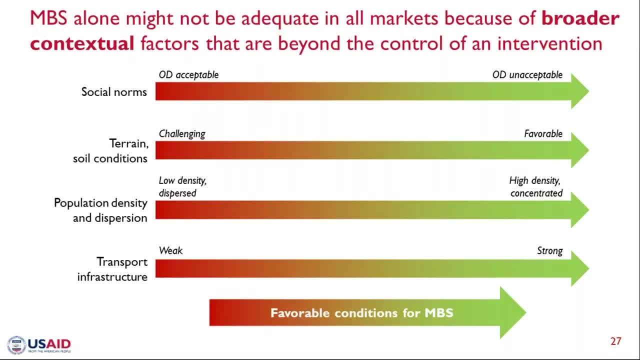 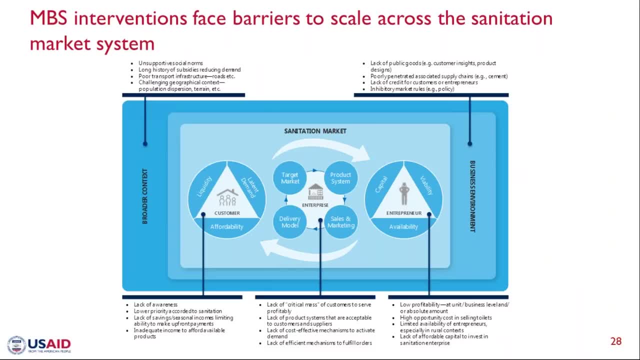 MDS with other approaches to ensure that we are meeting our targets. In summary, as you can see in the schematic now, which is just basically a summation of all the barriers we have talked about, across various layers and elements that an intervention has to address and overcome in order to truly take the sanitation market to scale, 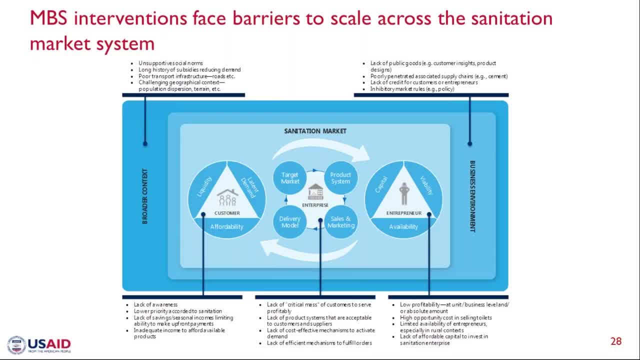 And therefore it's hard work. Our hope is that this schematic can be used as a diagnostic tool to evaluate a local ecosystem by both funders and implementers as part of the intervention designed to identify barriers that need to be addressed by the intervention. 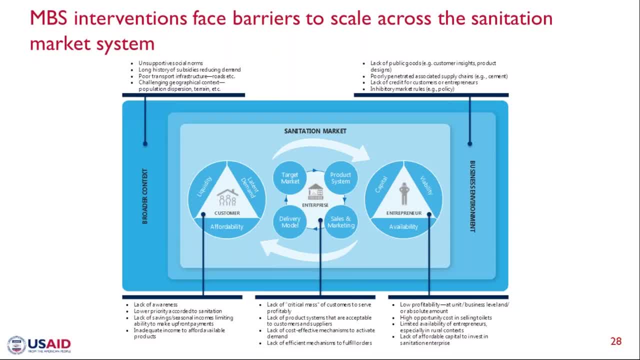 Thank you. Having seen the myriad of barriers that we have talked about in context- business, environment, the sanitation market itself- I want to run the final poll, And this was just to see: after listening to the last 20 minutes, has your opinion changed on which is the most? 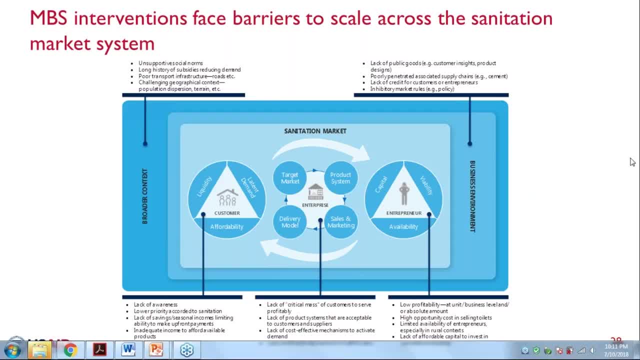 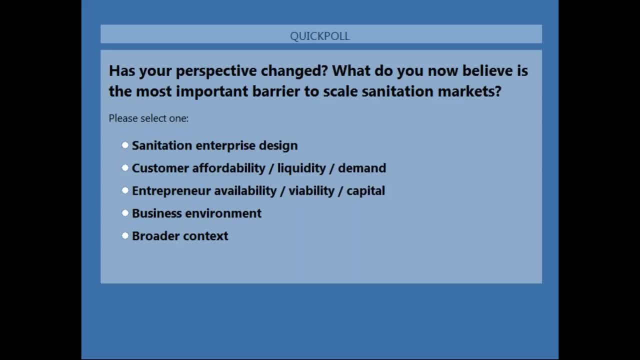 important barrier, or does it remain the same? So I'm just going to launch another poll and would be obliged if you could participate. Okay, I'll again let it run for around 30 odd seconds. Okay, thank you very much. We've had 60% of people voting, so I'm just going to let it be on for another five seconds. 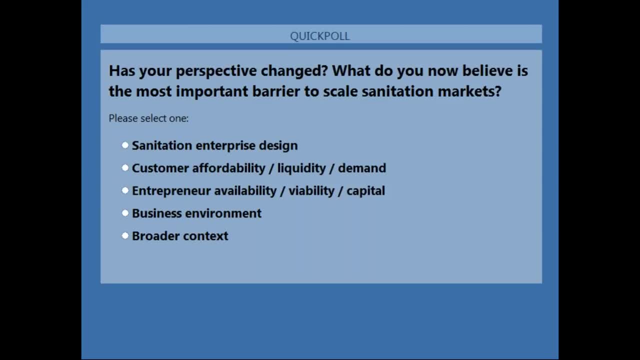 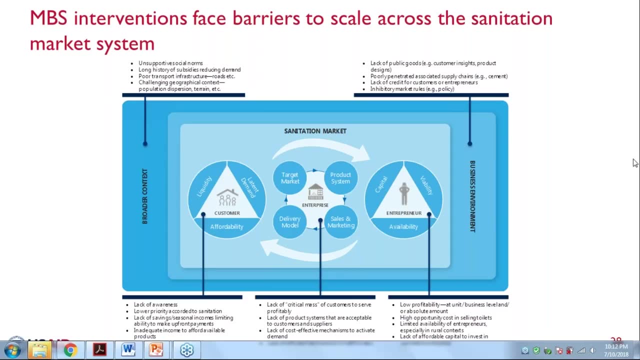 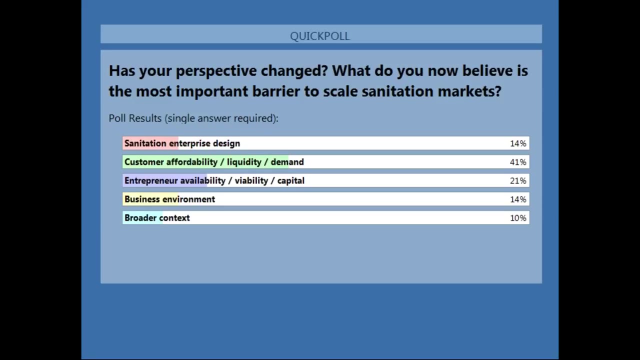 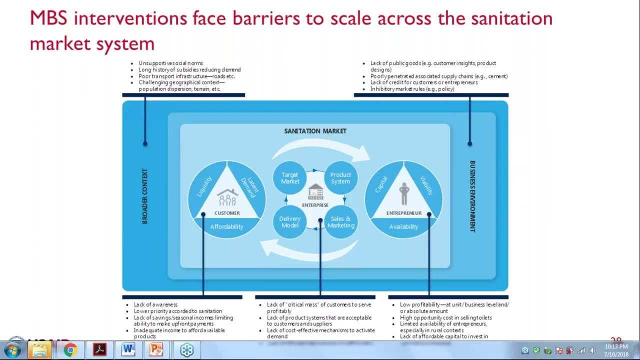 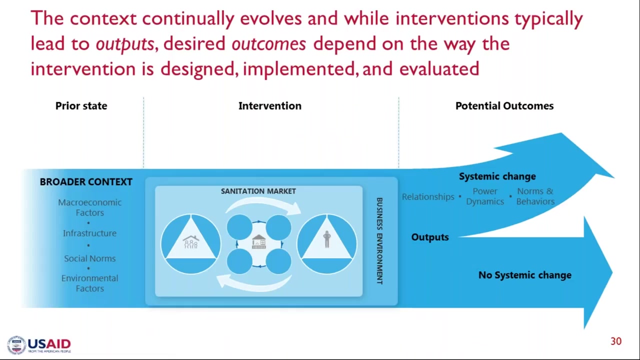 Okay, so, sharing results now. Well, that doesn't seem to have been a much of a change in the process. Okay So, moving on, One point that we did want to raise was on the potential of MBS interventions to lead to systemic change. Now, while we do say that MBS interventions cannot change the 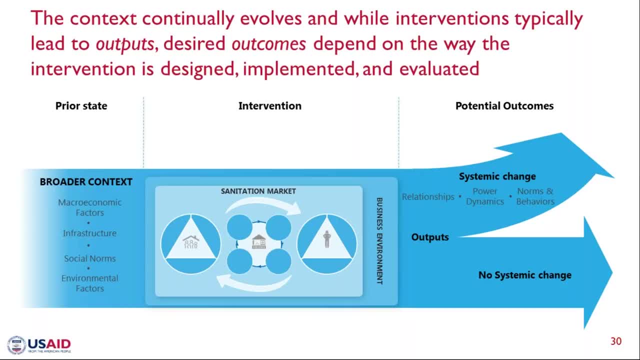 broader context and we make that point in terms of how we lay out the layers in our model. We do believe that it can certainly strengthen and provide momentum to the positive change in the underlying vectors which create the change in broader context. The important thing, 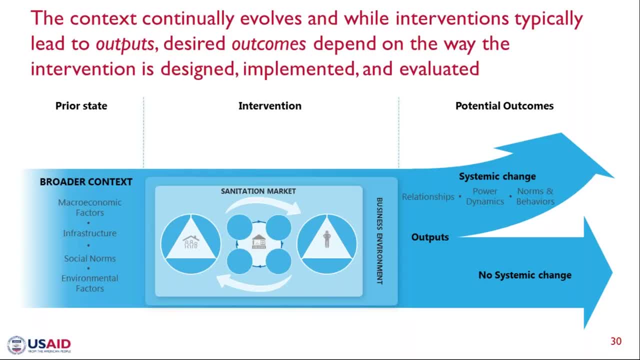 to remember here is: the context is always evolving, whether or not there is an intervention. The intervention itself is an opportunity to steer the change in a positive direction. However, that can only happen if at the outset we aim to measure the change in a positive 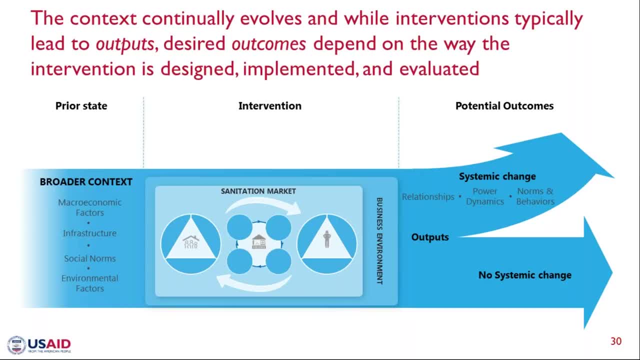 direction If, at the outset, we aim to measure variables that go beyond the outputs, such as number of toilets, number of entrepreneurs, to actually measuring underlying variables such as relationships. Have we changed the relationship between the government officials and the entrepreneurs? Is it still an antagonistic relationship or a synergistic one? Power dynamics. 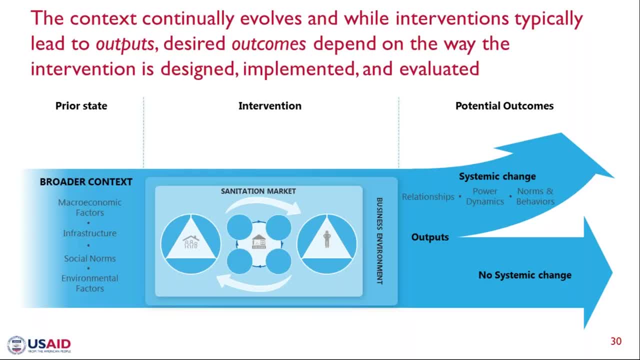 the social norms. Well, a market-based intervention would really be able to change social norms itself. has it supported positive social norms or not? Over a longer period, we believe it's entirely possible for an intervention to deliver thousands of toilets without leading to any systemic change. However, what we should be aiming for is to drive change on those. 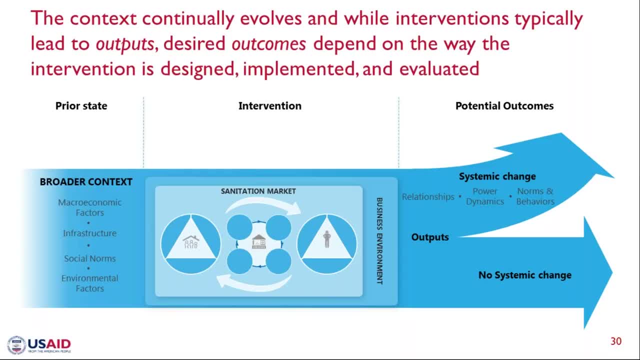 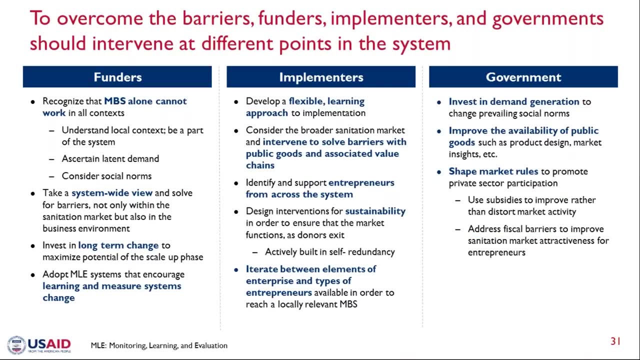 systemic parameters we talked about to not only lead to a higher coverage, but to create a sustainable, vibrant sanitation market. With this we come to the end of our presentation. If you have any questions, please feel free to ask them in the Q&A. 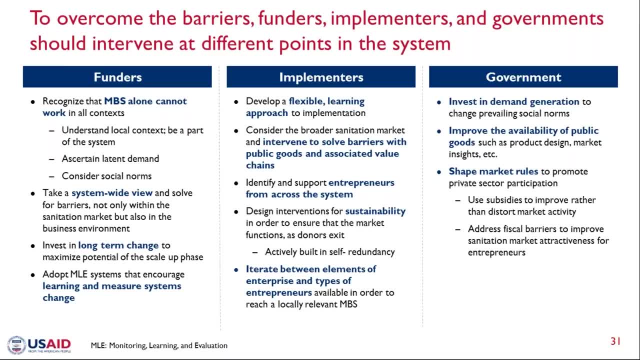 Thank you. And now we move on to the recommendations for each set of players that are involved in an MBS intervention. For funders, we recommend that they see MBS as one of the approaches to address the sanitation challenge, one of the key approaches which they can determine. 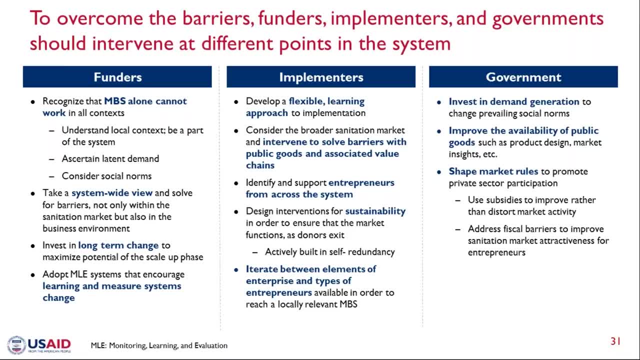 when to use, based on context, status of latent demand and social norms. Take a system-wide view and solve for barriers not only within the sanitation market, but also in the business environment And, most importantly, invest in long-term change, both by staying invested. 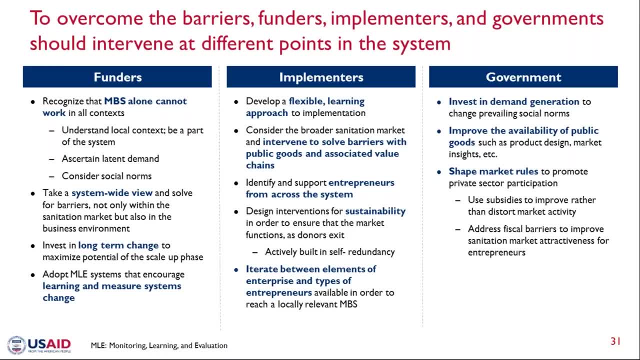 over a longer period than typical programming cycles and by measuring system change. For implementers, we would recommend, first and foremost, actively building self-redundancy to develop sustainable markets. Not thinking about it early on creates a situation where, as soon as the implementer leaves the markets crash. 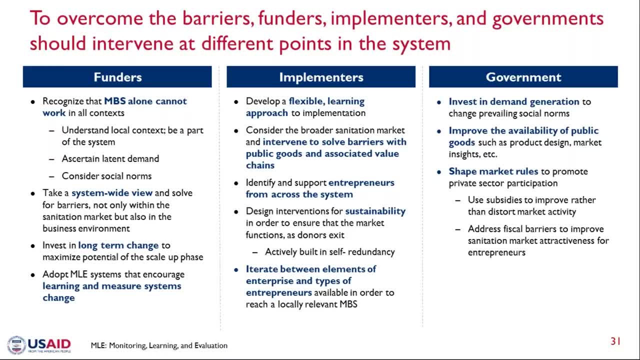 Follow an adaptive management approach to intervention and in identifying and supporting entrepreneurs from across the system. Lastly, solve for barriers around public goods to the extent possible. Governments, on the other hand, can play a significant role by investing in demand generation and creation of public goods. They can also shape market rules. so 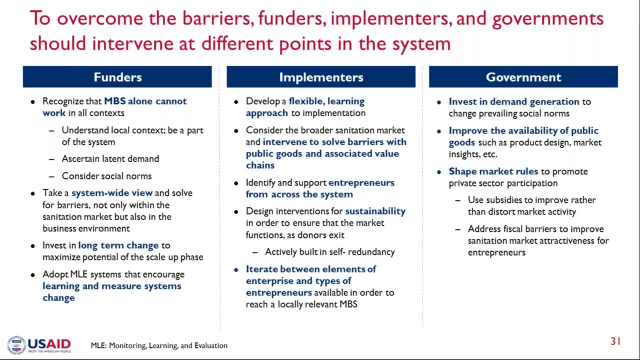 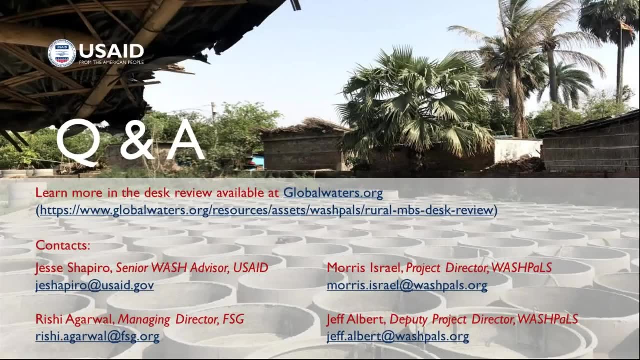 as to encourage private sector participation in the sanitation market. So at this stage I'll stop my monologue and we would be happy to take questions. Thank you very much. Okay, Thank you very much, Peter. Absolutely thank you. 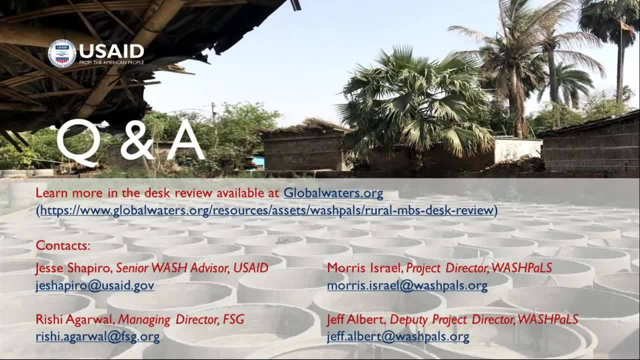 Thank you. is there everyone? Yes, there's a cell here. Okay, Thank you very much. Thank you, Rishi. this is Morris Israel. I'm the project director for wash pals and I'll be moderating the discussion based on the questions that have been submitted. 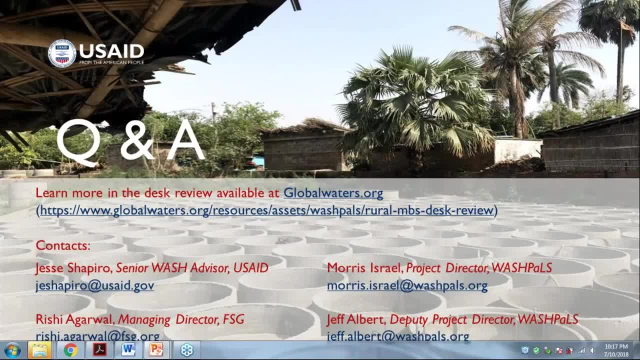 and as panelists for to address these questions, we have Rishi and Subhash Tanuri from SMG, FSG, as well as Jesse Shapiro from USAID. so we did receive a handful of questions during the presentation and I see that others are coming in as as we kick off the the question and answer, we have about 45. 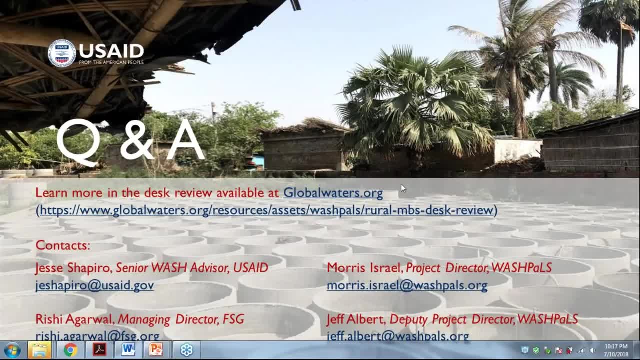 minutes set aside for the Q&A, so we should have plenty of time to address the questions. Rishi, for you an initial question: clarification and definition. really, one question asked for the definition of toilets that we are talking about and the definition of toilets that we are using in this study, and what components of that toilet do we include? 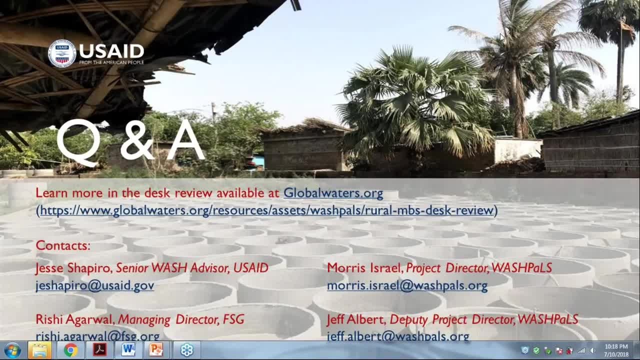 substructure, slab superstructure. so could you address that for us to clarify? so the way we looked at it was at least a superstructure plus an interface could include superstructure as well, but we were looking at a minimum of substructure plus an interface. okay, thank you. and then also by way of: 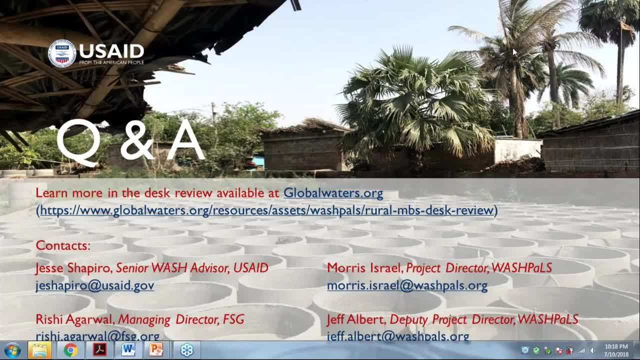 I guess, definition and understanding the focus of the study. we have a question that regards scale and the comment and anticipate that all attendees and participants can have seen the questions, trying to group those together. but the comment with regards to scaling is that there is in most countries a 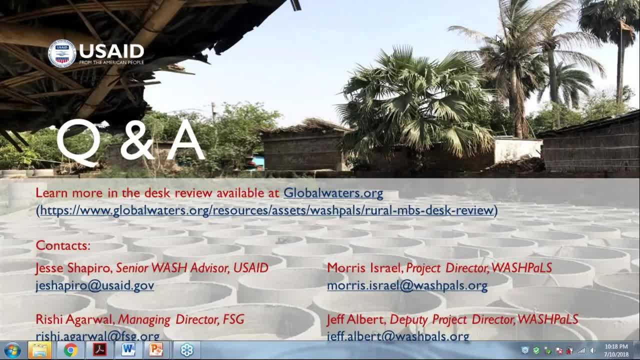 fairly vibrant, lucrative market for sanitation products at the higher quintiles for obviously for people that have reduced barriers in terms of the affordability and liquidity and whatnot, but that those challenges to scale increased tremendously as we address the bottom quintiles. and so the question was: was the study focused on this lower segment of the population, mostly in the 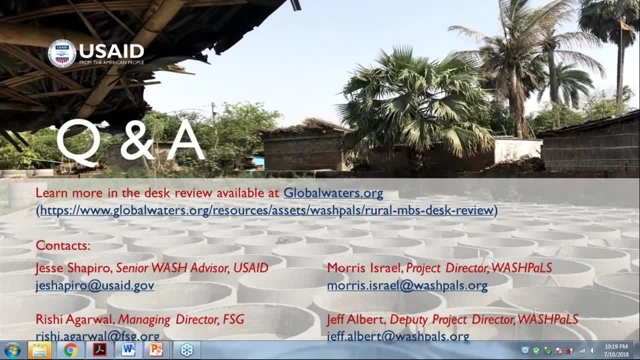 rural areas or was it looking at the sanitation market broadly across quintiles? that's a great question. so we were focused largely on the bottom of the pyramids and primarily on the rural populations. so if you look at all the interventions that we have covered- ID in Cambodia, watershed in 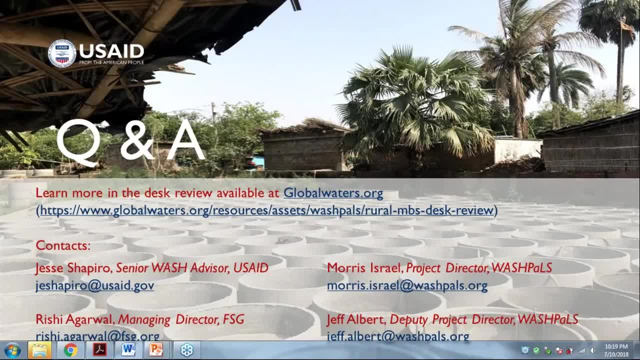 Cambodia, PSI in Bihar, water in Nigeria, Choba. all of them were predominantly targeting bottom of the pyramid, rural populations. I guess Peru was the only exception, but they're also. they were targeting bottom 40% of the population. okay, thanks and thank you, Rishi. we've had a few comments, questions that speak. 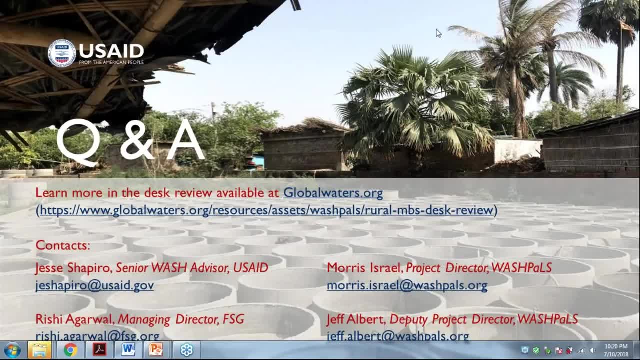 to the issue of subsidies and I was wondering, Rishi, if if you might be able to take a first stab at this and then understand. other panelists also would like to to touch on it, but the the few questions that we have on this one is: how do we manage the impact of subsidies in in a market based approach and then 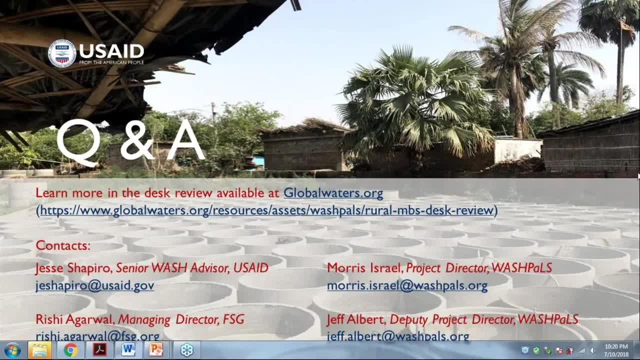 also, how do subsidies impact the effectiveness of a market, of a sanitation market? sure, and as he said, I will start off on this, but I would definitely want to invite panelists on to contribute on this one. so two things: aid subsidies in itself are not bad. yes, untargeted subsidies which create expectations of continued 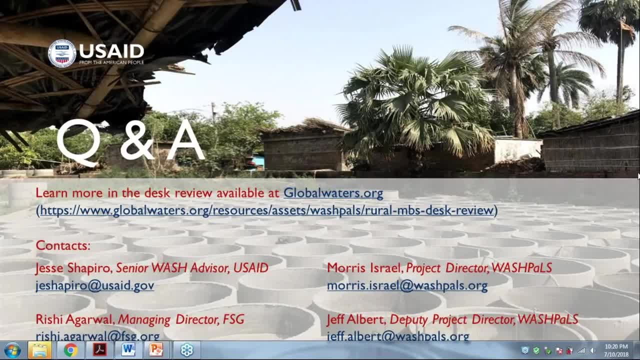 provision by the government is what really impacts the market. so if I go into a village and give subsidy to five people without any context, without any linkage to the markets and creating an expectation now that everybody is going to get some space at one time, so if a 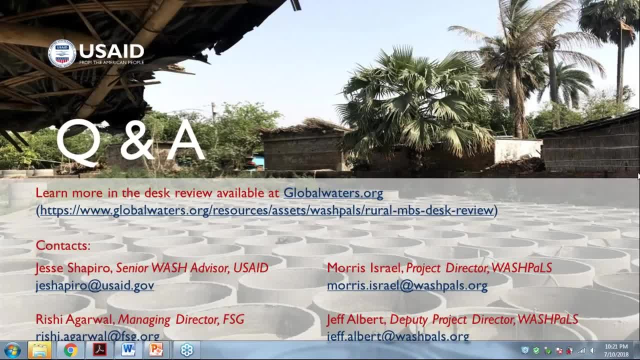 market player actually goes and tries to sell in that village. it's not gonna happen. so that's how we what we are calling distorting the market. however, if I provided vouchers through a lottery system- and that was also to be- was being given to the poorest, for example. 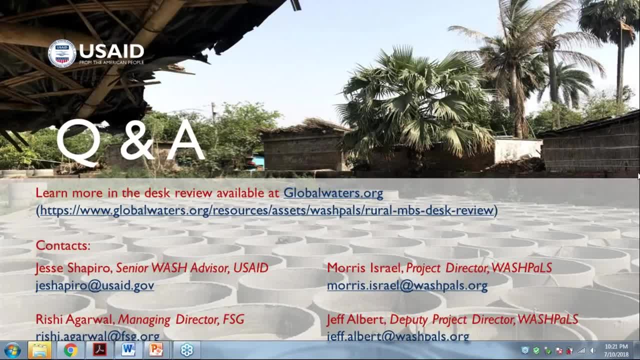 and then- and the provision still happens through the market- that is not really creating that much of a friction with the markets themselves. so that is what I would say could be a targeted or. Cambodia Choa is a good example where ID çok was used to target the subsidies and I know Jeff might have an. 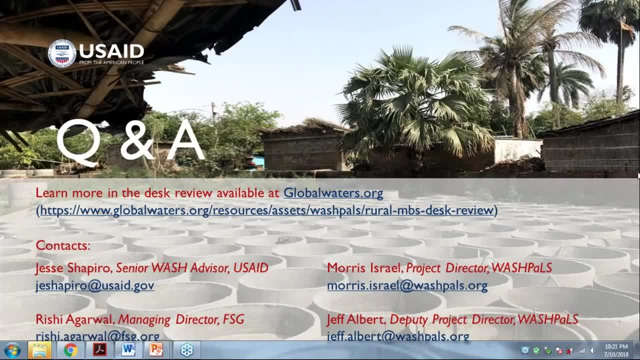 interesting point of view there, so, and I'll stop and let the other panelists contribute on this one. okay, thank you, Jeff. did you wanna? yeah, yeah, sure I'd be. I'd be happy to contribute here. It's interesting. Our poll results reflect, I think, a recognition among the community of the primacy of affordability. 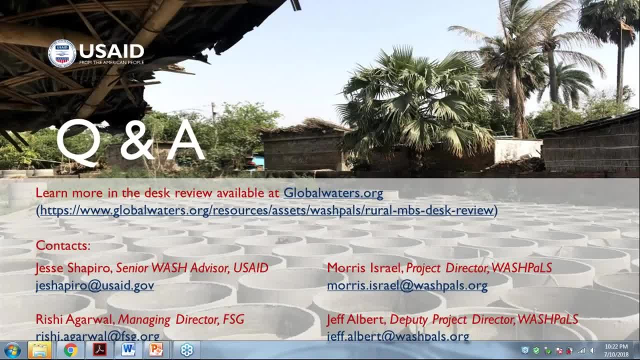 constraints, as well as, obviously, liquidity constraints, on the success of these programs. I guess we included demand as well in that option, But certainly it's recognized as a major issue. I should mention that the WashPals program is going to be actively examining the ability. 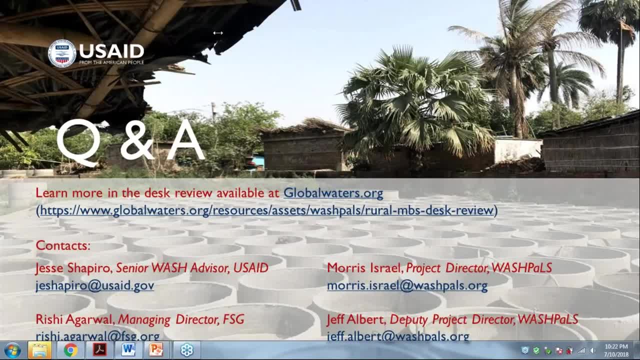 of subsidy to impact the sustainability of CLTS programs. There's no immediate plan to examine subsidy and MBS approaches, But the There's certainly this emerging suggestive evidence that subsidies can be managed in a way that doesn't distort markets to the point that it constrains outcomes. 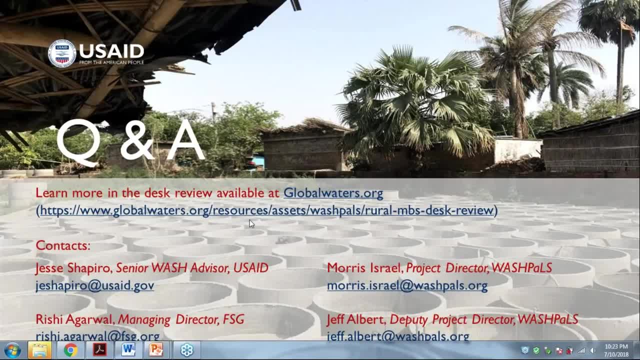 I see Yi Wei from IDE is among the participants here, and IDE has recently been examining deploying a targeted subsidy in Cambodia. Would you let us know what you think of that? You know the first thing: we are a big, big-time fan of the idea of getting some sort of significant 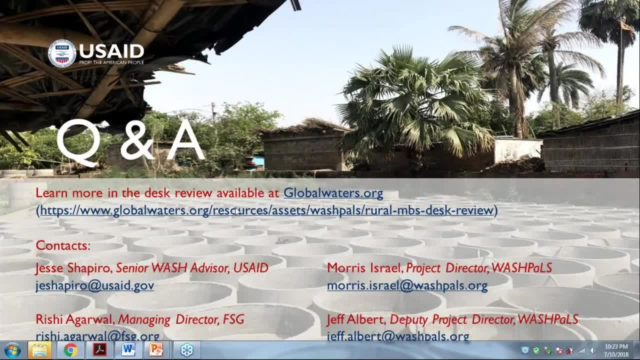 increase in subsidy recovery. That's different from, I guess, what you had mentioned earlier about the deal that we had with the. Yeah, There's a large number of areas that need to be done. I think, for example, we have on the left here the устройment. 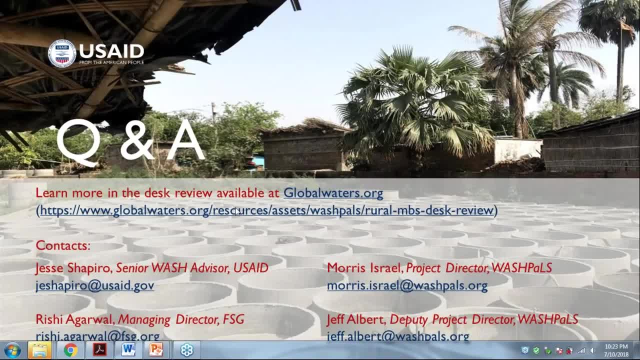 We have all of these inputs, We have all of these. We also have the old ones. We have the old ones, And that you know that all subsidies are not alike And the subsidies that I think many in the sector think of, or the interventions that they think of when they hear about subsidy, are full government, full provision of the asset, including both the substructure and superstructure, without much input or investment by the customer. 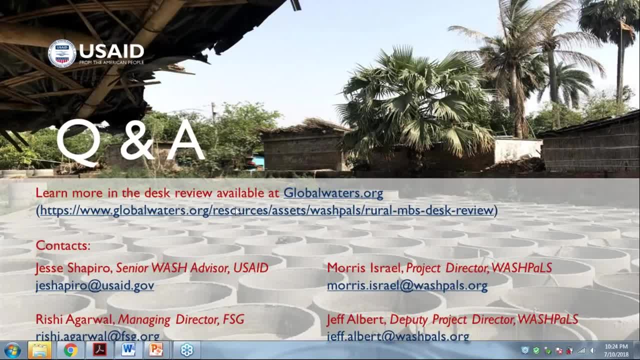 And the targeted subsidies that have been examined, you know, recently, are of a very different character and still require investment by the consumers and are generally again targeted at a subset of the population. And this encouraging population And the positive spillover whereby those households that aren't eligible for subsidy increase their purchases of toilets is something really encouraging and worthy of follow-up. 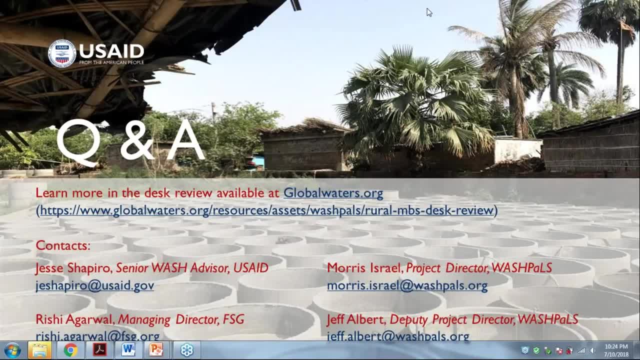 Okay, thank you, Jeff and Rishi, for that. I'm sure there's plenty of other thoughts about subsidies and I believe there's. we'll see some additional questions or comments coming in on that. Jeff, you did mention that WashPals, as a project, is undertaking a subsidy study. 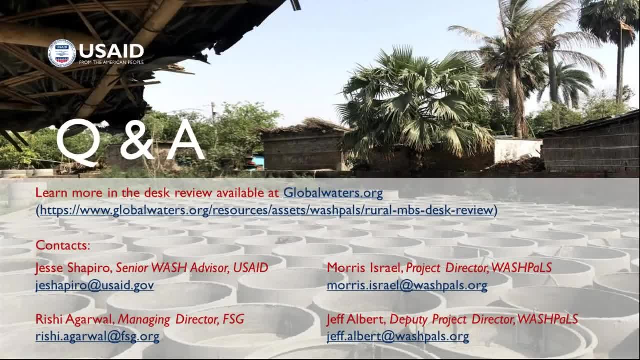 And there are two questions that are coming in I think relate a little bit more to what the next steps for the project are And Rishi, perhaps, or Subhash, you can address. There's one that asks, of the barriers identified and discussed in the presentation, which were the more significant. 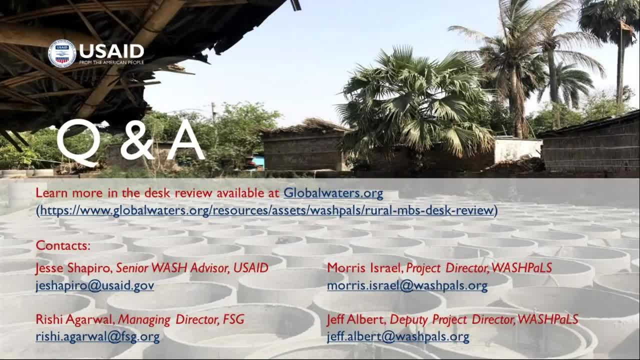 Were we able to identify through our research which of the barriers might be more significant? And then, building on that is, which of those evidence gaps are we anticipating going forward? Are we anticipating to fill as a project? Where's our research going And where would we see room for others to contribute to help fill those evidence gaps? 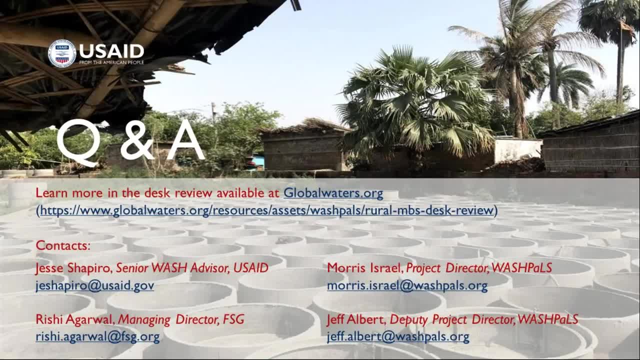 Sure, Thanks, Morris. So let me answer the first one and Subhash can probably do the second one. So in our research, what we have found is that there isn't a single most important barrier Right, And that's why this multi-layered, multifaceted framework, for which we're saying, you know, we're not going to be able to do it, 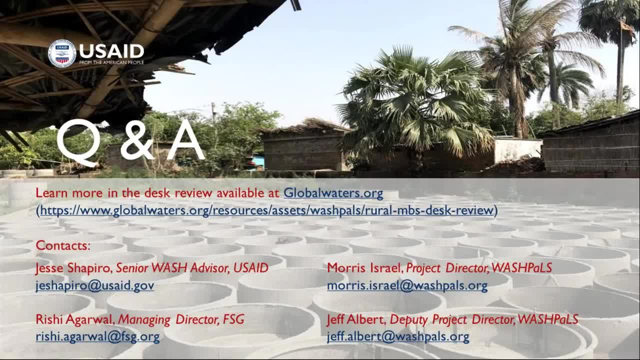 It depends very much on context. So let me take the 3SI Bihar example. The time you went in, we went in 2012.. At that time, the biggest barrier was an appropriate product system and liquidity. So those were the two biggest barriers. 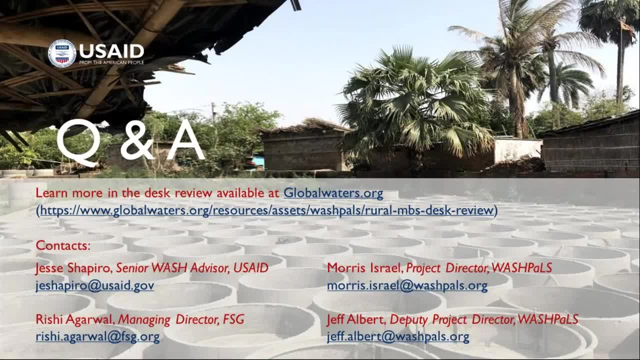 The rest was fine, Right. At the same time, if you look at go back to Watergate Nigeria, then availability of entrepreneurs itself was a significant barrier. So I think it's very, very context-dependent. And not just is this context-dependent, it's also temporal in nature. 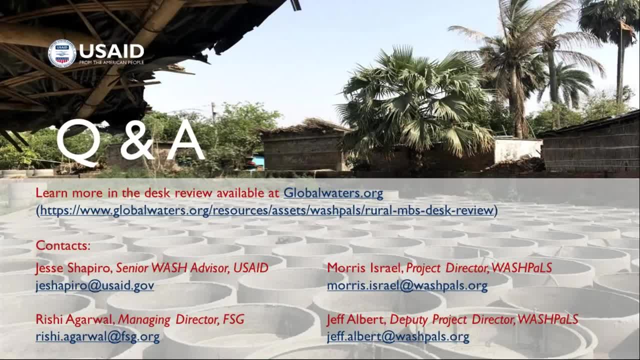 So as you solve for one barrier, the other barriers will become your bottleneck. So it's a constant vigilance exercise to sort of say: which are the barriers I'm solving for? What are the barriers are popping up And using this framework as a radar map of saying where these problems might pop up and what do I need to solve for. 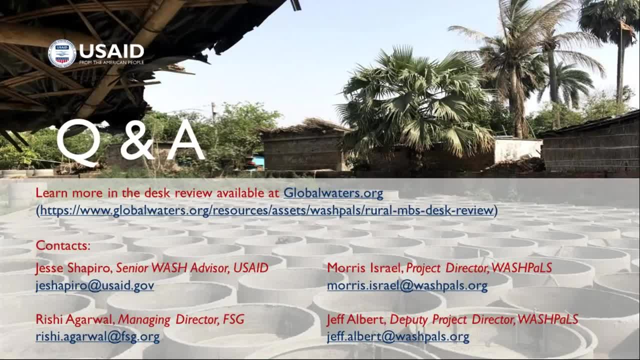 Is what we are hoping, is what the programs would do? I don't think, because I don't think there is one common problem that exists everywhere. Apart from saying affordability for the poorest of the poor is a barrier for sure, Subhash, you want to address what we hear. 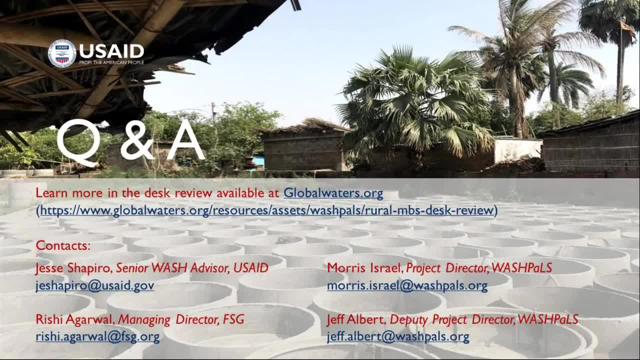 Yeah, Thanks, Rishi. And in terms of what areas we're currently investigating. as washpals, we prioritized studying the question about how do you make sanitation enterprises viable. Our research showed that there were some interesting practices that were coming up in terms of what entrepreneurs were doing. 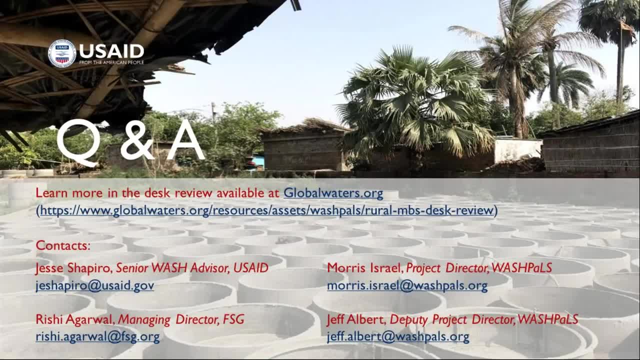 Some indicators as to what kind of profiles might be more suitable to run sanitation enterprises. However, we didn't actually get enough evidence in this space, And what we're currently doing is looking at entrepreneurs in three different countries to precisely identify these factors that influence or impact the viability of enterprises. 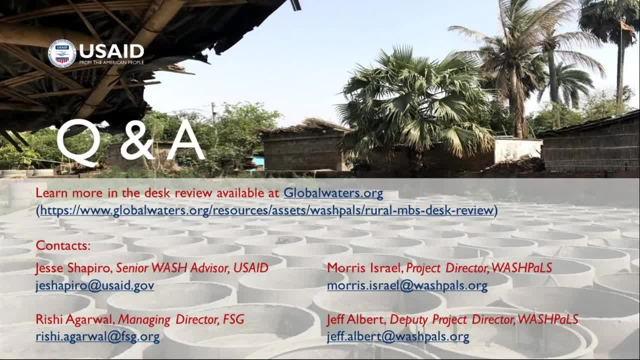 And moving on to the second evidence gap is around market rules. While our research showed that market rules can play a major role in supporting sanitation markets, there was very little evidence in terms of what kind of rules were implemented. what benefits did they result in? 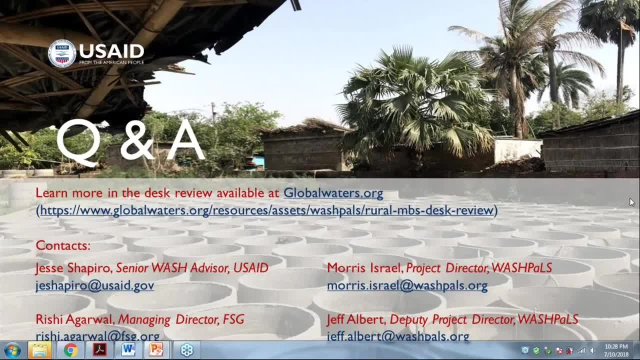 or, for that matter, what are the costs that are entailed in that? And with that lens in mind, we are looking at three types of market rules. One is to support: what kind of support do entrepreneurs require? The second is: how do penalties impact the uptake of sanitation products in the market? 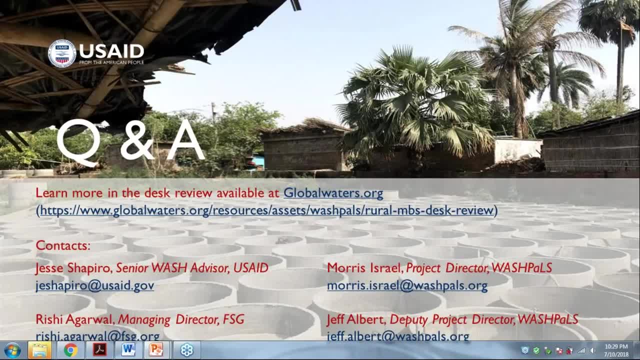 And the third is: what specific role do fiscal mechanisms like tariffs and taxes on the raw materials create impact on the viability of the sanitation enterprise? Thank you, And perhaps Sufash. building on that, there is a question about what we found regarding the sustainability of the private sector entrepreneurs. 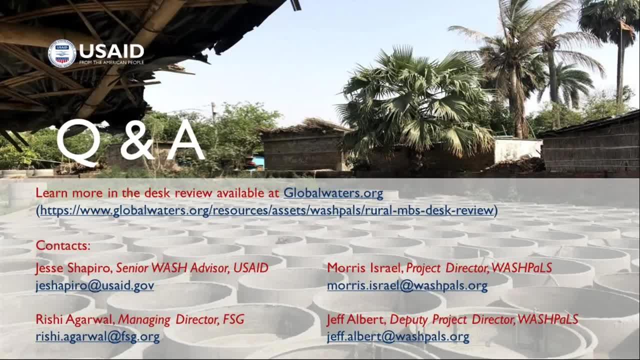 after the NGO or after the funder has departed the market, And perhaps that links a little bit to the discussion you just had about understanding the viability of the entrepreneurs, But would you have some observations on the longer-term sustainability? So two things. 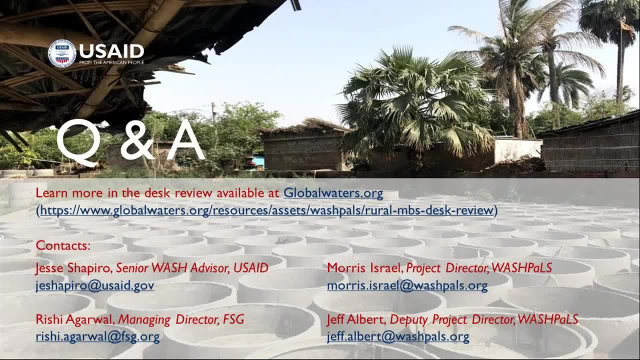 A. that is one of the key questions we are trying to address in the next phase But, at the same time, looking at some of the examples, what we have seen, and it comes back to our recommendation of actively building self-referencing for the implementers. 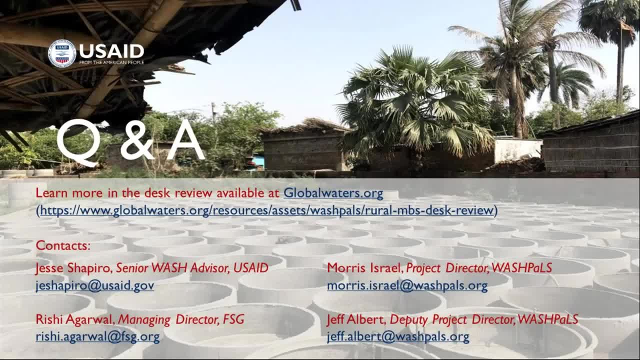 is where implementers become a player themselves rather than a facilitator. In those situations, they have to stay on for the markets to be vibrant. In other places, where they have tried to extract themselves out, the markets have stopped working, And that's what we have seen in terms of where they, for example, 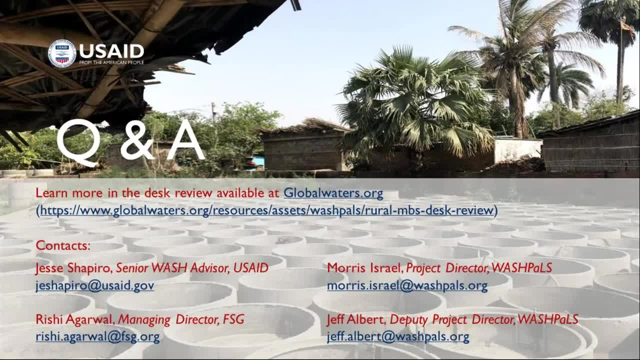 ended up paying the field sales agents' fees while not being in the market for the longer horizon. Those are places where the cracks are emerging now, So I think it's about how you design That decides whether these will sustain beyond the program tenure or not. 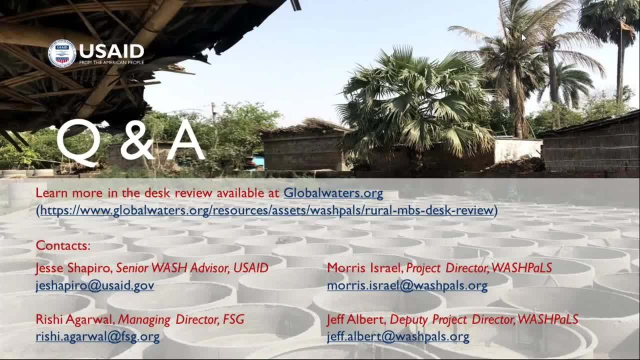 And a follow-up to that, Rishi. another question poses again the challenge of sustainability to these enterprises, as in a market we begin to reach, perhaps, points of saturation. Specifically, coverage is around 70%, And so the challenge of hitting those last few. 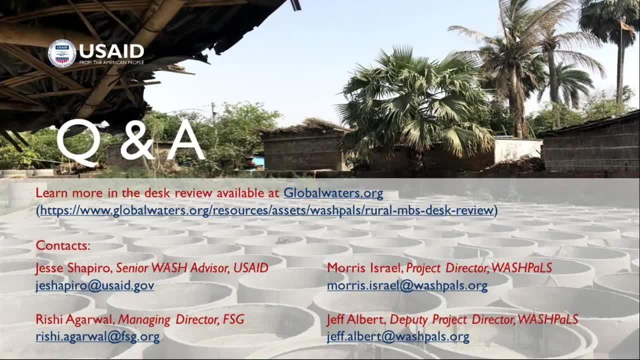 that last 30% of the market presents unique challenges to enterprises. What can be done in those contexts, and how might we begin to address that In the design of the interventions? Sure, So two things. A- the poorest of the poor. the problem will always remain affordability. And there would be a section of population in every country where land rights would be an issue, where the available space would be an issue, where those things are something that markets will never be able to target. At the same time, would the viability be okay? 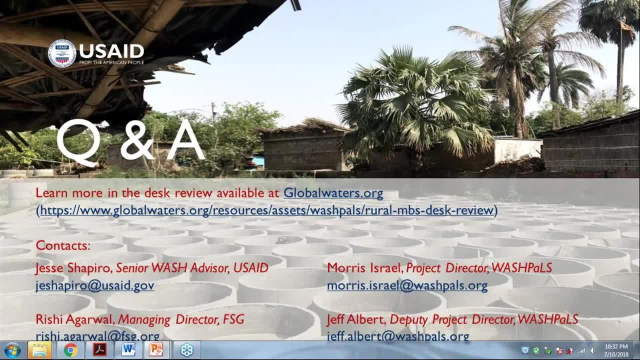 and sustainability be okay for sanitation enterprises, And I think that would be a big challenge. I think that's something that we need to look at And if we're going to look at the future of sanitation enterprises, we need to look at the future of sanitation enterprises. as we start hitting 70% coverage. I think even if we hit saturation, there would be a phase of consolidation. But as with every other sanitation market, let's look at US. we still have thriving sanitation enterprises with near 100% coverage. So I think that would always be an option, because families would divide, There would be an intraday required, There would be a replacement demand. So that's viability of the enterprise of the last 20%. I think that's where we need to figure out. 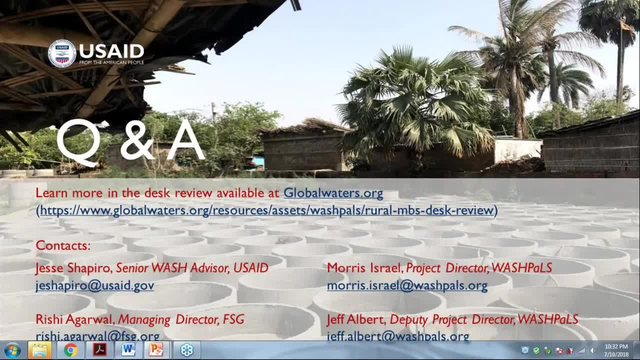 the affordability part of the equation. Okay, thank you. We have, Rishi, one question specific to the interventions that you mentioned in Nigeria about installment payments, And the question was: what impact does the payment and installments have on the sanitation market? 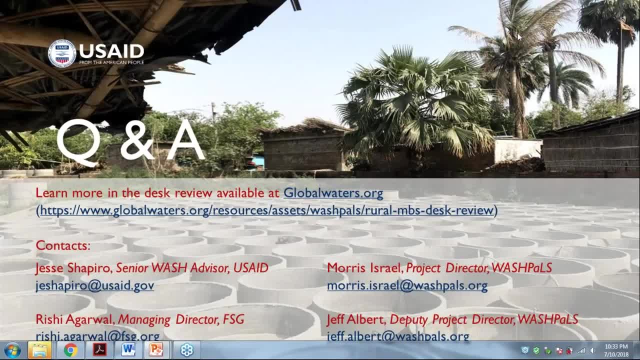 This is Sivash. Thank you, That's actually a great question. So I think there have been numerous formative research focusing customers that actually show that they will be more receptive or receptive to actually purchasing toilets, because it goes to addressing the issue of liquidity. 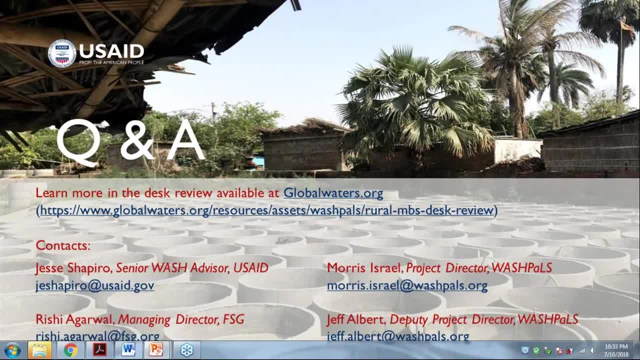 that we had highlighted in the framework. However, on the other side, which is the sanitation enterprise, the evidence around what impact does that have on the viability of the enterprise is actually not clear as yet, And primarily because it depends on context And it's entrepreneurs may be reluctant to take on a risk. 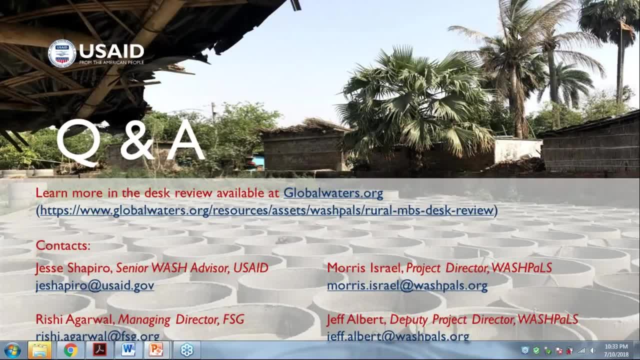 of excessive bad debts or the added complexity of following up with customers and ensuring recollections. And I do mention context because there is a cultural layer in markets, not specifically on sanitation. If the norm is that customers can borrow, businesses do extend credit to customers. 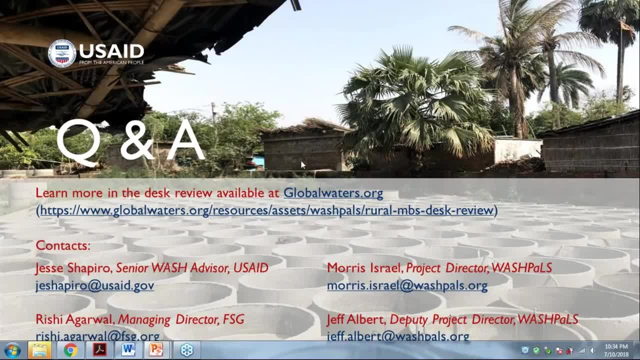 then there might be more scope for using this mechanism to improve sales. So, as I said, it boils down to context. Thank you, Okay, thank you. Next, we have a question on the role of product development, research and development, particularly for some of the more challenging geographies. 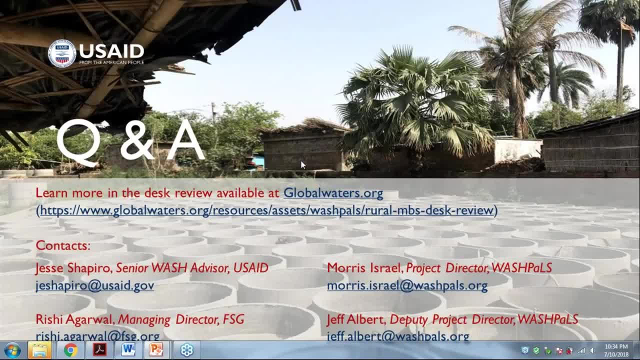 and market segments in areas where there's high water tables and the such? What information or what findings did we have from the literature review about the role of R&D and how to encourage and ensure that it happens? So I think I'm just sort of hearing the questions in two parts. 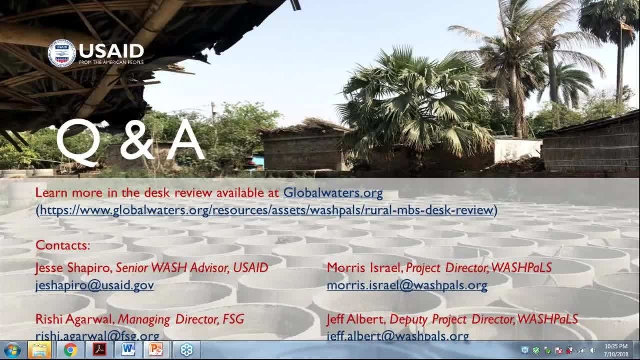 and please do let me know if I'm interpreting the question wrongly. A is product research and development for within the intervention is still required, still happens, and that's part of the public goods we were talking about. So, for example, there are more often than not price gaps in the market. What's available is either, you know, septic tank full-on $1,000 product or really cheap temporary $50 product which the customer doesn't really want. There normally isn't a middle-of-the-road product which is good enough. 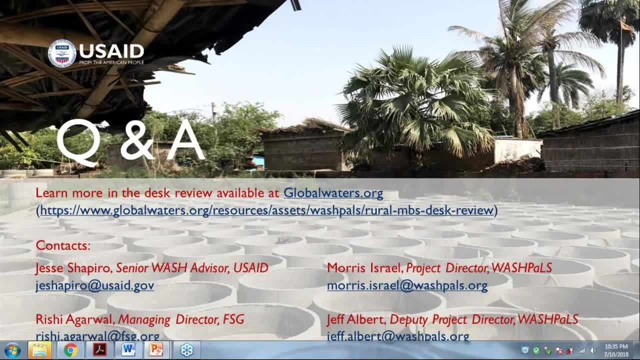 which provides all the benefits but might not cost as much. And there is always some product design work required to get to that product And that we believe is always part of an intervention, even though it sits in business environment, because for one enterprise, especially in the context we're talking about, 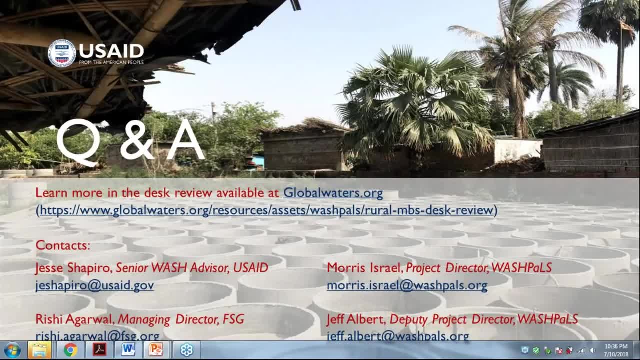 rural part of the pyramid markets. it's very difficult for one enterprise to do that research, So that's where the public goods come in. On a broader scale, if you're talking about hard-to-reach markets such as high water table you mentioned, 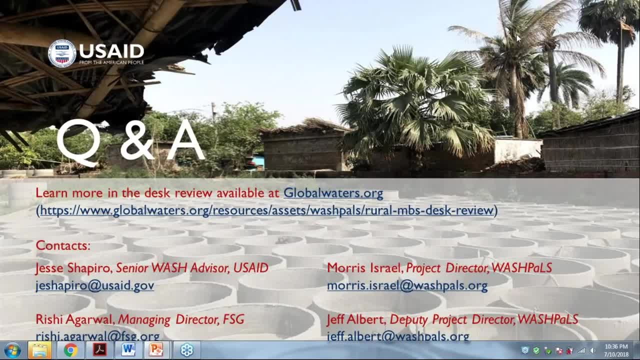 or, for example, really porous soil near the water banks. in those situations, we believe there's a separate, broader question and product design that needs to happen, maybe even outside the local ecosystem, which talks about looking at- is this a global issue and saying what can be done for product design. 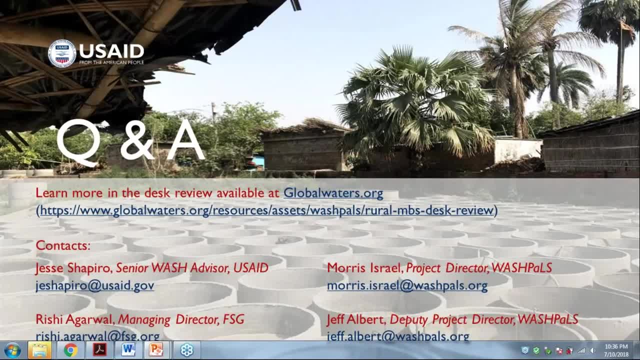 for high water tables globally. Okay, thank you, Subhash. there's a broad question asking about the role of women groups in the sanitation market. I know we've had conversations and we've done quite a bit of thinking about that. What would be your comments, reactions about the role of women groups? 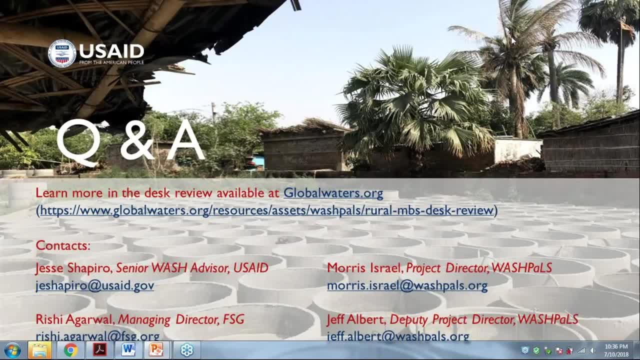 in promoting sanitation markets. Thanks, Morris. I think in certain contexts the role of women as a demand activator can, or rather I would just say women could be potentially more active, effective as demand activators where they themselves are able to tap into the networks of self-help groups. 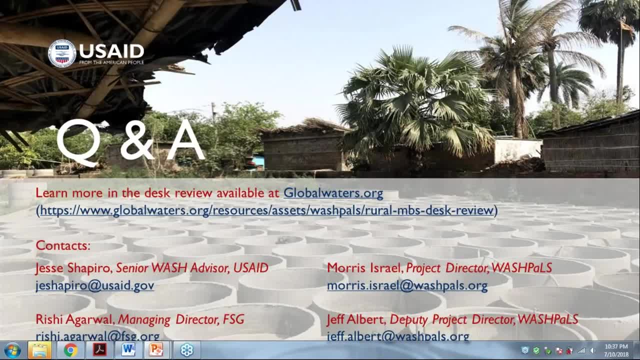 what they call- in India or, I think, under the geography, such as Vietnam. we've heard of the Vietnam's Women's Union, where they leverage those networks to be able to influence women in order to purchase a toilet There. the network effects could potentially play a role. 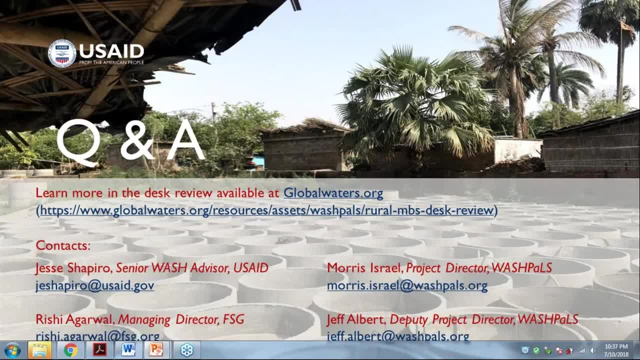 But what we haven't actually seen- explicit evidence as yet showing how the role of women in the sanitation enterprise value chain can impact both the viability of the enterprise, both in terms of increased sales or, for that matter, increased profits. Okay, thank you. 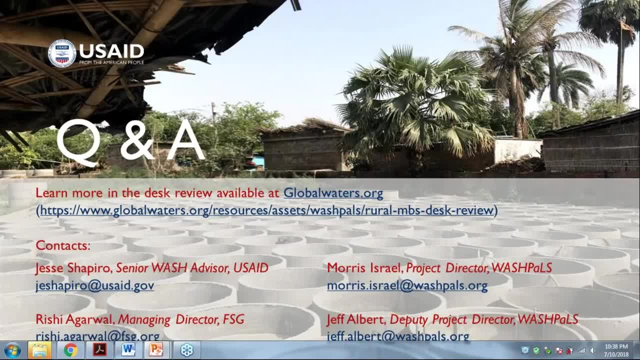 The other thing that I would note at this point is that WashPals does have a small grants program that is looking at innovations in behavior change related to sanitation, And one of the grants that we have currently underway with IDE is looking specifically at the role of women in the sanitation value chain. 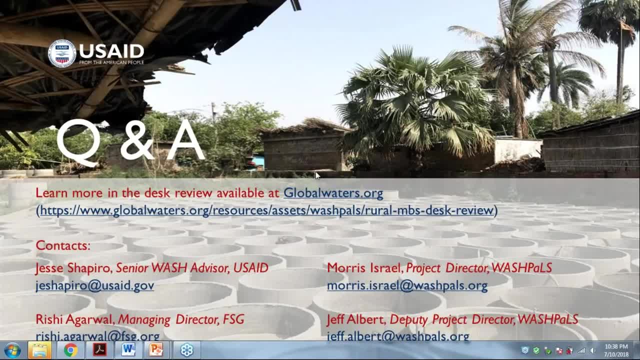 So that one is a few months in and looking at, as I said, the role of women in the value chain. So stay tuned for results and findings on that, as that might contribute to answer the question. Next question, one that just came in, relates to: while our literature review. 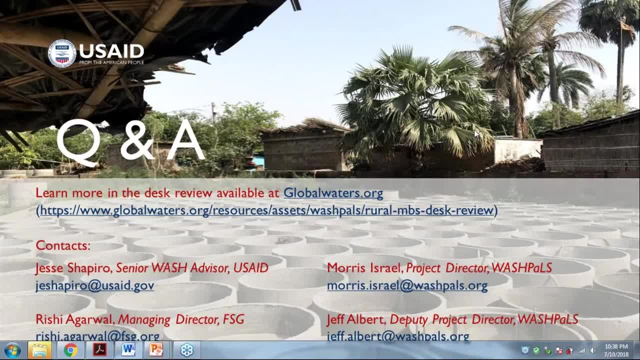 and the focus has been predominantly on rural areas. to what extent does the research, can it be transferred? is it applicable to informal settlements in urban areas where, again, the sanitation issues are challenging, to say the least, and that are subject to fairly rapid influx of populations? 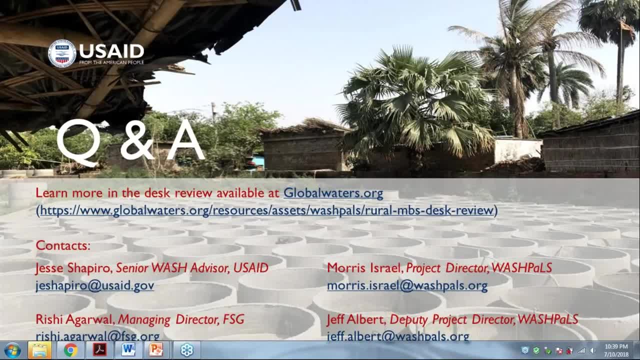 Are there lessons that we can take from this work and apply to those informal urban sectors? Yes, that's always an interesting challenge because there are two or three things which will change. So one of the barriers which is not in our framework, because we rarely see 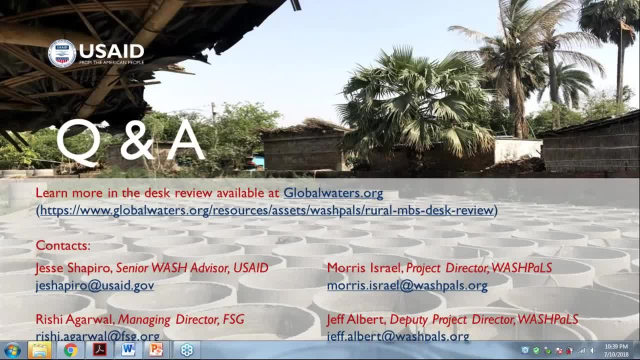 that in rural scenarios but is quite prevalent in informal settlements, is land rights. So we do see that becoming a major barrier for the willingness of a customer to invest in the toilet, Beyond affordability and liquidity. and that's what sort of would prevent latent demand from converting into actual purchase. 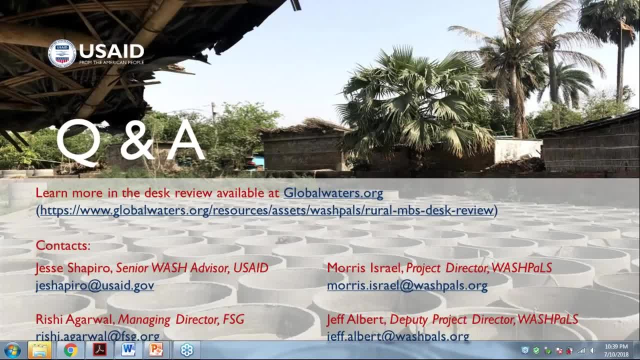 There's just a lack of land rights, because of which they won't invest in home improvement, they won't invest in building a toilet. The other is space which you would see in terms of spatial constraints, which, again, you won't see in rural environments, but you will see here. 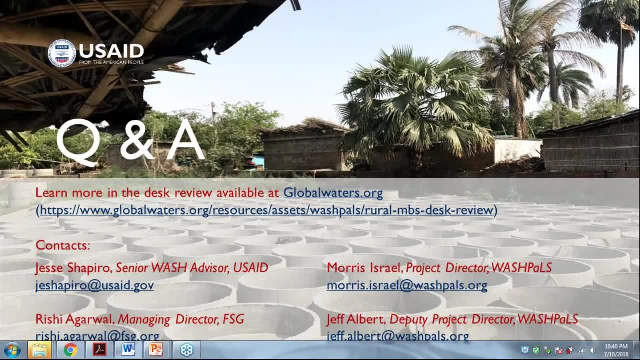 I think the other components remain the same. So it's essentially the customer barriers would change slightly because of the context we are talking about, Which would bring in A space and B land rights, which we don't see. I think the rest of them, the elements, would remain the same and can be. 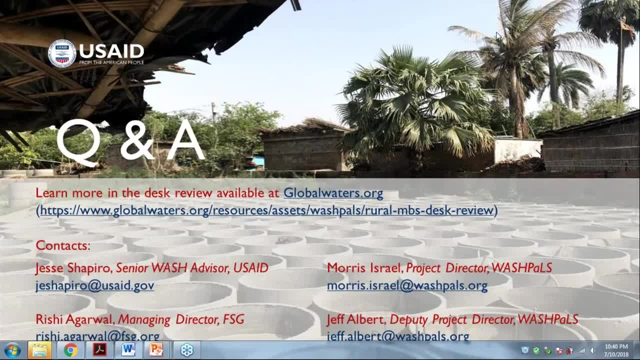 transferred over. Okay, thank you. Thank you, Rishi. One additional question that we have regards implementation of the programs and the interventions themselves, and specifically asking to what extent do endogenous factors, such as organizational structure or differences in management approach, Affect or impact the results of interventions as compared to some of the 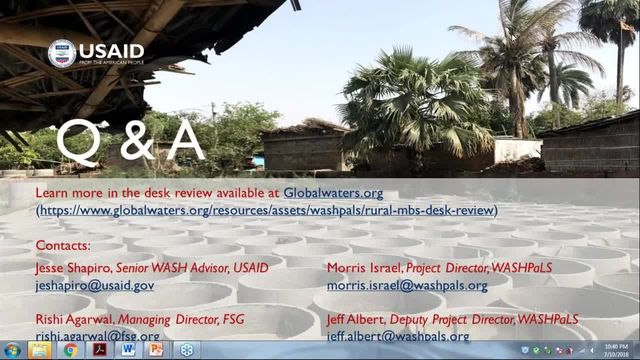 items in the framework, the business environment or the overall context. To what extent do management and organizational structural questions drive the intervention? Yeah, so to be honest, we did not review the organizational structures of interventions. I would like to inform this was a desk review. 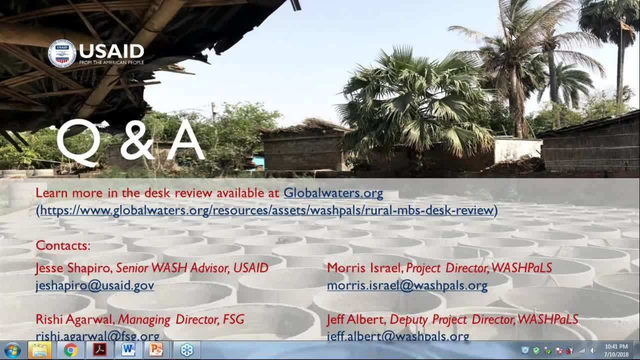 So we stayed with what was available publicly, without us going and interviewing people. in this phase, We did look at how different strategies impact and same organization, for example, have taken different strategies depending on different geographies. And that's where our- again, the actively building self-reliancy part comes in. 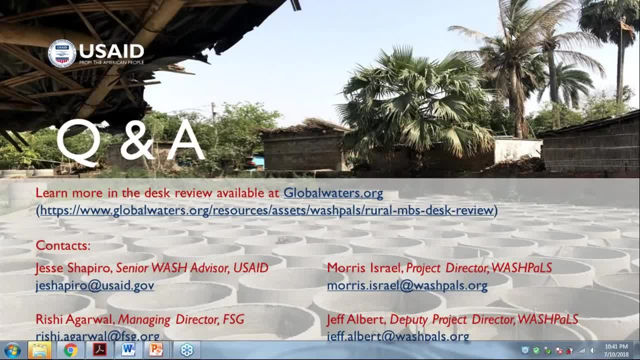 But we haven't really looked at endogenous factor. I think Jesse, as a funder, might have some thoughts. Thank you, Rishi. I'll just add: yeah, again, we didn't research these organizations, But one thing we could acknowledge is the ones we did research, they were all. 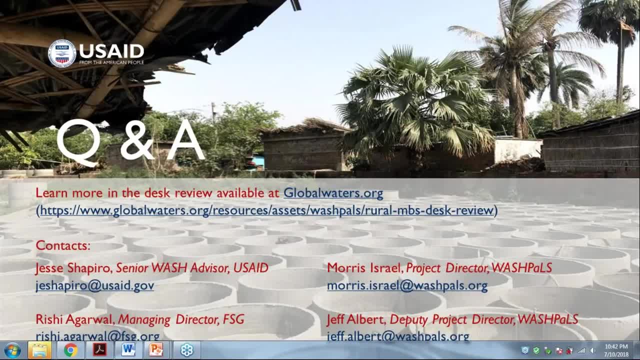 NGOs, and they were all funded by external finance, And so I think that's just something that our sector can recognize Globally, and there may be other approaches, methods, actors that we may want to be involved for this to be successful as well. 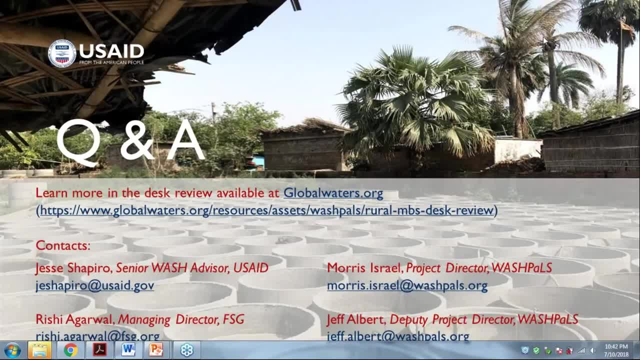 Okay, Thank you, Jesse. I don't see that we have any additional questions from attendees. I'm not sure if others that are moderating this draw my attention. anything that I might have missed. Morris, there was a question about R&D, I believe product R&D. 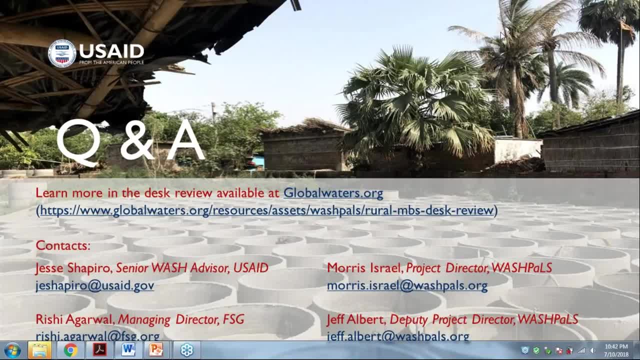 I think we discussed that. Was that covered, Okay, Yeah, Yeah, I think Rishi addressed that. So, from the participants, please remind me submit additional questions if we did overlook a question that came in. So we just got something on. 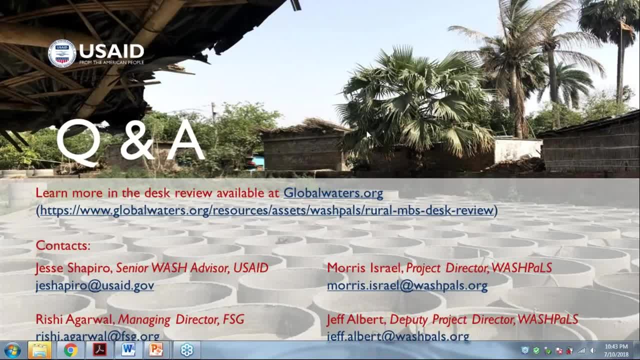 Hold on one moment. Yeah, So there's a question about implementing CLTS and market-based sanitation programs jointly, knowing that CLTS itself requires a fairly significant effort. So again, I think there's. when we look at the CLTS literature, there is talk of CLTS+. 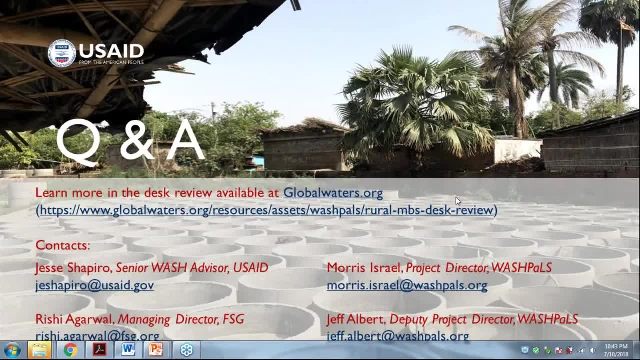 and that plus is often related to supporting local markets in some sense And, as Rishi indicated and talked about in the framework, while we're looking at MVS interventions, there's a significant role on demand generation and demand activation. So perhaps Rishi or Jeff, leading those two components of our work, there might be opportunities. 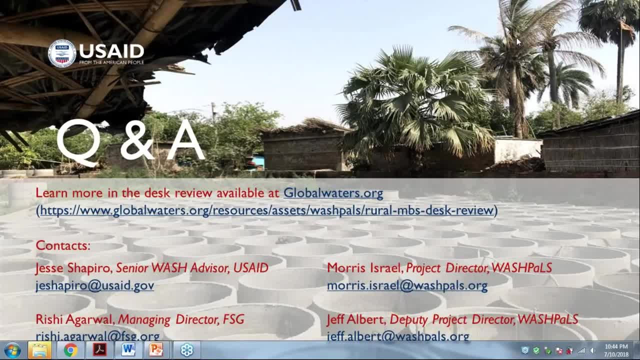 here to provide some insights on how we can better implement the two kinds of projects together. I'll let Jeff go first. Yeah, Sure, I mean, that's a great question And in particular, as we're, you know, as we think about not only the, you know the. 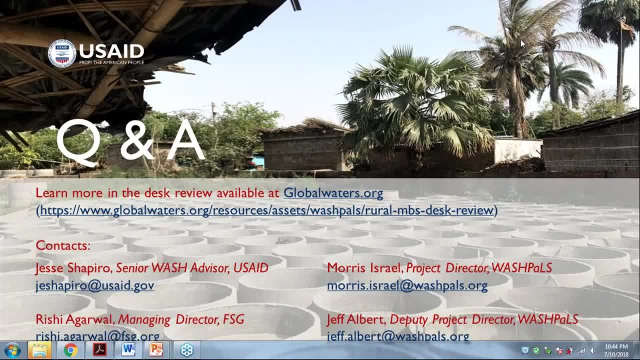 elimination of open defecation, but progression up the sanitation ladder. Mimi Jenkins, who's a researcher some of you may know, who's also involved in this project, is, you know- spells out the variables that drive purchases of toilets. 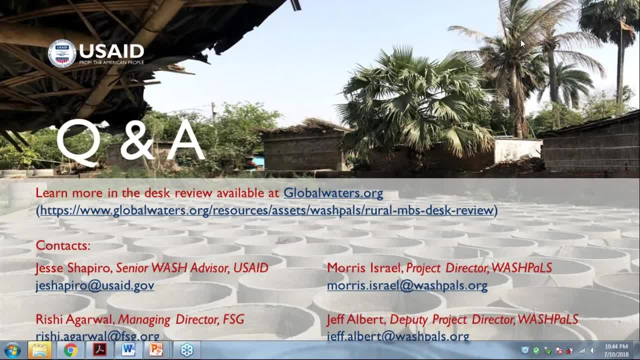 And she talks about motivation, which is obviously addressed by address, you know, by demand side approaches like CLTS, Opportunity And that's Driven by the availability of products by virtue of functioning supply chains and you know viable local suppliers. 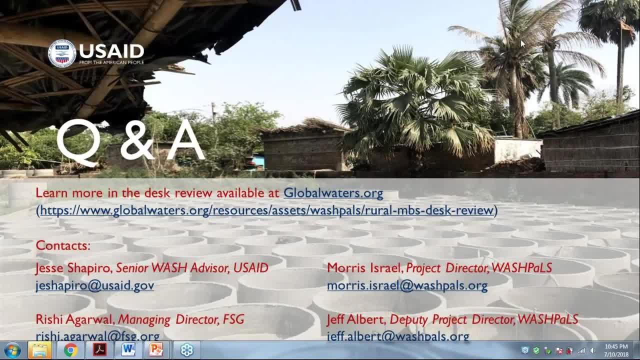 And then, of course, ability, And we've talked a bit about subsidy. But yeah, the interaction of the two is something that we clearly think about And I don't know that we have a consensus Sort of viewpoint coming out of this research project. 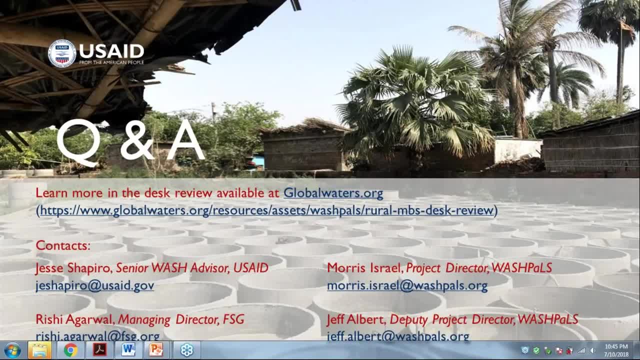 But this, yeah, I you know, an opinion that I'd offer personally is that this notion that CLTS alone can do the job to get us where we would like to get with the SDG, And now in SDG, in SDG, time is, yeah- has been discredited. 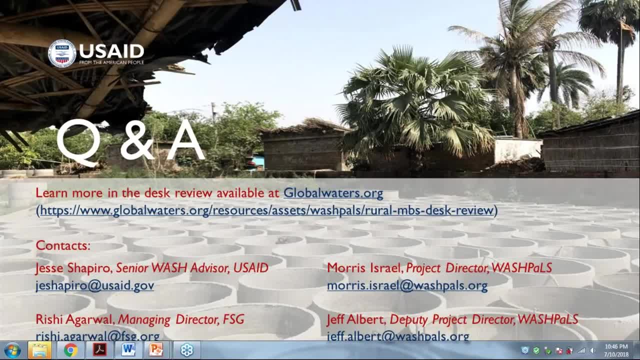 And that the As a sole, exclusive measure, And that the development of these markets is really essential. And so the you know, certainly within the CLTS community, there's this focus on collective action And that's And staying rather neutral on the promotion of given products. 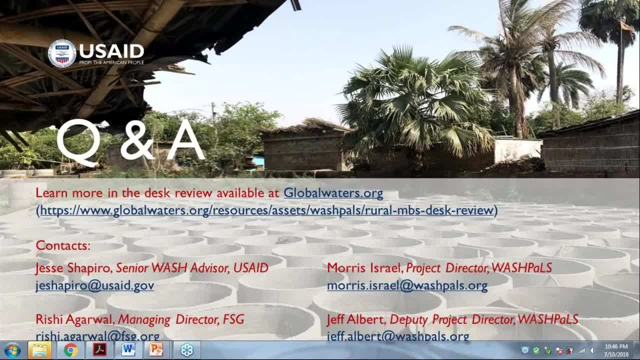 But yeah, certainly within this project that's something that we're seeking to test And certainly within our work on subsidies. there's no way to, There's no way to act on a subsidy if there's no existing market to basically meet the newly generated demand by a CLTS program. 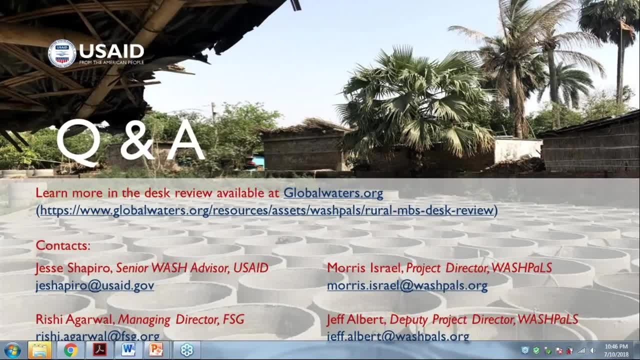 Rishi, Yeah, I mean saying of this same hymn sheet. The way we see it, I don't think a single approach, either market based or CLTS, is enough by itself to solve the challenge. We do think it's horses for courses. 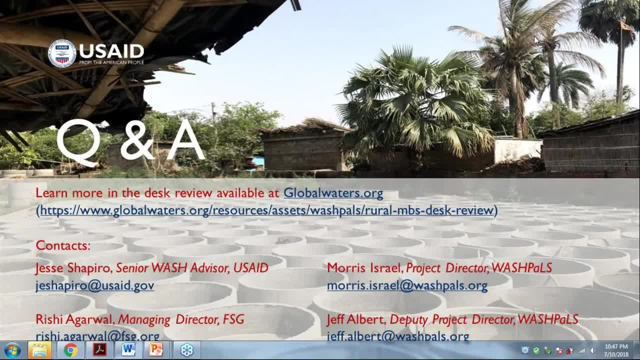 So, depending on the situation, depending on the population segment we're talking about, we should be leveraging both And, in some ways, one of the questions we haven't answered on the question which is open- And I saw John had a question in terms of what are the open questions that you would want other people to look at- 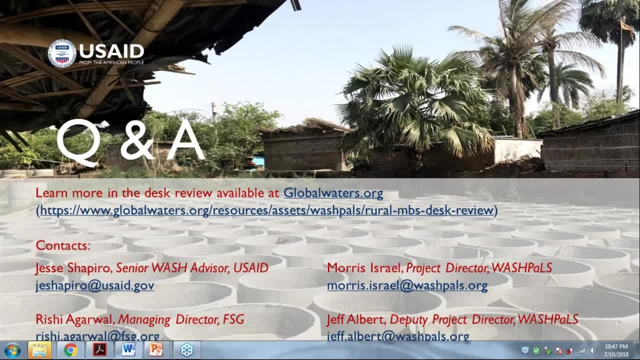 Is: Is there a sequencing? Should there be a sequencing? How do you actually put CLTS and MBS together, And that's something we are not looking at. That would be a great question for others to contribute. Just to add to that. I agree as well. 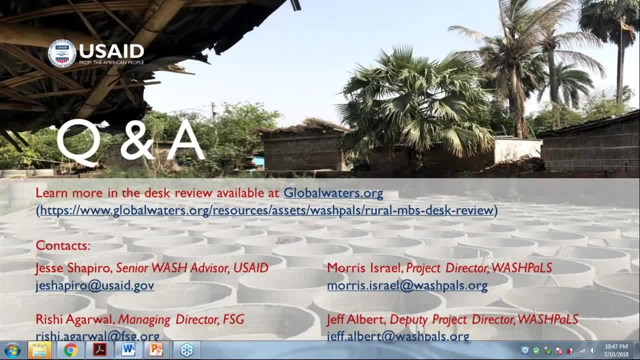 This is Jesse, I think. when looking at how do we drive sustainable sanitation at scale, I think the sector is coming to a consensus that In a lot of situations, CLTS works and a lot of situations, MBS works and a lot of situations both are required. 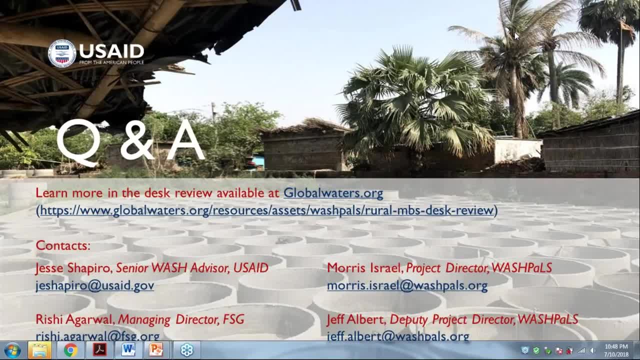 But again, building on what Rishi and Jeff said, those alone are also not sufficient. There will be other approaches and other activities required to enable the market and the entire population to reach sustainable sanitation, And really the question is just about sequencing, And I think there's been a lot of vibrant discussion in the sector over the last number of years about this question. 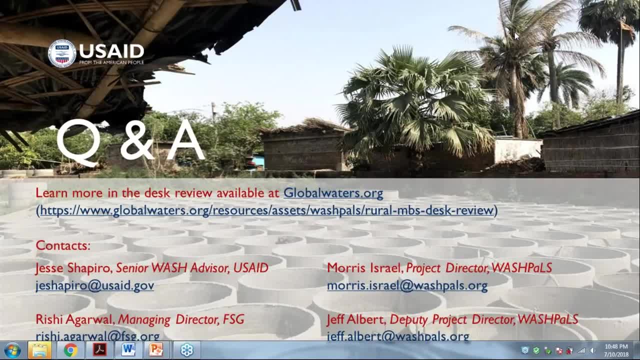 Some in the CLTS community say no CLTS first and some say MBS first, And I think what we've really seen from our study on CLTS is that, as Jeff said, CLTS alone is not going to be enough And that it seems that maybe a majority of situations the sequence would actually be some form of market needs to exist prior to the CLTS. 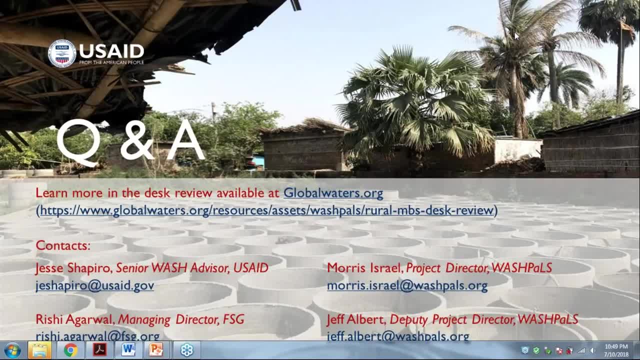 And then that needs to grow more robust over time If we really want to not just have effective programs that trigger the sanitation behavior but then sustain it and have facilities that can sustain that behavior over time. Thank you, But I think this is still a question to be answered, with no definitive action, definitive answer or consensus on the subject. 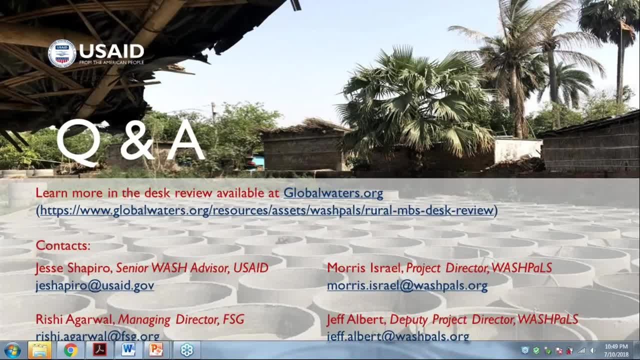 So I do see it as something that we can all explore going forward. There's lots of programs out there now trying to mix these two approaches as well as others. Okay, Thank you on that. One additional question just came in, Noting that in the desk review we're fairly silent on the role of the large private sector players: the international, the and the such. 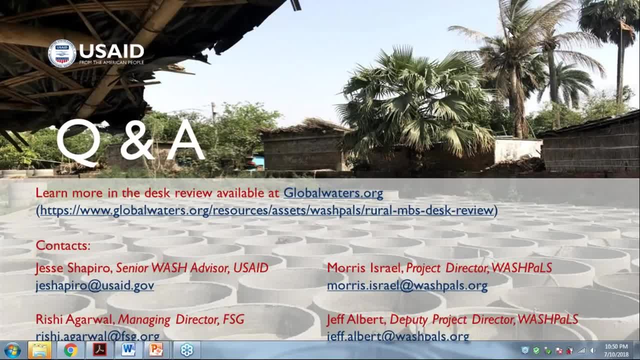 So I was wondering, Rishi, if you had any thoughts or observations on the role of those larger private sector firms in the sanitation markets that have been the focus of our work, largely rural focus, Sure, I mean the Peru Mi Banu example is one where we do highlight some of the larger players coming together. 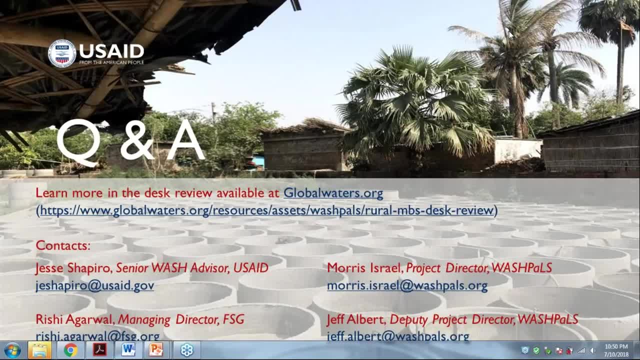 So that was an alliance of 12 players coming together to form a coalition to target the additional half a million households in the bottom 40% of the population that we were talking about. What we haven't covered is players likely to excel because they have been a product innovator. 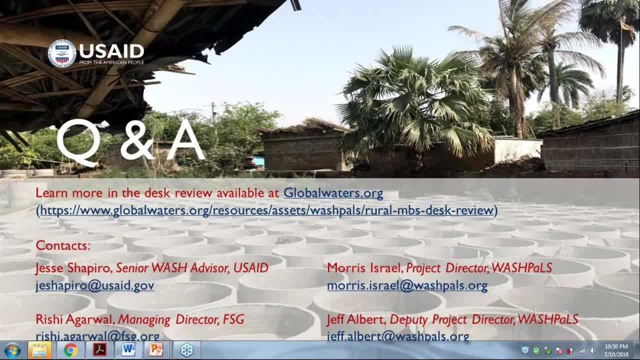 They have been more of a product innovator sitting outside these interventions. So one of the things we wanted to see was: how do these interventions get to scale? And they have been very, very focused on just one piece, which is interface. So that's why we haven't seen much on them in our report. 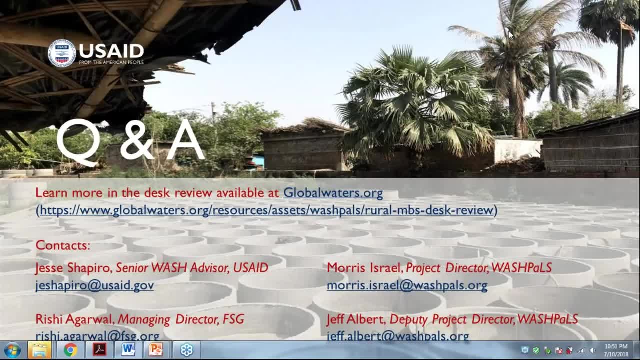 But how do large players contribute? One example we have picked up is the Mi Banu example, which was about large players coming together, including a large bank. Okay, Can I add something here? You'll notice that the first slide, or sort of the opening slide, of this presentation actually has images of Lixil's SATO pan. 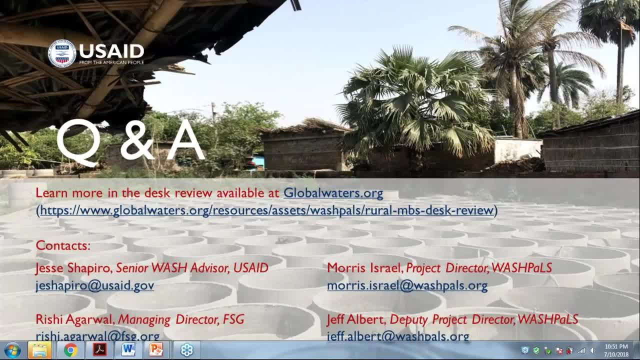 And it's certainly a test sort of business division. Okay, And it's certainly a test sort of business division within Lixil, which is currently a CSR activity, but which Rishi correct me if I'm wrong- is it a five-year? 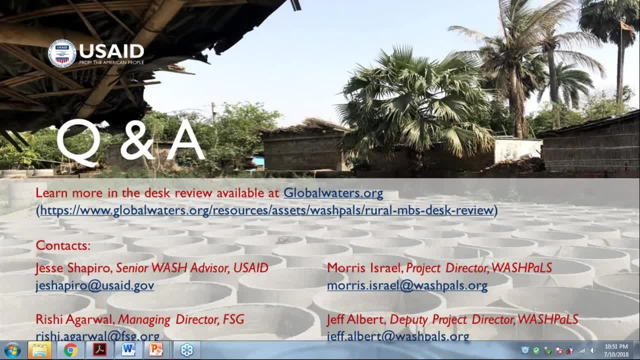 They basically have five years to turn it into a profitable division within the company, And they've. you know they're quite aggressive at this point. Yeah, they need to be self-sustaining. if not profitable, That's not it. 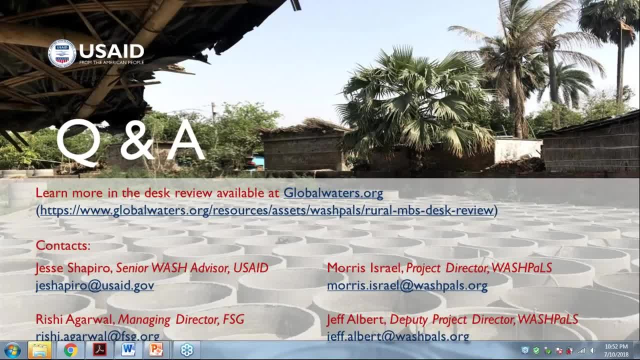 Within a five. I believe it was a five-year horizon, if I'm not mistaken. And yeah, we were at a meeting recently in which we saw a presentation from Lixil And they've reported pretty impressive sales in Tanzania over a fairly short time period. 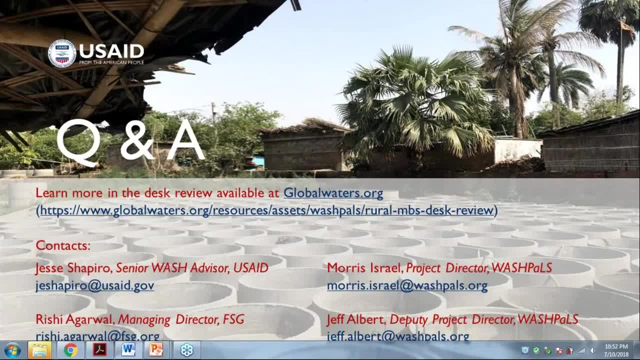 But again, yeah, as Rishi points out, the focus is very specifically on the interface here. Okay, thank you. Another question came in again on how we measure, how we rate the success of market-based sanitation interventions and whether there's been impact that made it a significant impact at a global scale. 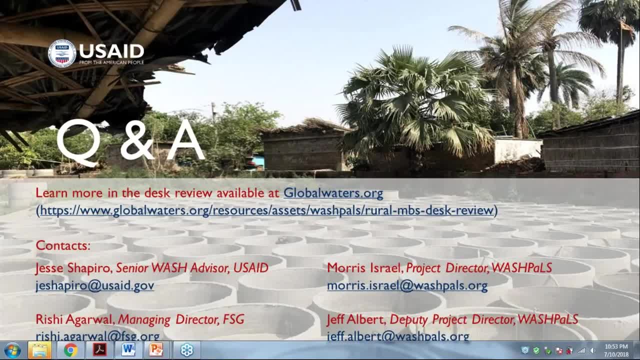 And this goes back a bit Rishi, to the early slides on how we define scale and how we would look to grow the intervention. So any thoughts on opinions on how we would rate the success of market-based sanitation? So I would say: green shoots, good early signs. 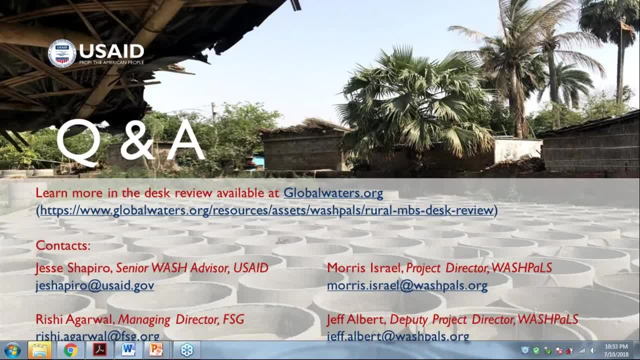 Part of the issue is also: it's not. it's very hard to measure what the real market change has been, because most programs tend to measure their own success rather than what might have been enabled in the market. Okay, So I think it's important to measure the success of the programs, but not directly due to them. 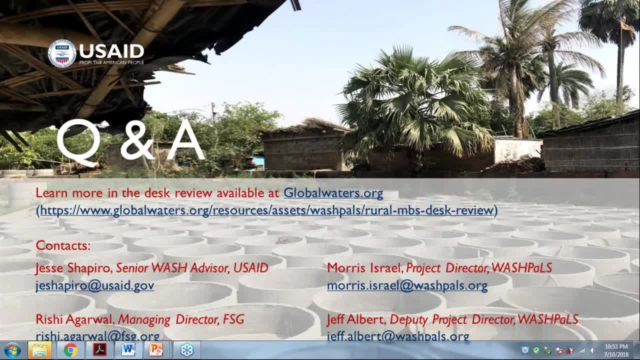 So there is a measurement question there as well, But to me it's early success. It's not something which has become a major force so far, but has the potential of the coming one. Okay, thank you. I'll ask our attendees if there's any additional questions or comments that they would like at this point. 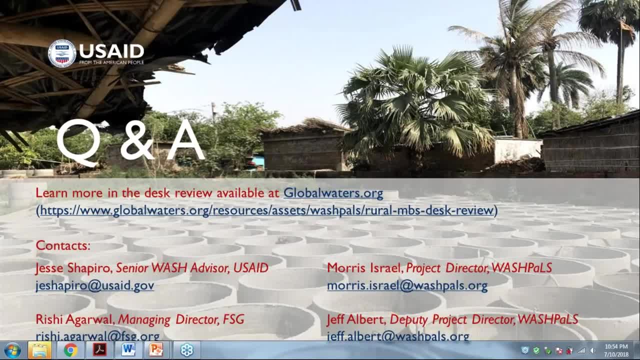 We still have some time, But for now it seems that we've addressed, I think, all the questions that have come in, And so one did come in about in the report. we mentioned that the need particularly Rishi. you just building on what you just said about monitoring, that we need to monitor differently. 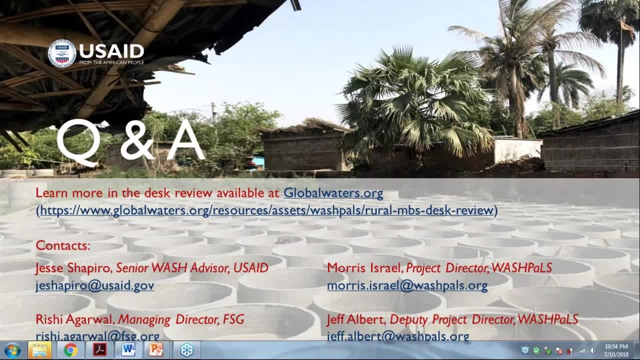 Are we exploring anything specifically from Along those lines on the monitoring? Yeah, So the key thing, John, I can see this is your question, but is moving away from just measuring. So you know, the process of measurement is baseline, a midline and an endline. 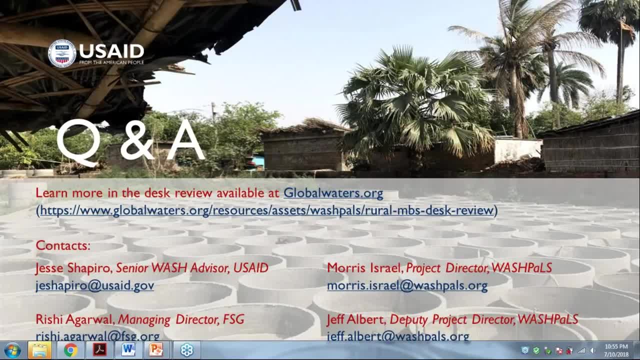 A midline, if you're great To really cutting-edge measurement right now is: oh, we also measure processes rather than just the outputs. What we are saying is: if you really want to bring about systemic change, you need to measure what happens in between. 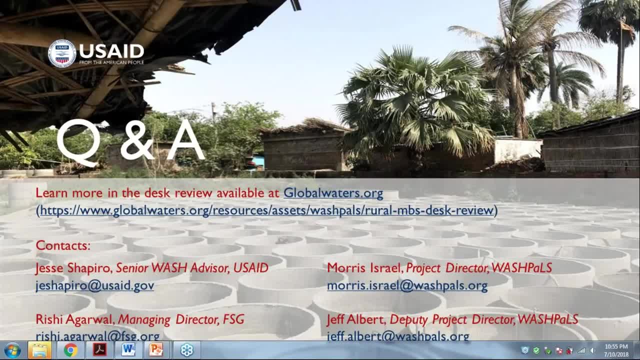 What happens between what your processes are delivering versus what the numbers are delivering? Are you changing something in the system, And that is relationships, power, dynamics and norms. So, if we can measure some of those- and those are difficult to measure and that would require you to do a bit more of sensing rather than surveys- 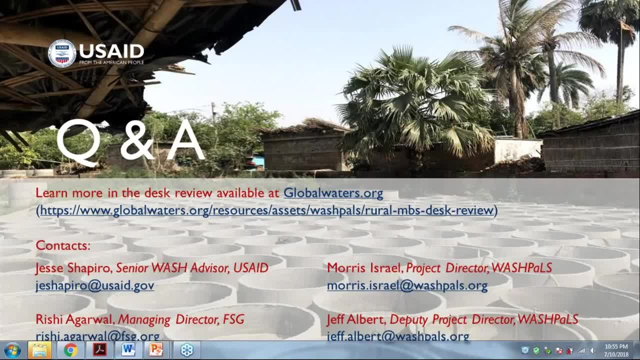 Be comfortable with a bit more ambiguous And if you can measure the parameters, you can actually deliver a lot more value and would allow you to understand where, for example, trust gaps are in an active map in a local environment And where your intervention could actually create a vibrant market for a longer period, beyond the intervention itself. 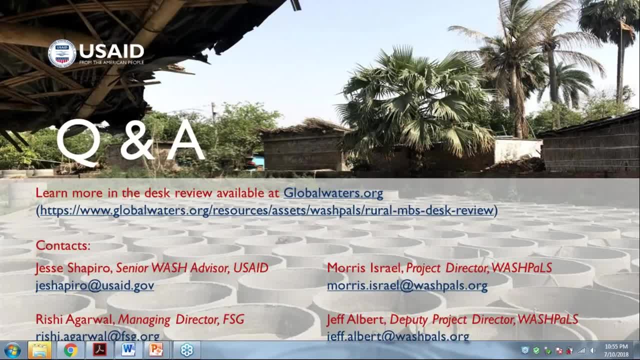 So those are the things we would recommend: to sort of move away from just numbers, to actually start looking at some of these components which drive long-term change, which are the vectors of change. Yeah, So if you're looking at the, But by itself is not enough. 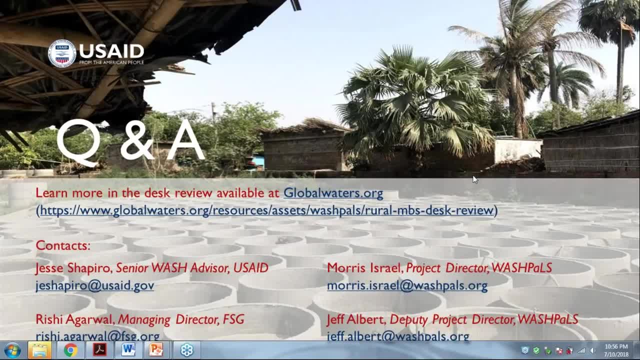 Okay, Thank you, Rishi. Okay, I see we have no additional questions at this point, So let me take a moment here to thank our panelists, Rishi, Subhash, Jeff and Jesse, and the presentations and the thoughtful work they've done. 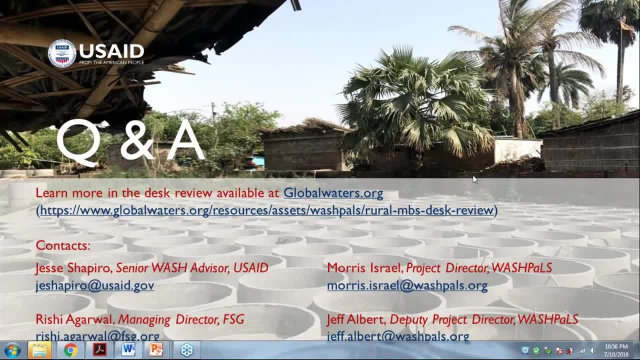 So I would just like to thank. it was a pleasure to meet you and I look forward to seeing you next. And now I would like to thank all those who have participated in this webinar responses to the questions. thanks also to our attendees for those questions, and i'd like to